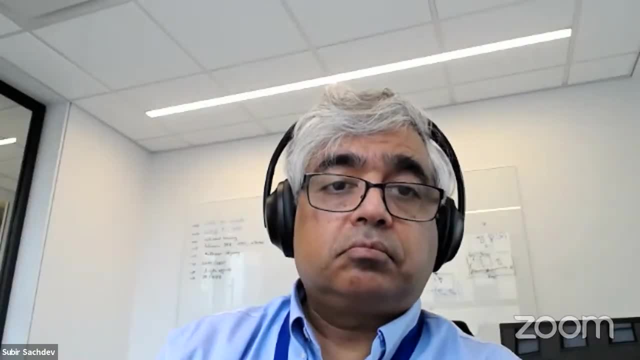 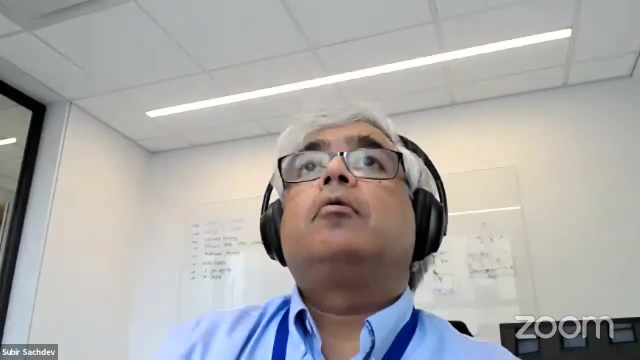 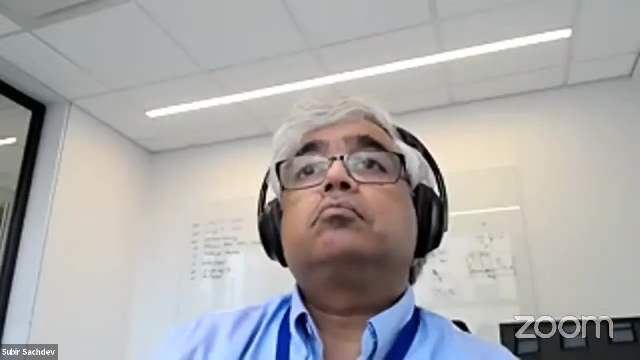 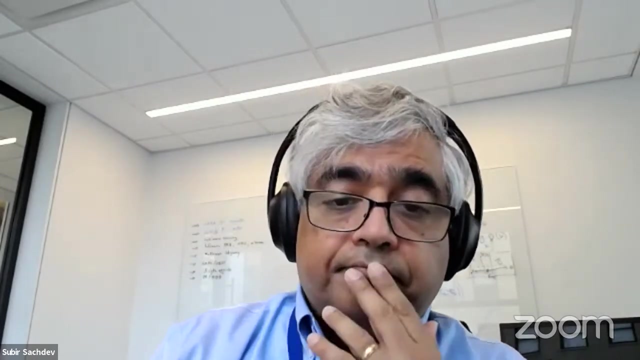 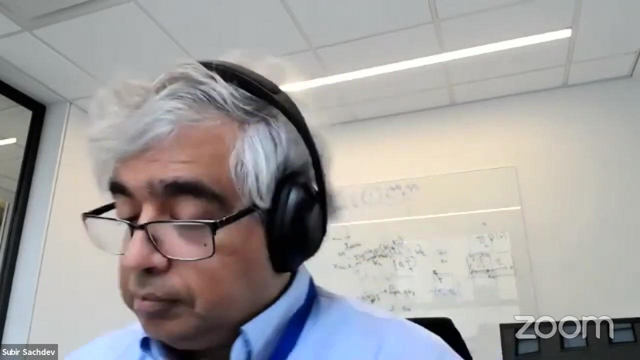 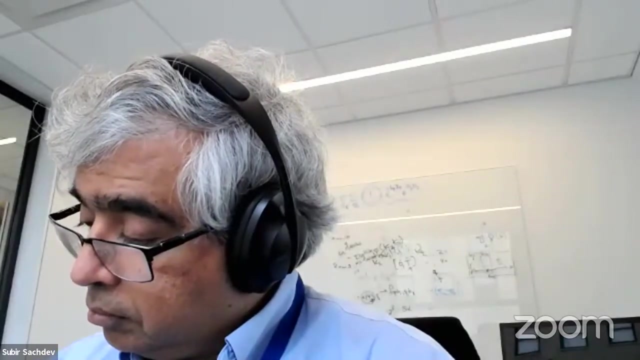 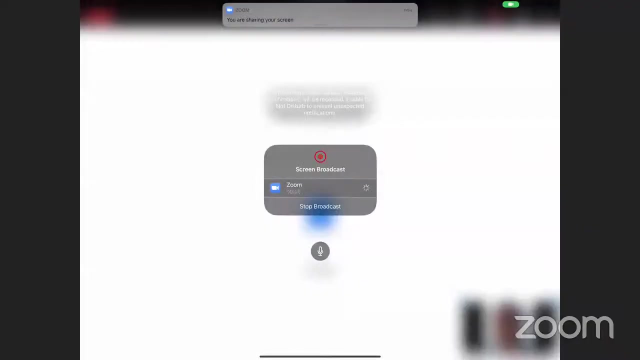 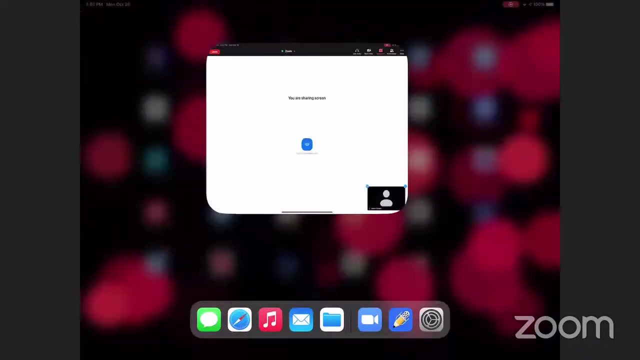 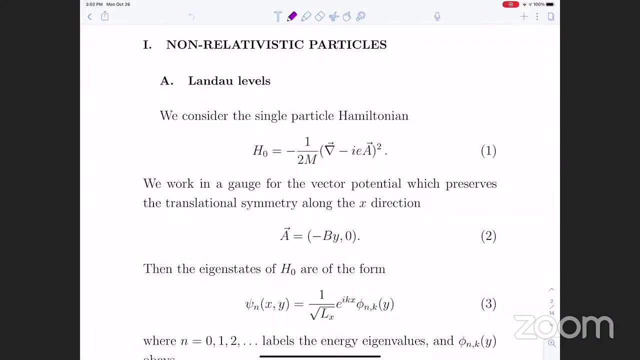 Thank you, Thank you. Okay, so welcome everyone. So we have spent about a week talking about all the beautiful physics in one dimension where bosons and phytonutrients are present And the fermions in the end behave in a very similar way. 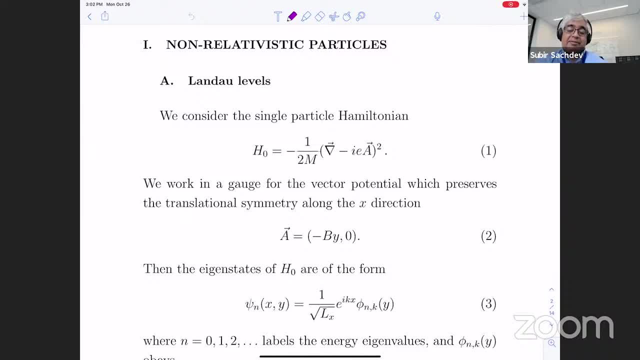 And they give you either this gapless Luttinger liquid state, which is almost a superfluid and not quite a Fermi liquid, Basically all correlation functions that you know of the power law, And there's no discontinuity in the Fermi distribution function on the Fermi surface. 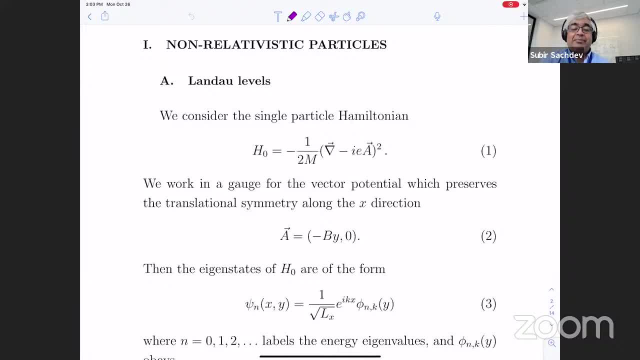 Okay, but nevertheless it has a very simple theory. at the end It's a theory of free bosonic relativistic particles, And from that you can work out many things, including the nature of its phase transitions to gap phases of various types. 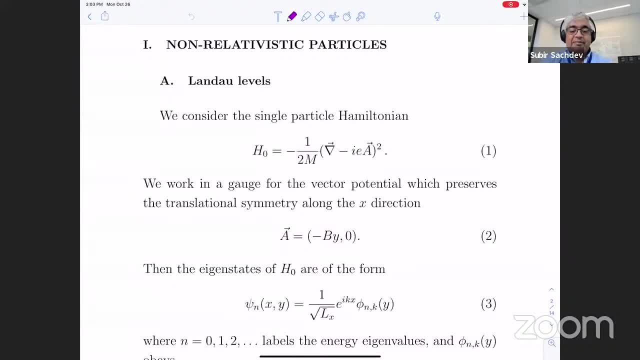 And I think you're going to learn a bit more about those phase transitions tomorrow in a section where how you will cover the part close to the critical point. Okay, so that's the end of that topic. Are there any remaining questions on Luttinger liquid theory? 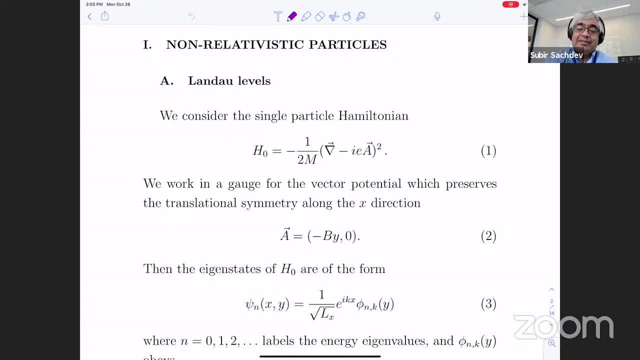 All right. so today we're going to go back to two dimensions and start looking at, in rapid succession, more complicated new phases of matter. We met, of course, the well-known phases: the Fermi liquid, the superfluid, and then the modinsulator and then things like the Willis-Bondt solid. 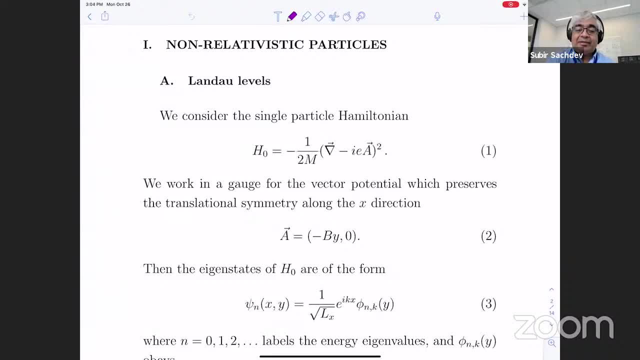 and finally the Z2 spin liquid. Only the last has what we call bulk topological order with anion excitations, And soon we're going to meet new types of states with also anionic excitations and also, in this case, as we'll see today, edge states which are topologically protected. 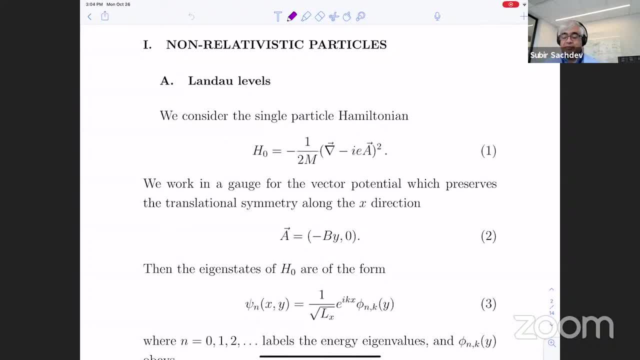 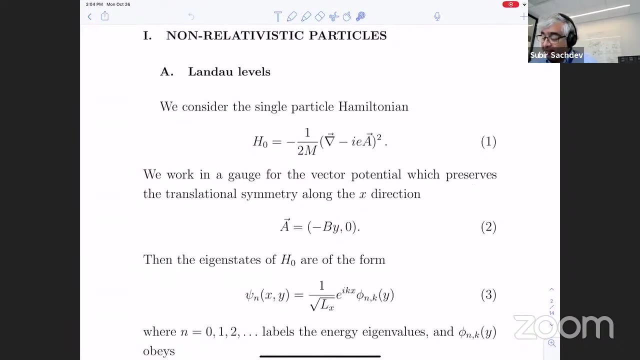 So the simplest case to consider is just particles in the presence of a magnetic field in two spatial dimensions, And so we're going to talk about the integer quantum Hall effect, of course. Okay, so we just take this very simple Hamiltonian: just three particles in the presence of a vector potential. 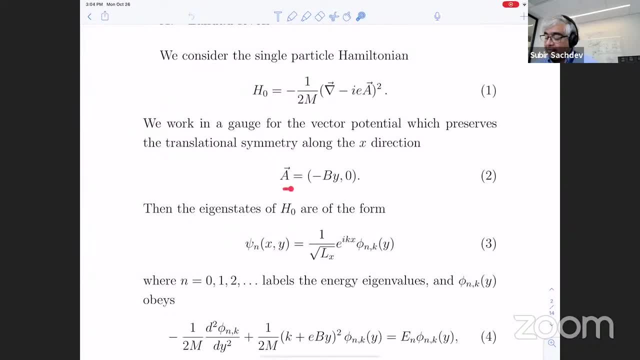 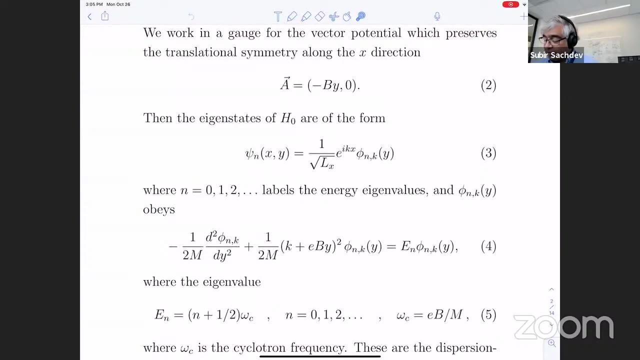 The convenient choice is to take the so-called Landau gauge. where the vector potential is in the y direction, x component increases in the y direction. And then, if you rewrite this out as a Schrodinger equation, as I presume you've seen in maybe your undergraded quantum mechanics course, 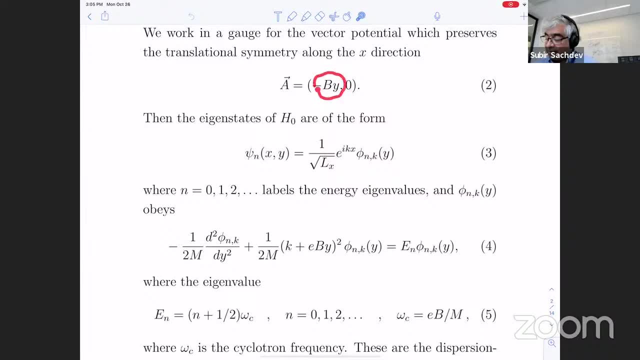 because the vector potential is independent of x. you can guess that the dependence on x will be just a plane wave- It's a vector k And the phase function along the y direction will be, in general, something you have to determine. Anyway, you just insert this, these two onsets- in equation two and three into equation one. 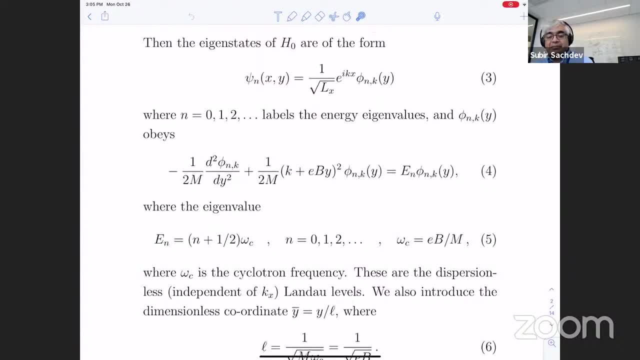 and you get the one-dimensional Schrodinger equation four. So these wave functions phi are labeled by the wave vector k, which determines the dependence along the x direction, And function phi sub n of y, which is a one-dimensional Schrodinger equation. 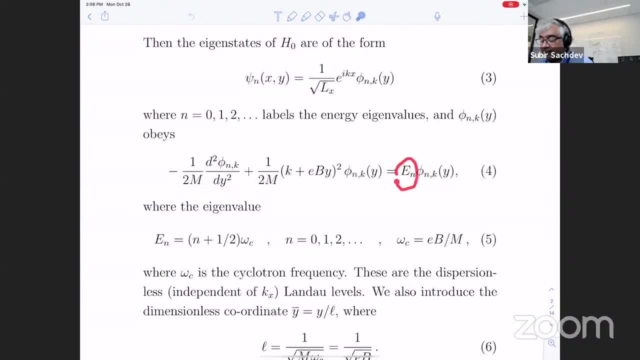 along the y direction. So you have to find the eigenvalues e sub n and the wave eigenfunctions phi sub n for each value of k. So now k, here is just some parameter in the Hamiltonian, And for each k you get a different Hamiltonian in the y direction. 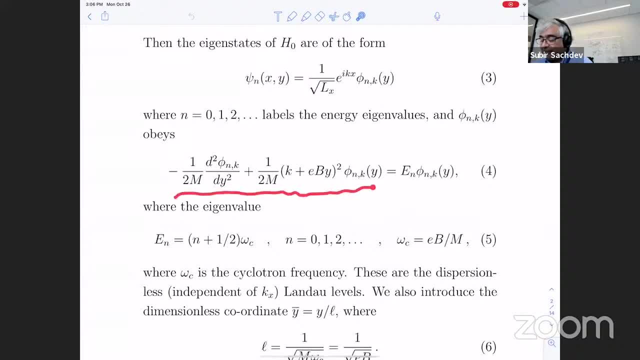 Okay, Remarkably, this is just the Schrodinger equation of a harmonic oscillator, with just one small twist. So you can see that the origin of the oscillator is not at y equals zero, It's at y equals minus k over eb, So it's a shifted harmonic oscillator. 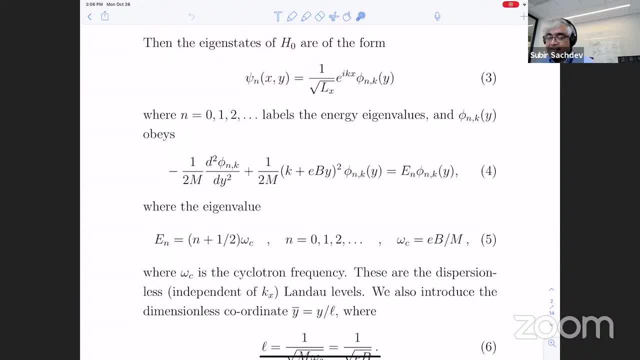 But just shifting the origin of a harmonic oscillator doesn't change the energy. And so you conclude that actually the energy doesn't depend on k, which I kind of anticipated here. All of the wave functions will depend on k, All right. 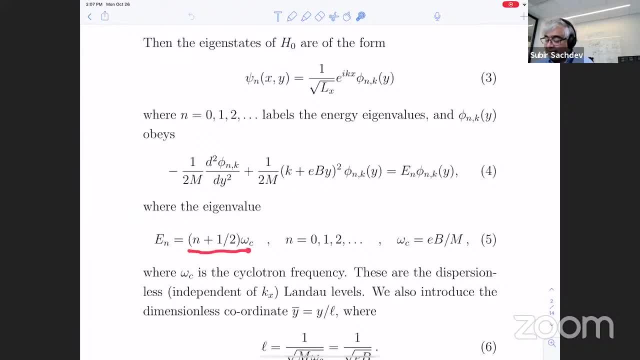 So then the energy eigenvalues are the harmonic functions and those are the harmonic oscillator eigenvalues. And you just look up the spring constant here, and that turns out to be what's called the frequency, is the cyclotron frequency, omega c, which is the charge of the particle. 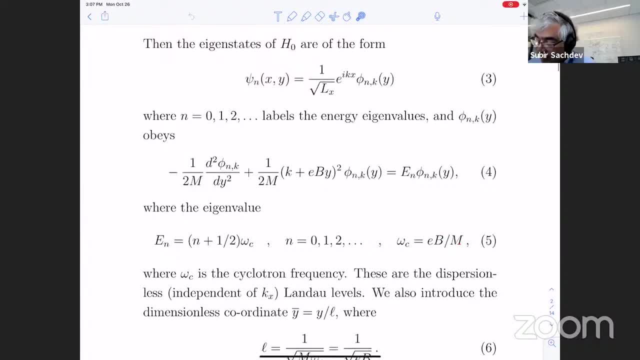 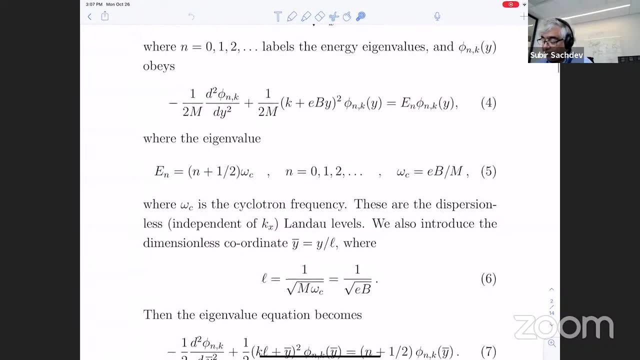 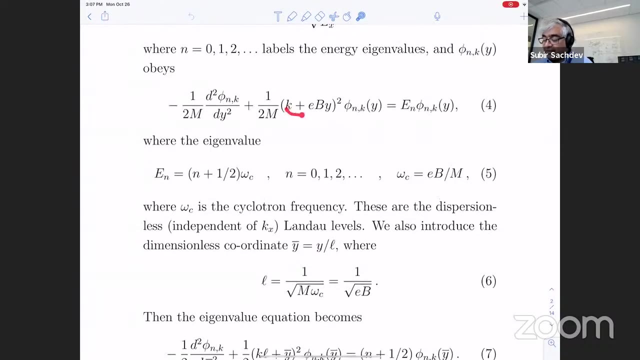 the magnetic field B divided by the mass of the particle, capital M. I'm using capital M because little m will soon represent something else. Okay, So another important quantity here which you can already see over here in units where h bar is 1 here: 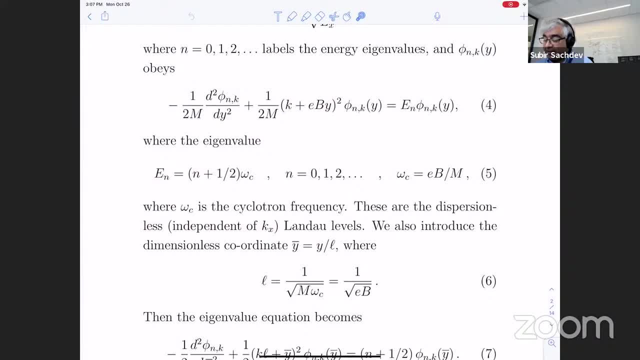 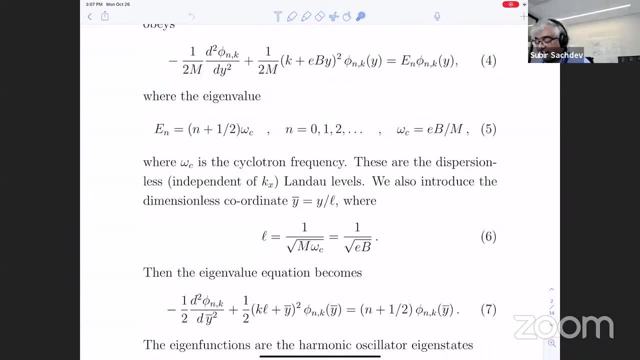 is the magnetic length. So the magnetic length, roughly speaking, is the width of the harmonic oscillator which, as you know, is square root of h, bar over m, omega c, And that's square root of e times B. So this is a fundamental length that you can obtain from the magnetic field. 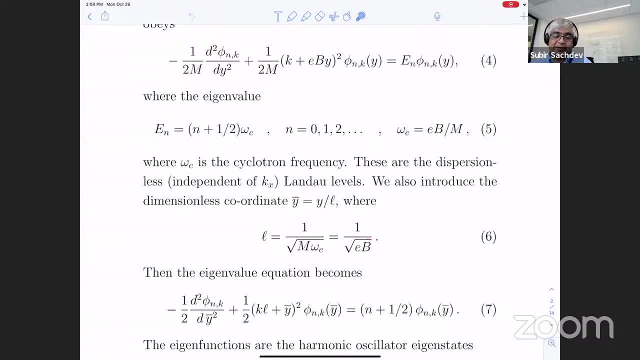 and the charge of the electron. And an appropriate fact is that appropriate factors of h bar that are not here. So anytime you have a system in the presence of a magnetic field, you can characterize the influence of the magnetic field by this length scale L. 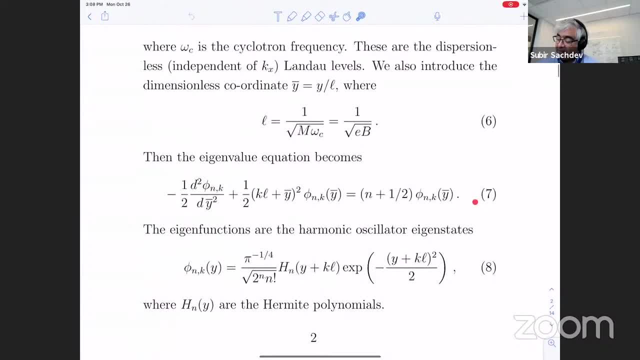 Okay, In terms of the magnetic length, you get this dimensionless equation. and then the eigenfunctions are the familiar Hermite, polynomial, stem, Gaussian. Everything's just been shifted and that's all the shift does. The key value of k does is shift the origin of these things. 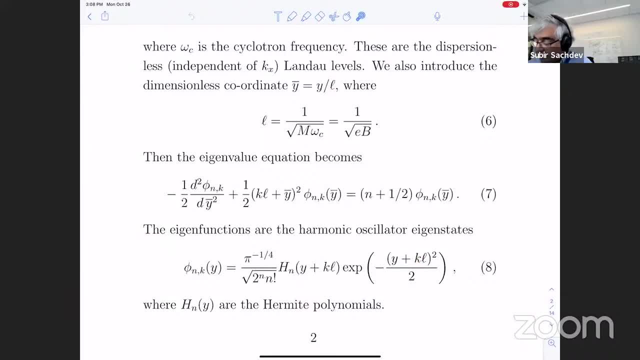 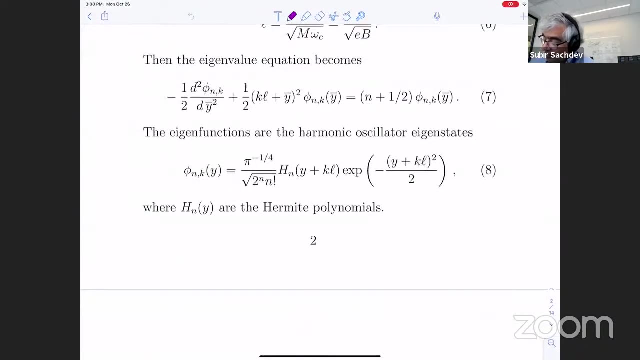 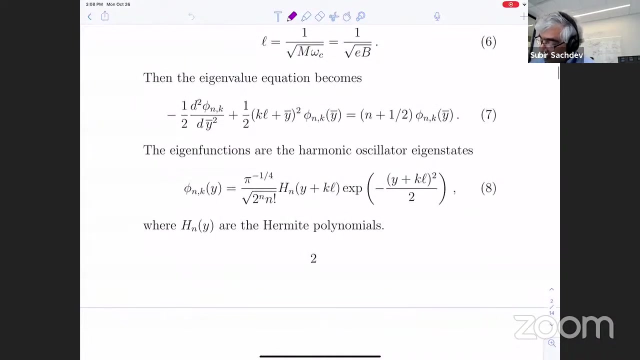 but doesn't change the energy. Okay, So you've got a set of hugely degenerate levels here. You know you have these levels. that are all you know. something like this: If you pick a value of k, then there's a y. 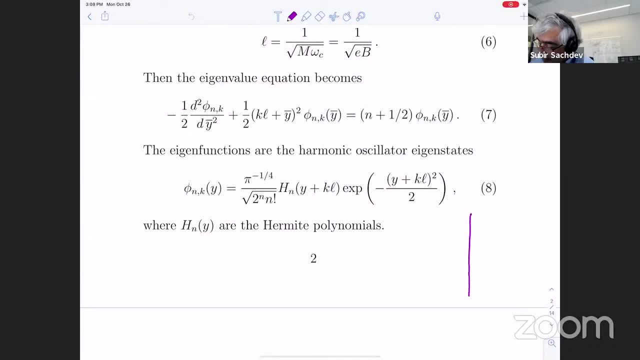 equals minus kl, where they're centered. So this, this is a. you know, this is the y direction and this is the x direction. Then the wave function is just some Gaussian which is moving in this direction with the wave vector k. 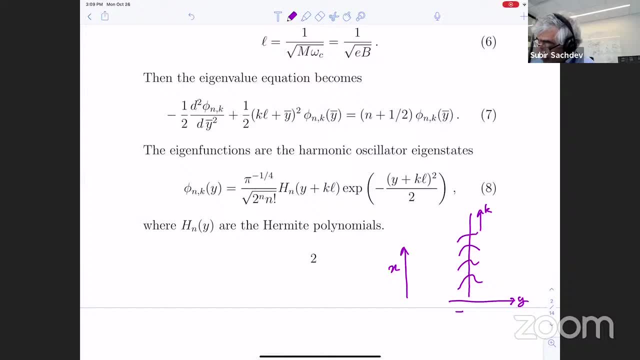 and this location is minus kl. Okay, So as you change the value of k, as you change how fast the particle is moving, you change the origin of coordinates. So you can sort of see that I may get the sign wrong. maybe on the left it's moving up. 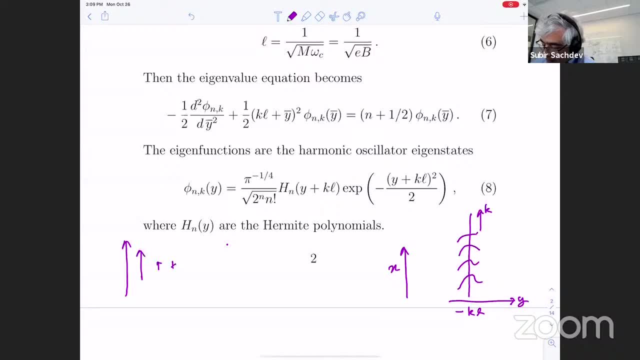 and then it's moving slower and slower, and then this side will be moving this way. So this will be: y equals zero, and the length of the arrow represents the magnitude of the strength of k. Okay, So that's a particular gauge. 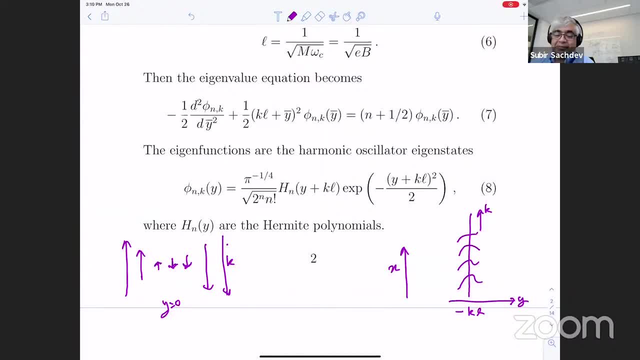 I mean you can see the kind of cyclic nature of the motion, but in this Landau gauge they're just moving in linear directions and they're all degenerate, have the same energy even though the value of k is different. 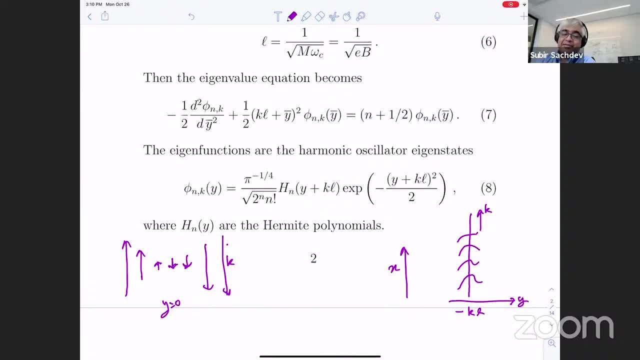 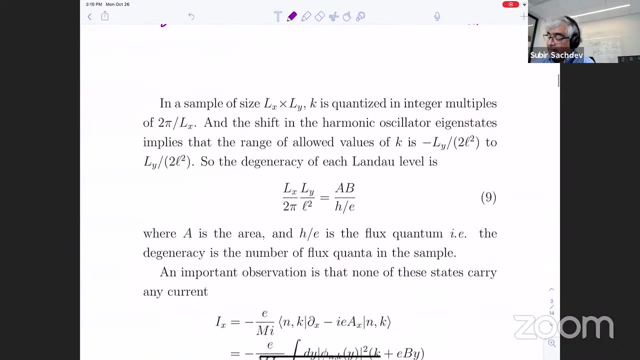 and you can take different linear combinations and in fact rotate them by 90 degrees. and nothing special about y. There are corresponding states along the x direction too. just by taking linear combinations of these states. Okay, So these are the states of the Landau level. 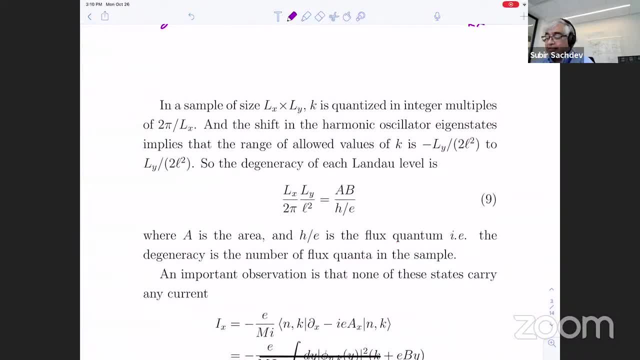 So now how many states are there? So anytime you count states you have to count, make the system finite. So make the system Lx times Ly. So if you have a system here, this is Lx, this is Ly. then the values of k. 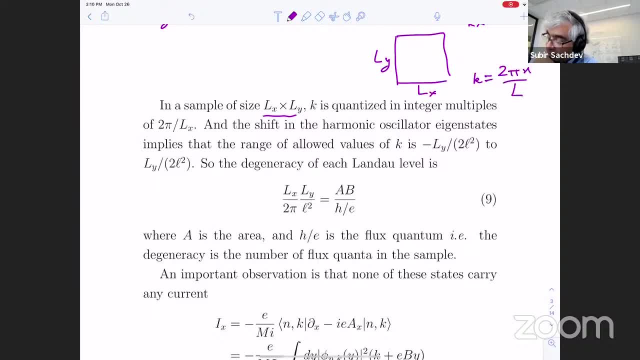 are integer multiples of Lx, So they're discrete. Now, each value of k determined the value of y, where the wave function was centered. So for each of these k, you have these orbitals in this direction. And what's the spacing between them? 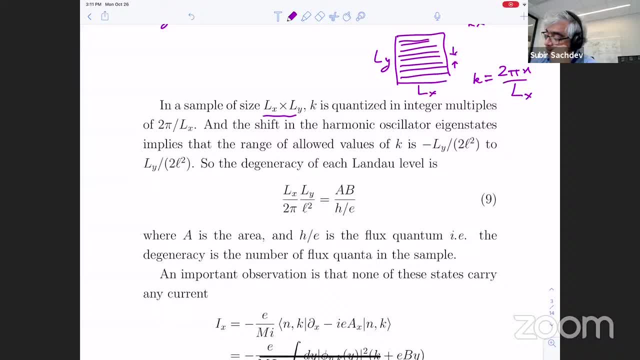 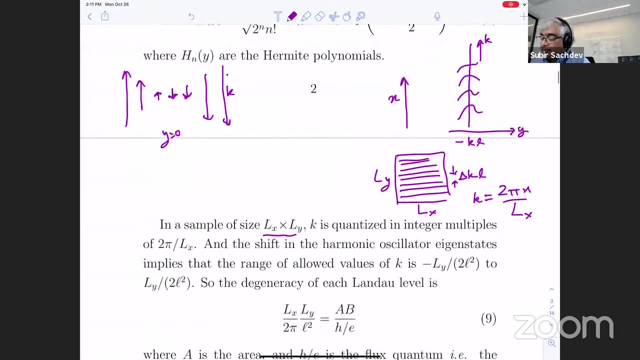 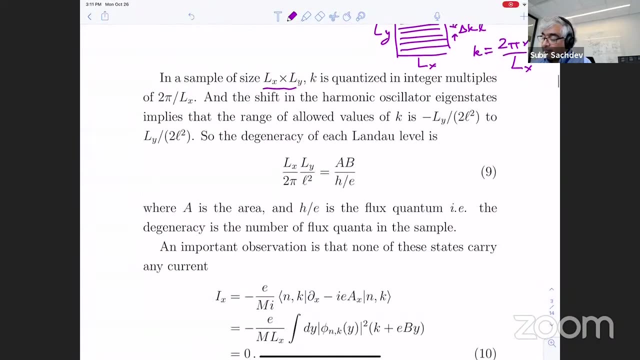 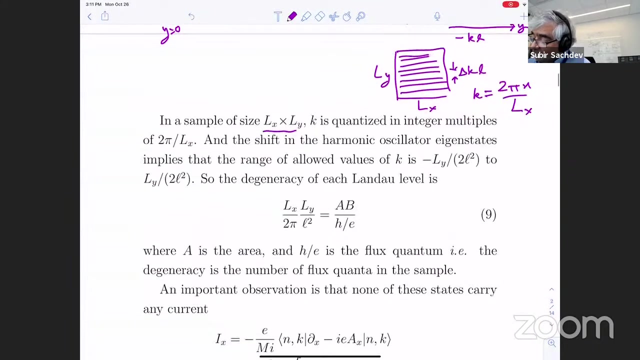 The spacing between them in the y direction is basically delta k, the change in k between two successive values times L, the magnetic length That comes from this L over here. Okay, So all right. So imagine that Ly- so you went from minus Ly over two- is less than y. 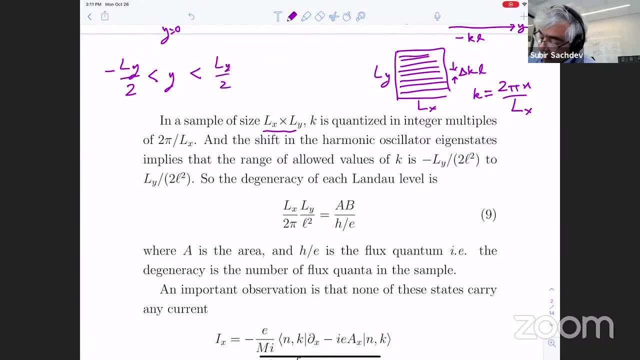 into Ly over two. But y is equal to k times L. So that tells me that what is going on here? The range of allowed values k minus y, get an L squared there. Oh sorry, There must be a mistake here. 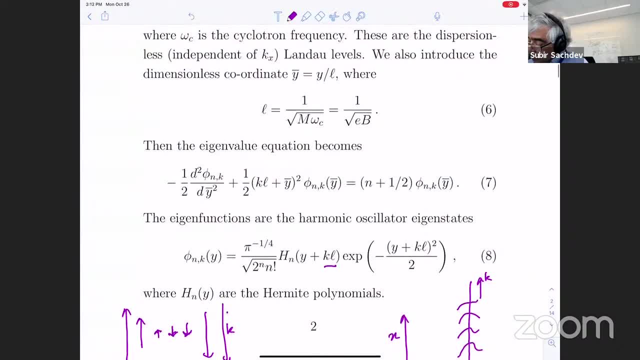 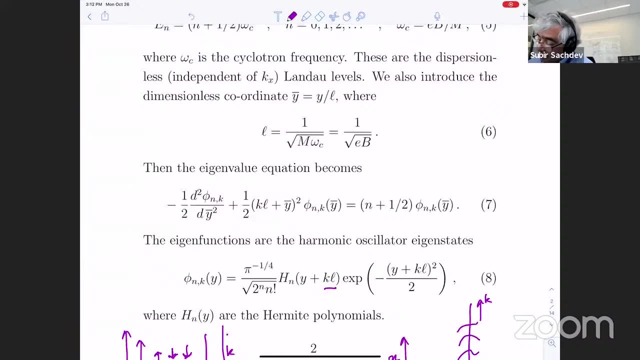 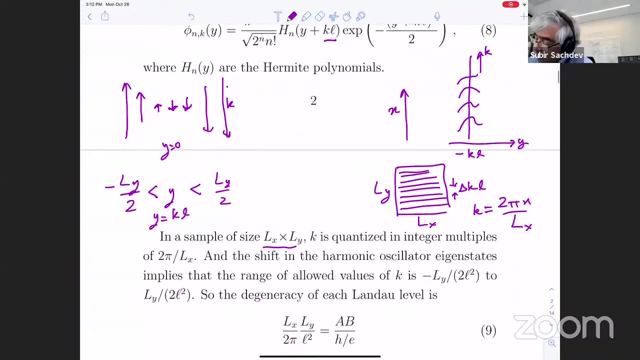 This doesn't make sense. Yeah, To get this. So this is dimensionless. So this y coordinate is y bar. Yeah, Okay, So y goes as k L squared. If you take the actual y coordinate, it's k L squared. 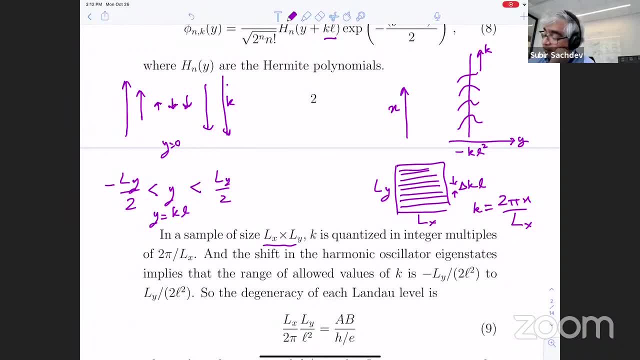 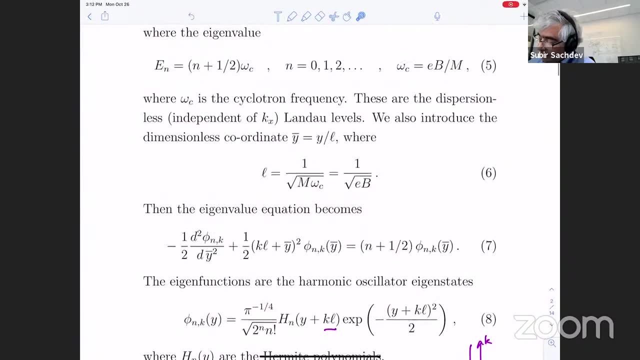 Because y has dimensions of length, k has dimensions of inverse length, So there must be a L squared. Yeah, So you know. this equation is y bar. The shift in y bar is k L. The shift in y is k L squared. 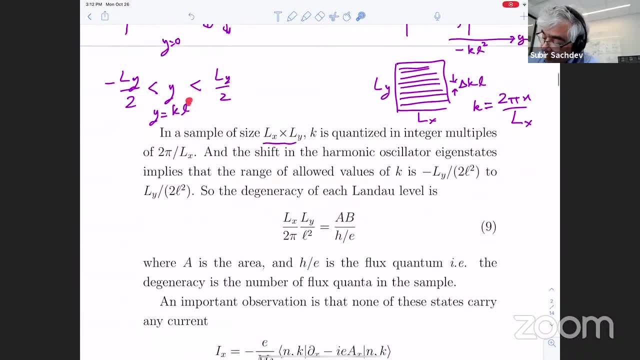 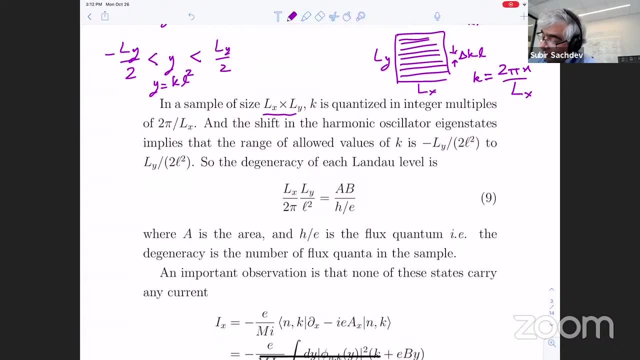 Okay, So this goes from k L squared. Oops, So that tells you that the range of values of k from this equation are between these two values. Now each step, each step of k is, has distance two pi over L x. So the total number of steps 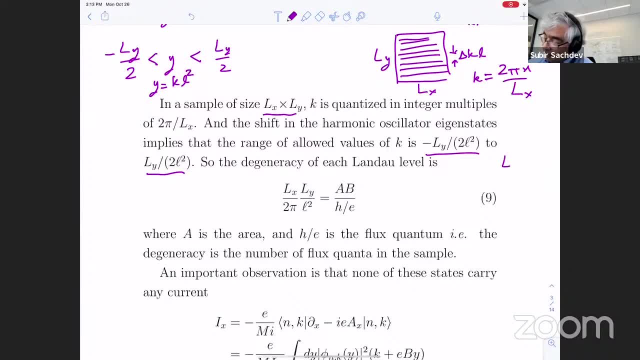 or the total number of states, is the distance you have to go, which is L y over L squared divided by the size of the step, which is two pi over L x, And that's equal to this And that turns out very beautifully. 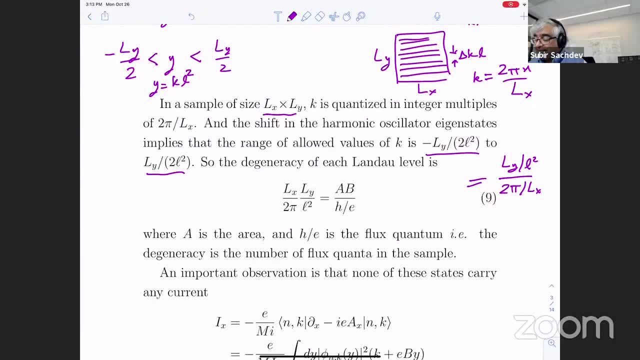 L x and L y appear in the same way as they should. Otherwise something's wrong. That choice of y versus x is just a gate choice, And that's so. when you put it in physical units in the numerator you have a times b. 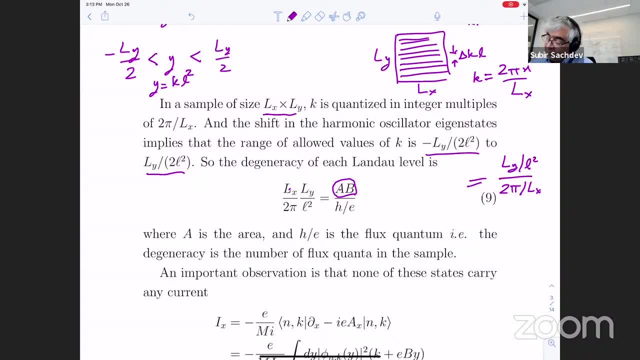 the area of the sample times, the magnetic field, which is called the total flux. And you divide the total flux by the quantum of flux, which is h over e, So that's just an integer. So that tells you how many flux quanta. 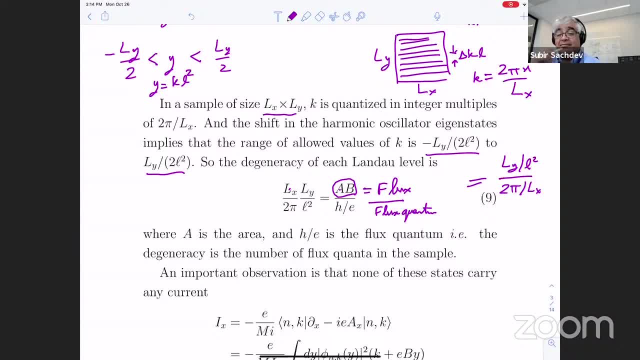 do you have in your sample Here? of course, we have met this quantum of flux before. It was h over 2e previously, when we talked about superconductivity. But here the flux quantum would be h over e because it's just single electrons. 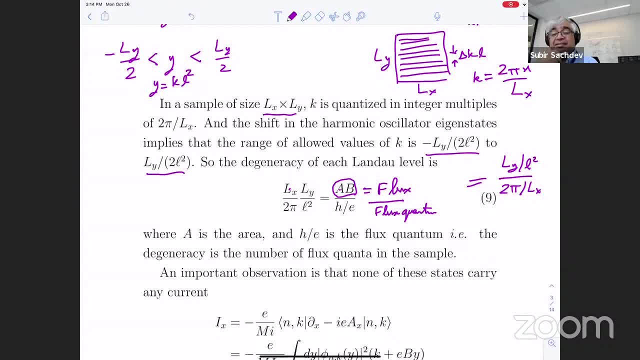 And also previously we had an hc over e. The c appears in CGS units. In MKS units there's no c. Okay, so we have then our spectrum as a function of energy. So you have some energy here, energy, and there's just a bunch of levels. 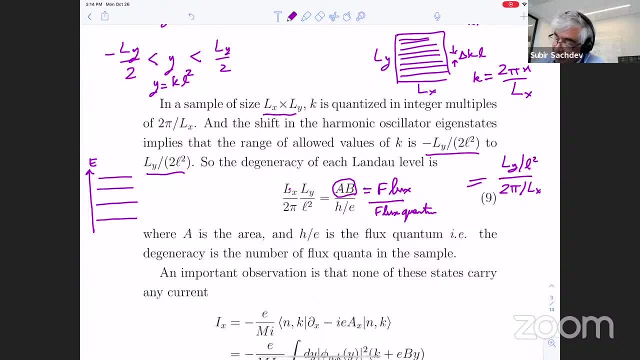 This is called the Landau level, And the spacing between these levels is h, power, omega, c, And this is called the n equals 0 level, just like a harmonic oscillator: n equals 1 Landau level, and so on. And the big difference, 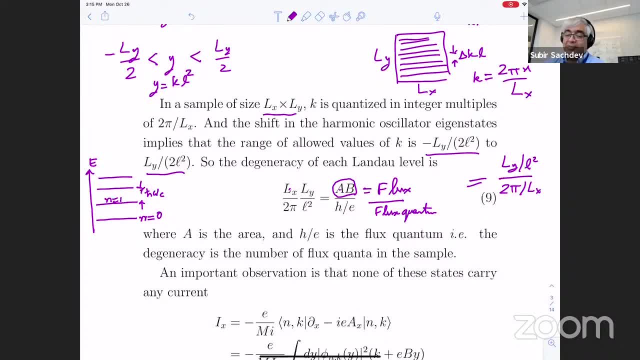 in the harmonic oscillator is that each one of these is not just one level. It's a huge number of levels. The number of states in any one of these energies is given by. here It's the total flux in the sample. The area is a huge number. 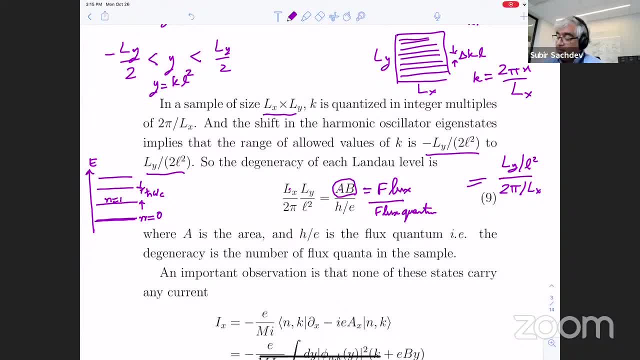 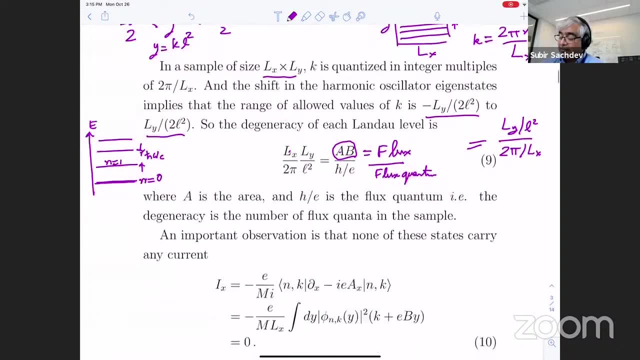 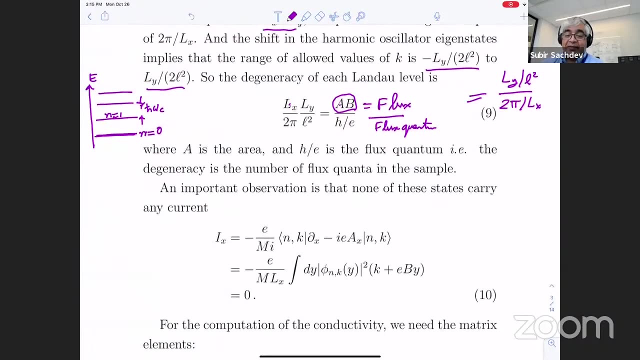 Divided by the flux quantum. Okay, All right. So those are the eigenstates of a particle in two dimensions moving in a magnetic field. So all of these states, in fact, don't carry any current. You might think they could carry current. 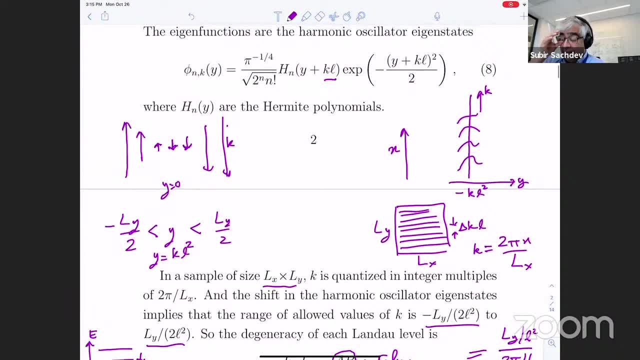 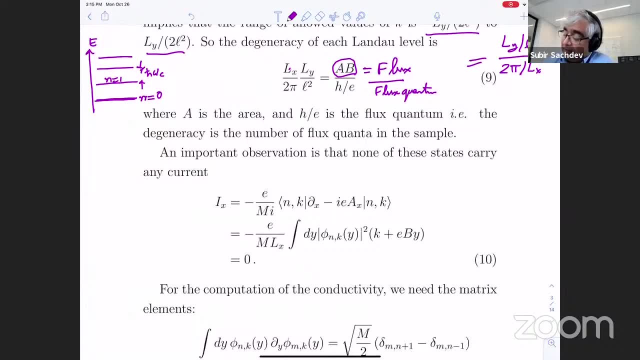 from the arrows I was drawing to represent the value of k, But in fact they don't, And so the gauge invariant current is of course the matrix element of the gauge invariant gradient: grad x minus ikx. But this combination, when it acts on the e to the ikx here, 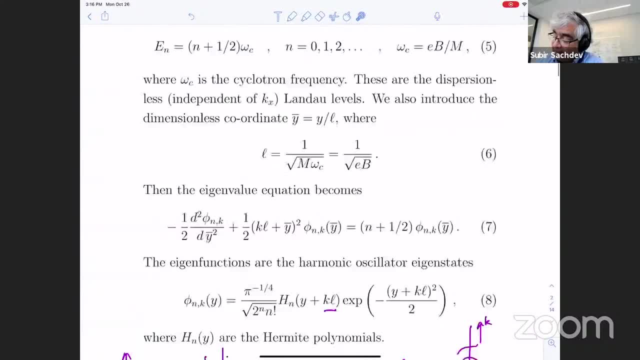 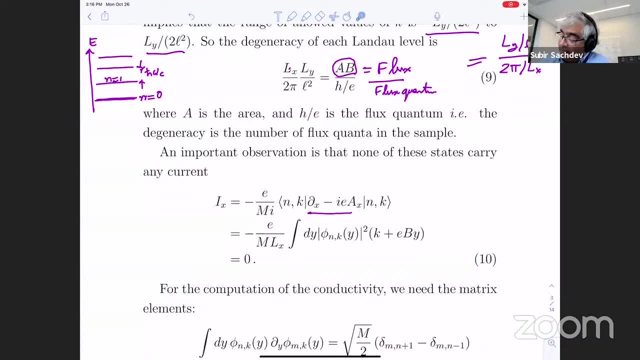 this e to the ikx turns the gradient into k And Ax was By And this is the wave function in the y direction. This is k plus By. But this is exactly. this is the shift at coordinate of y, exactly that appears. 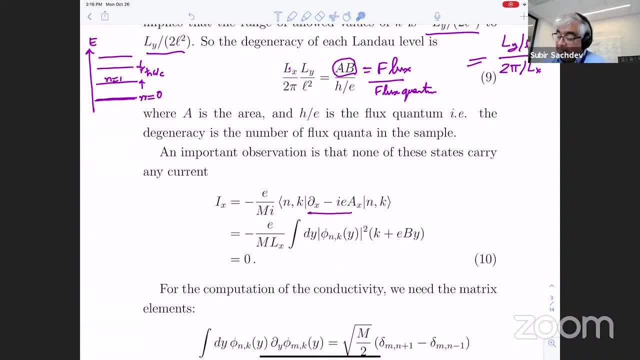 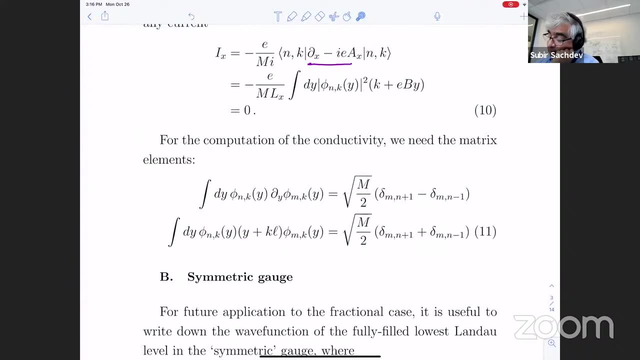 in the Hamiltonian. So it's zero. So in fact these are all. these are all states that are not carrying any current. Later on for a computation. we'll do, we can. you'll also need these matrix elements. I just wrote them down here. 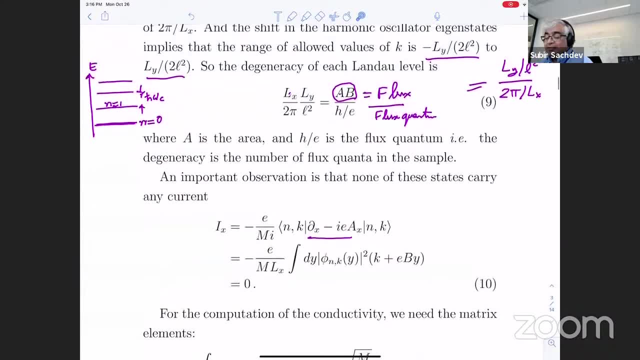 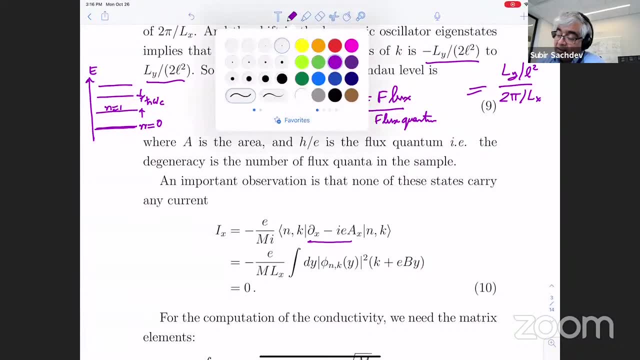 Okay, So that's, that's what will happen in a moment. And those are the states. And now you know, of course, if you're dealing with a many-body system, if you've got a bunch of free electrons that are going to occupy. 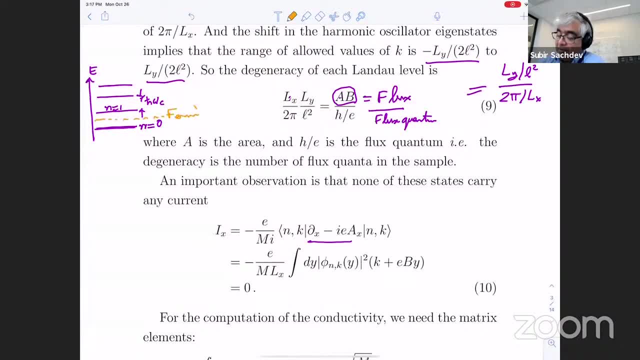 these states. you know there'll be some Fermi level- This is the Fermi energy- And this will be the situation where the zeroth Landau level, the first Landau level, is fully filled, whereas the others are not. I guess it's called. 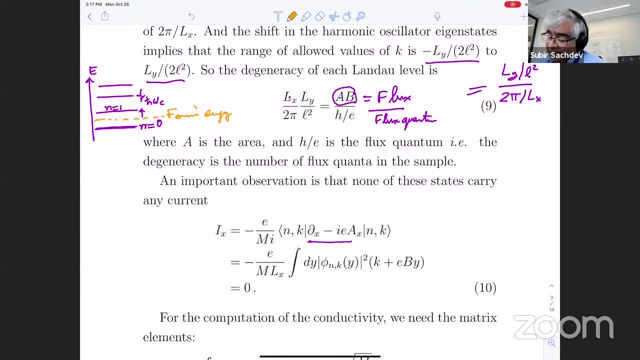 the n equals one Landau level. usually, Yeah, Not n equals zero. So you know, that's that's. that's. that's a very good example. Okay, so that's the result in the next slide. That's the result. 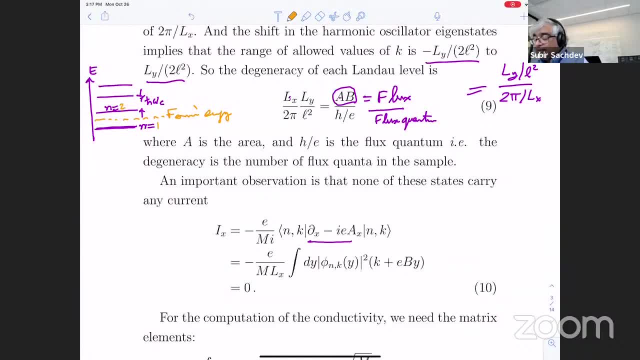 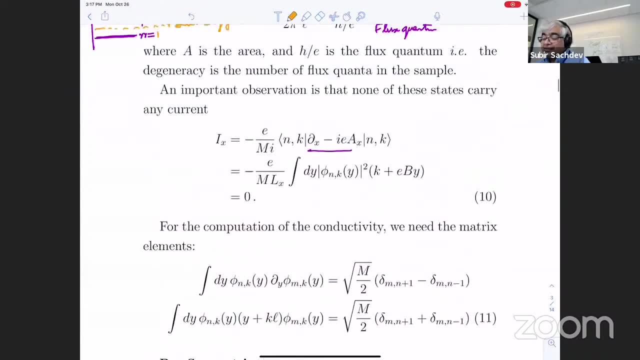 in the next slide. In graphene we have an n equals zero Landau level. Okay, Just as a quick aside, you can also try to work things out in a different gauge. And another gauge is to take: a is equal to 1 half r cross B. 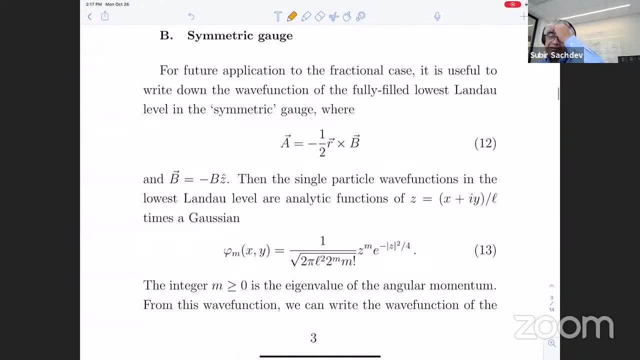 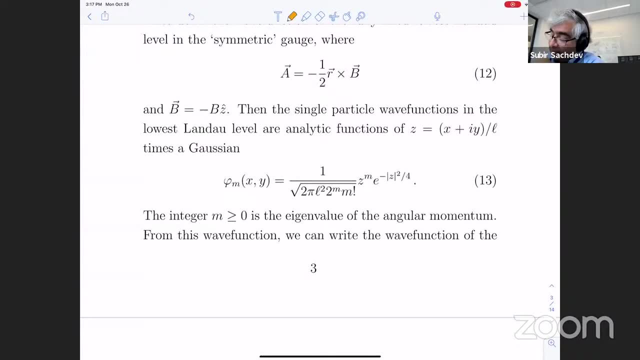 This turns out to be very crucial in the fractional quantum Hall effect. In this case, the wave functions are approaching a state that's going to be have this beautiful form: they are a function of z, which is x plus i, y, divided by the magnetic length. 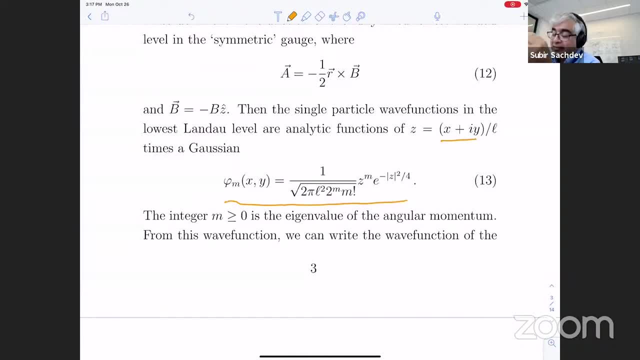 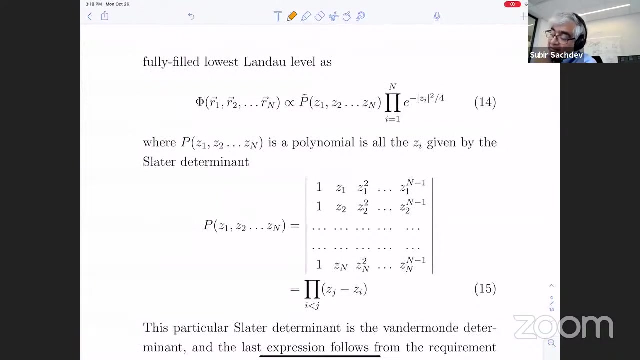 uh, so they're like circular orbits rather than straight orbits, and m is the angular momentum. okay, so they're just going around in circles executing cyclotron motion. um, okay now, another beautiful thing about this function is that it's useful to write out the many body fully filled lowest landau level. so if you just take, if you're going to fill all the states in, 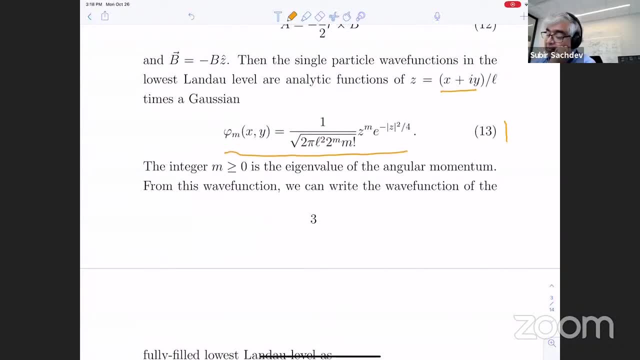 the lowest landau level. you're going to take states from: m equals one equals m equals zero, m equals one. they all have the same energy, all the way up to m equals n minus one. uh, m equals zero is the is the gaussian wave packet at the origin. m equals one is. 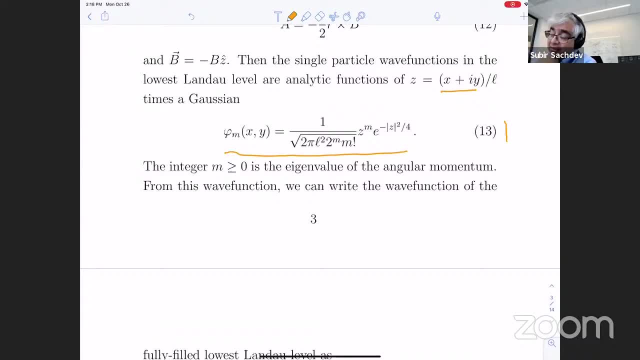 the you know another state which is all of these states are linear combination of the other states in the landau gauge, of course. so if you take the first m levels to get a droplet, so there's a wave function of a droplet. now, because as you increase m the wave functions go farther and out from the. 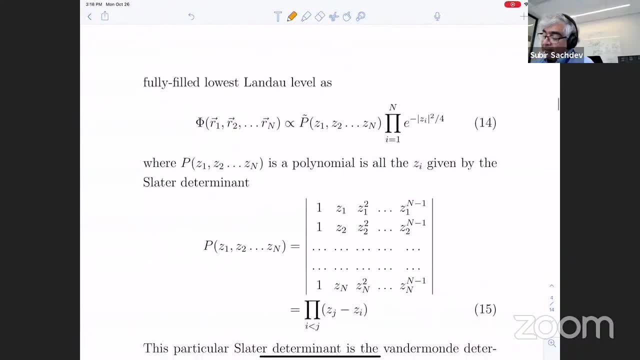 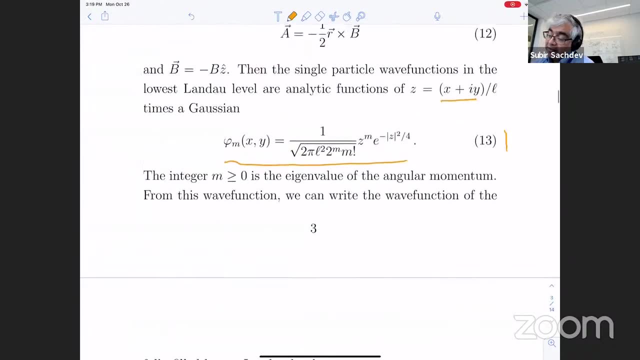 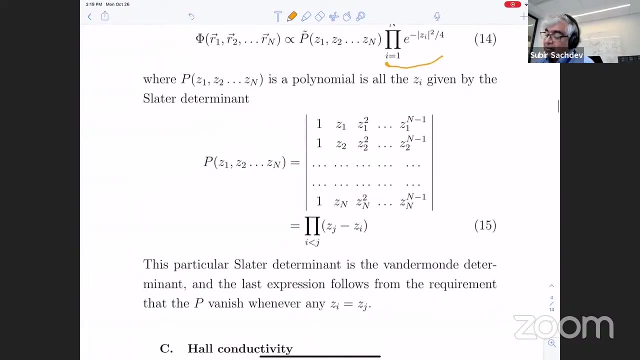 origin, uh. then the wave function will of course have these uh gaussian factors that are not terribly important, but the pre-factor, the gaussian, is now an analytic function, z, which is a function of x plus i, y, uh, and in this case, the states that you're occupying are, you know, one z to the one z. 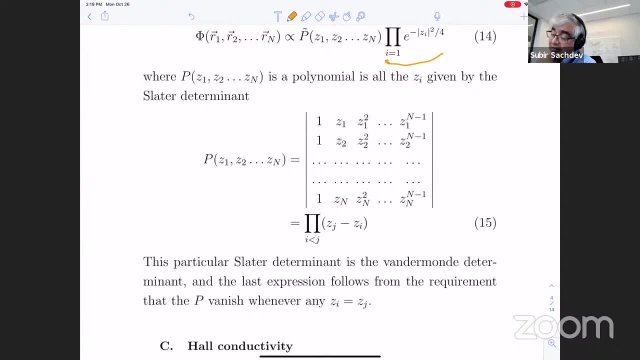 squared c, cubed all the way up to z, to the n minus one, but you have n particles. you have to take the coordinates of the different particles and then work out the determinant. and this particular determinant is something that's known. it's something called a vanderbond determinant. 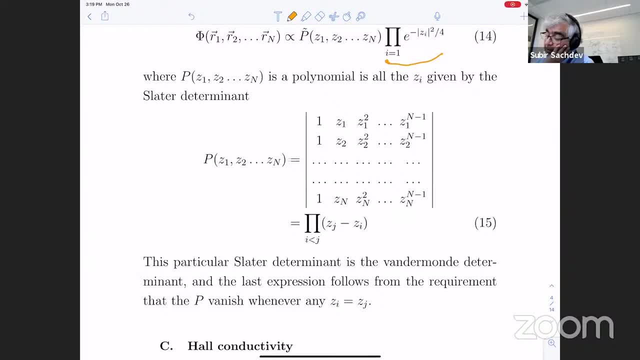 it's just anti-symmetry in the wave function of all the particles. it's exactly equal to this expression and you can prove that quite easily by verifying that, like any determinant. if the, if the two, any two, if z1 equals z2, it must vanish. 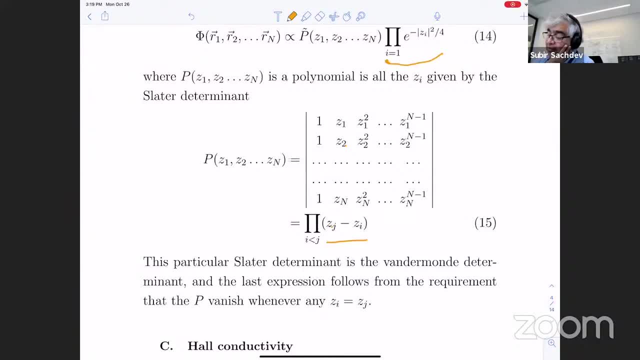 and so they have to be these factors of zj minus zi, because this, by construction, is in the polynomial, and then you can see that the degree of the polynomial that you estimate from the determinant is exactly the degree of this one. so there's nothing else. this is. 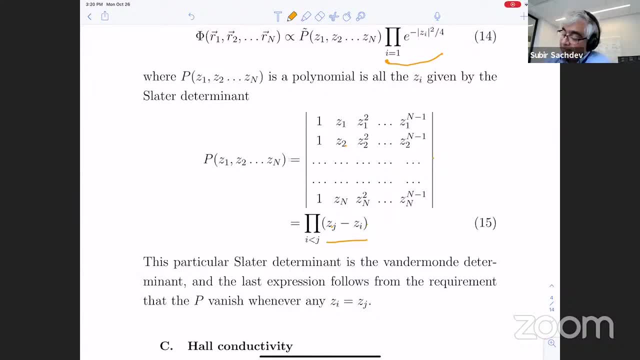 a complete answer. the only thing that remains to verify that the pre-factor is one, and that's that's easy to do, okay, so so the whole full wave function in the uh, in in the ground state, when the fully filled and our level z1 through zn is product on r less than j, zj minus zi. 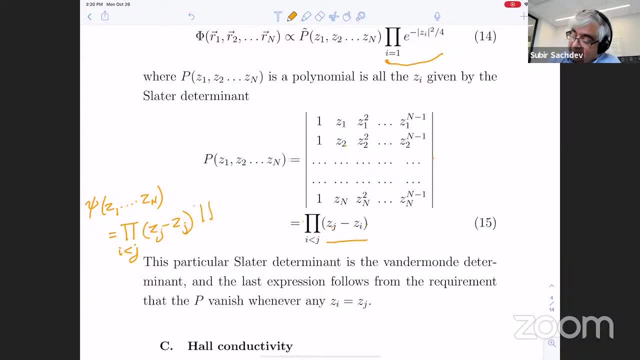 times product on i e to the minus z, i squared over four. so that's just three particles in the lowest land level and of course, as i'm sure, if you already anticipated, the reason i'm writing it out is when we include interactions and get the much more interesting many particles. 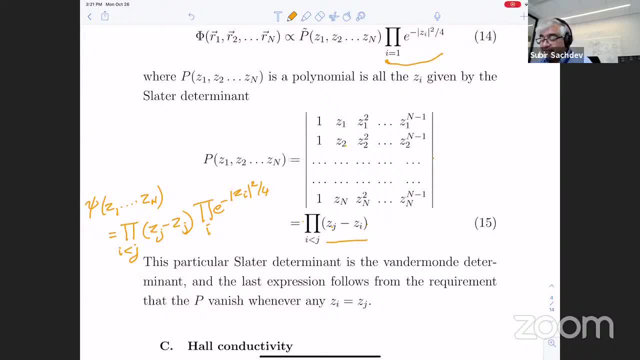 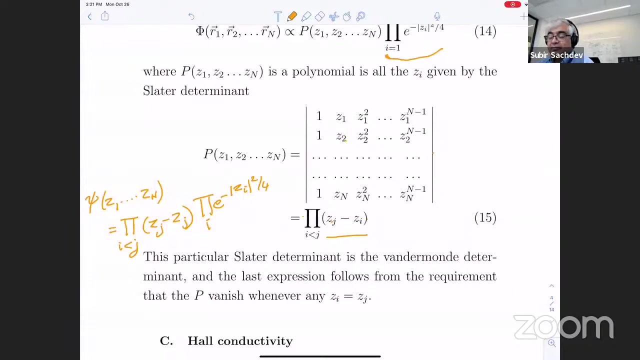 laughlin states, it's a very simple modification of this particular wave function. all right, so question. so far all right. so now let's do something a little bit non-trivial. uh, let's compute the conductivity. we have a fully filled land level. let's say the lowest land level is fully filled. 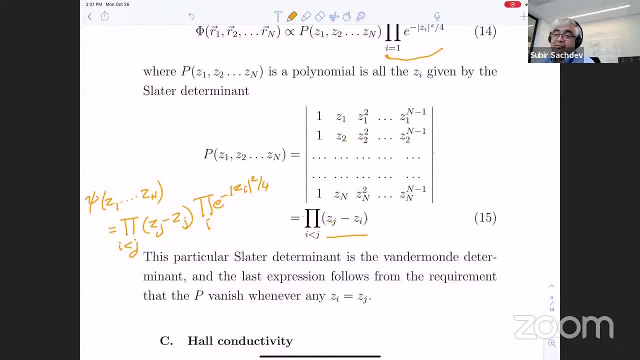 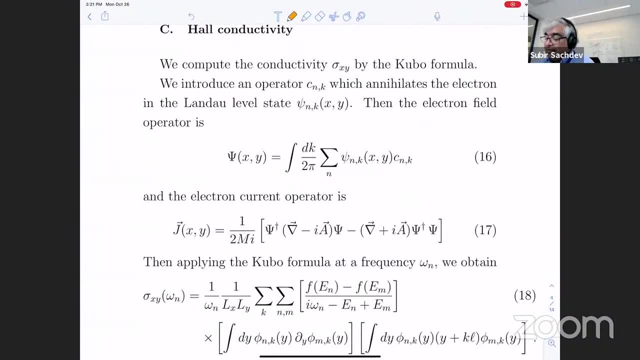 and we're going to apply an electric field and measure the current. okay, so this is the current operator in the presence of a vector potential. so what we want to compute is the. we're going to apply an electric field in some general direction and we're going to compute the expectation value of j. 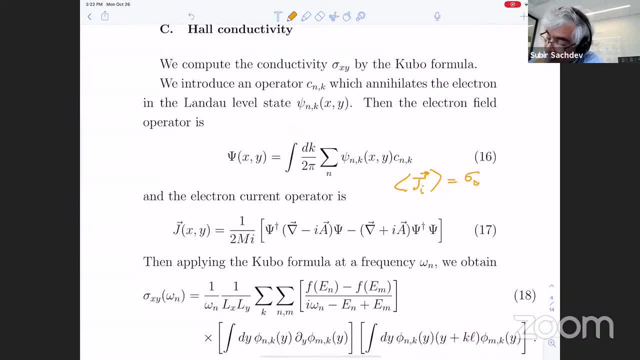 is sigma x, y sigma i is sigma i, j times the electric field applied in this j direction. okay, so you're going to change the hamiltonian to include a small electric field and you're going to do linear response theory. so this is worked out by the cuba formula. 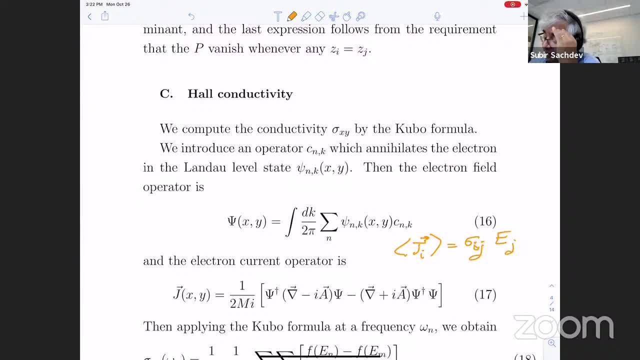 which i think has been well. we haven't really discussed it in this course, but it ends up being just, you know, you have a current vertex here for the current that you're computing, just computing this bubble diagram or the kinds of which you have seen before, and okay, um. 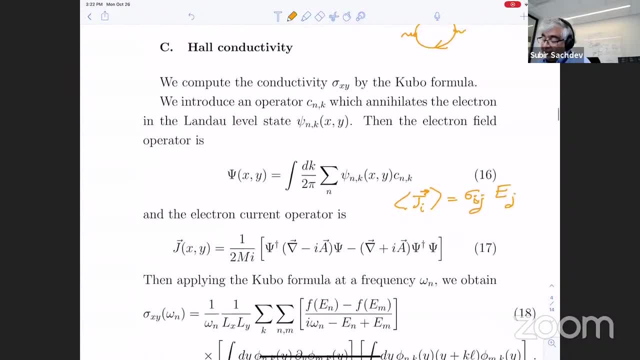 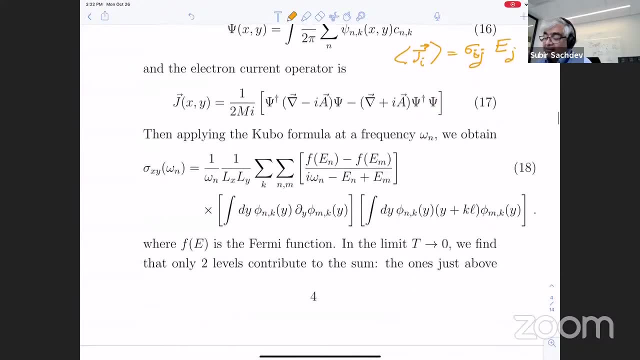 if you haven't seen this, okay, well, there's no big deal. uh, we're going to derive the final result many different ways, you know shortly anyway. so, if you evaluate this graph for these particular eigenstates, uh, this is, this is what you get. these are these matrix elements that i've 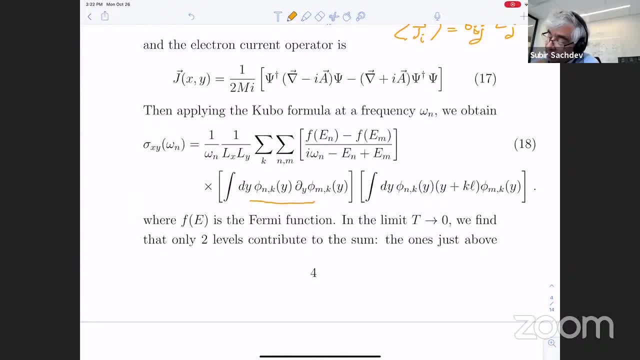 written down earlier before matrix elements of that cup. here, when you put the current operator- and these are the usual fermi distribution function, which says that, uh, you know, you have to make transitions from occupied states to unoccupied states. okay, all right. so now you evaluate this. now we know everything here. we know all the en, we know all. 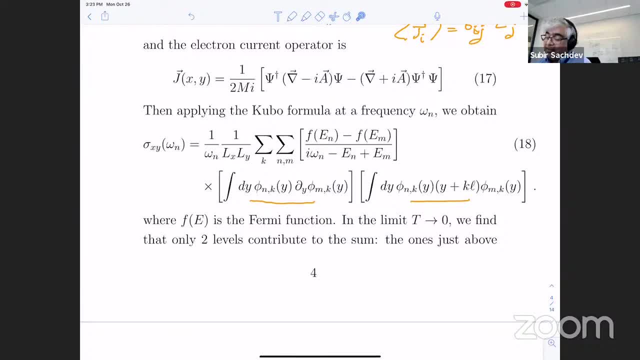 the phi and just evaluate this at zero temperature. it only the answer only depends on where you put the fermi level. so we'll just put the fermi level somewhere between two of these degenerate energy levels, which are called landau levels. i should have said so if you just pick the energy level. 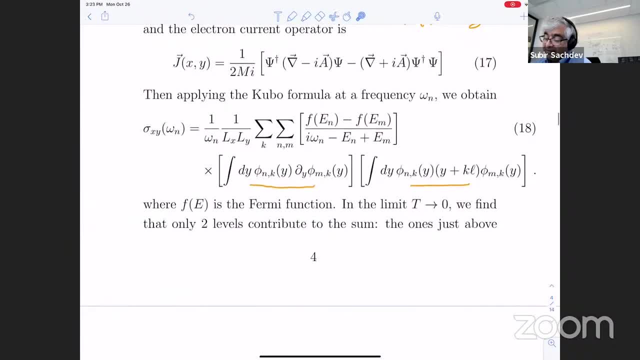 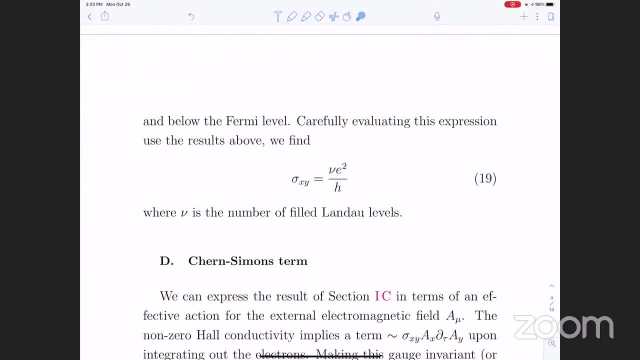 somewhere between these landau levels and you put the fermi level somewhere between these landau levels and just evaluate this mass uh and amazingly you find the following answer: all things drop out and your hall conductivity is the number of philando levels times. you know. e squared over h. 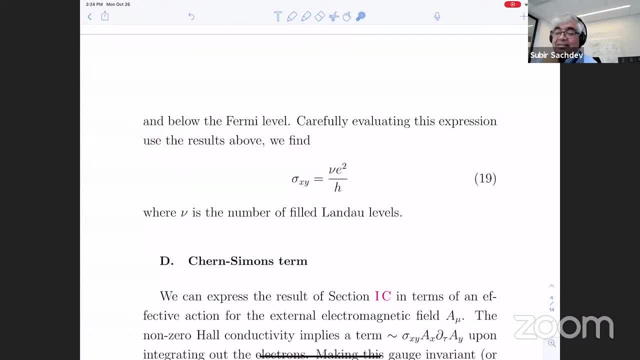 where is the electron charge and h is planks constant? and it's. this is when you know the whole conduct is well defined. where you're going to put the fermi level is right between two landau levels, so you have a gap to all excitations and in this case you find that the hall conductivity, when you 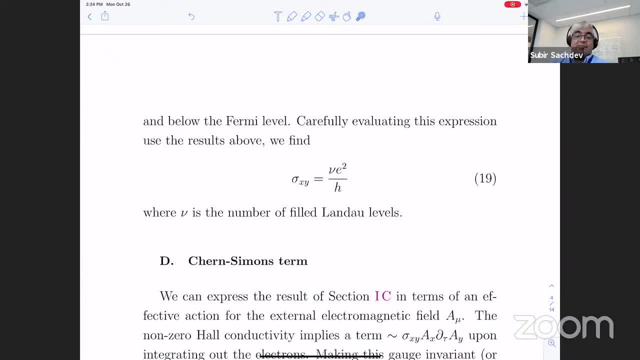 do this calculation carefully. uh turns out to be this number. so this number was, i think, computed by various, i don't know who, but one or at least a few people. uh, and was dismissed as some. some accident, uh, and then, i think, ando famously computed it. 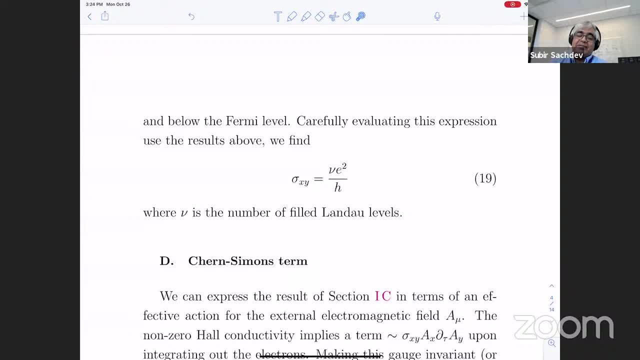 in the presence of disorder and some self-consistent bond approximation, and found again it was exactly equal to this, but it was felt that this is, you know, okay, this is some, some, some accident, and nothing, not nothing of particular attention. that was, of course, a big mistake because, as you know, 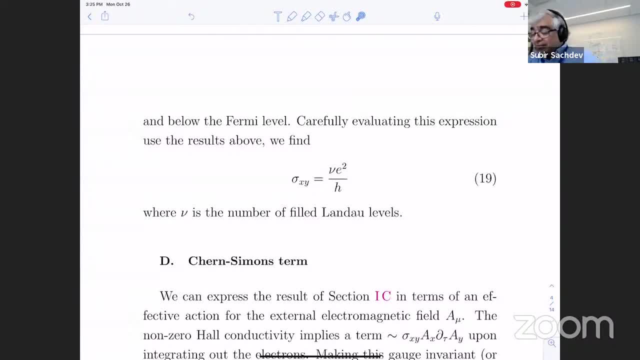 this turns out to be the exact value, with no corrections: uh, under certain conditions, at low temperature, uh, even in the presence of disorder, and even allowing for all kinds of electron electron interactions, electron phonon interactions, whatever you wish, they don't change this value. so that's the famous quantization of the hall. 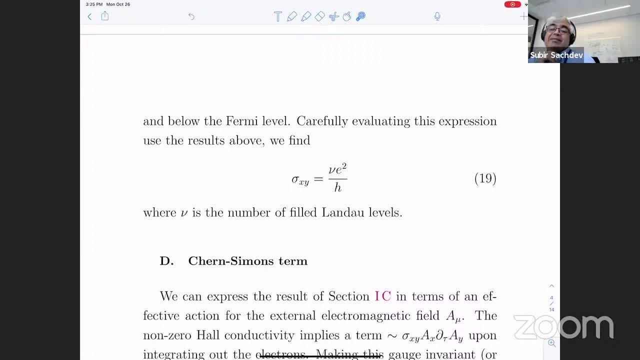 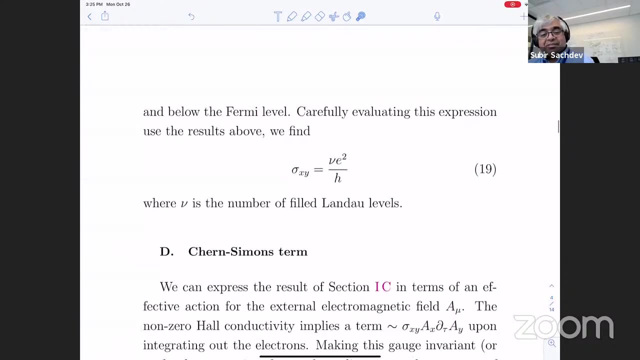 conductivity- which we haven't proven by any means, uh, but this is one. the fact that it came out with a simple number uh was a strong hit that somebody should have taken, and that's why it's so important, uh to look at this more carefully. uh, in the end, it was experiments that first gave a hint that. 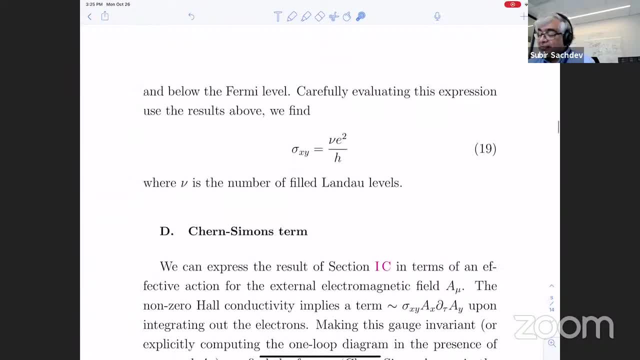 this is completely quantized. uh von klitzing did some experiments on semiconductors where you had a two-dimensional electron gas on the surface and he discovered the quantization experimentally and went ahead and claimed, to his credit, that it is quantized because, although he had no, 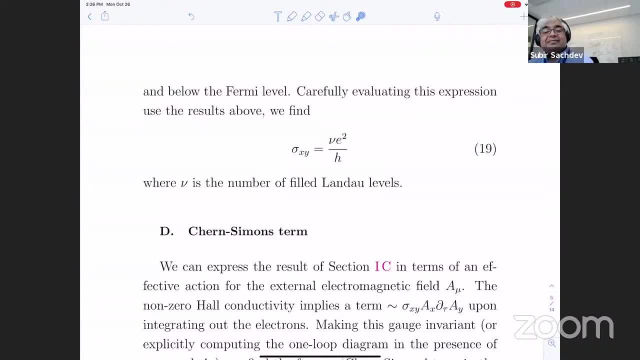 theoretical reason for suspecting. so that was smart, because that was a reason that he won the nobel prize for this discovery. okay, all right, so we'll get to this and there's various ways of understanding this quantization and we'll at least. i won't have a full proof, but we will give. 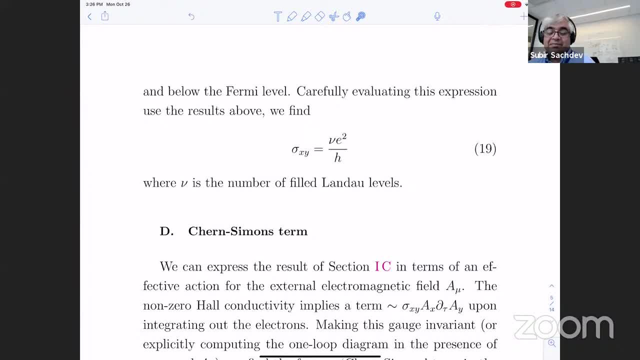 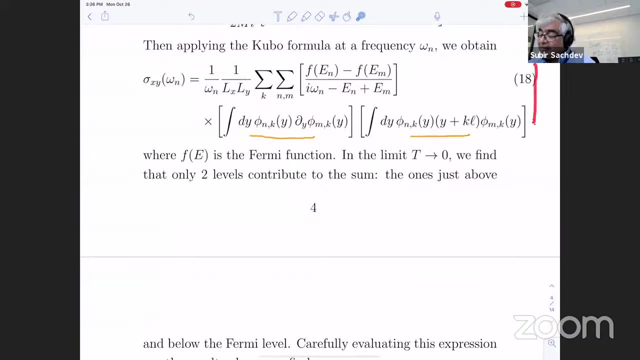 you at least a hand-waving argument of why this is correct, why it's quantized okay and- and in fact i i am also not going through all these very complicated calculation here, because later on we'll see a much simpler calculation that will give you the same answer- 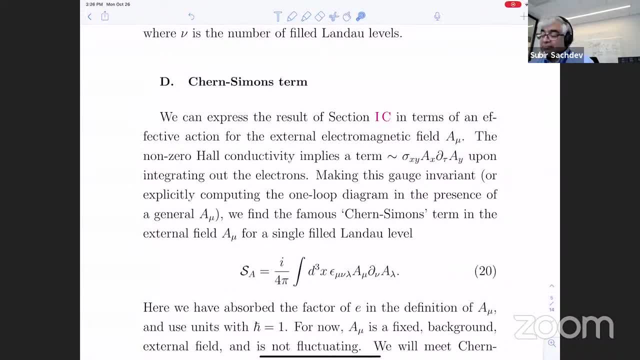 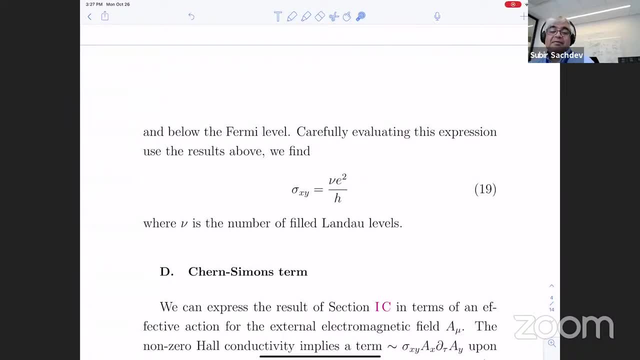 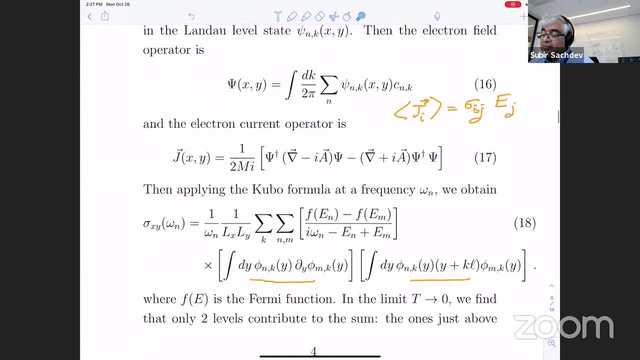 all right, okay, so before i start talking about the origin of corn, let me also re-express this result in a slightly different way. uh, so this is, i said, was a response, uh of of the system to to some general electric field. in fact, here i'm taking an electric field. 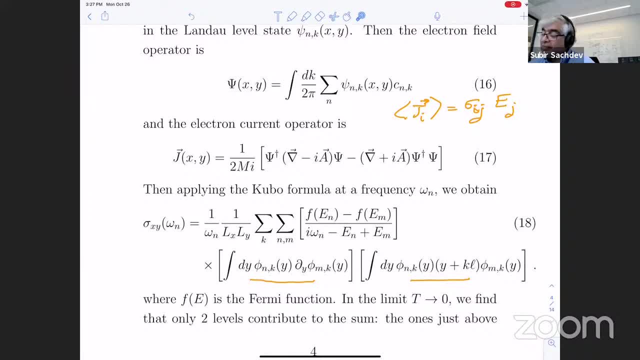 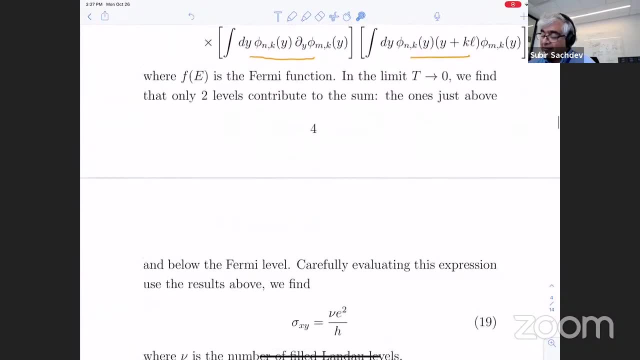 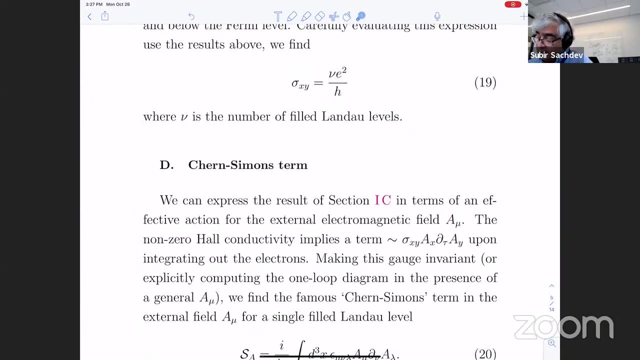 in the y direction and measuring the current in the x direction, uh, but by gauge invariance, you can kind of deduce what the answer should be: uh for arbitrary electromagnetic fields, and let's just see why that is so. okay, so you know. so the hall conductivity: 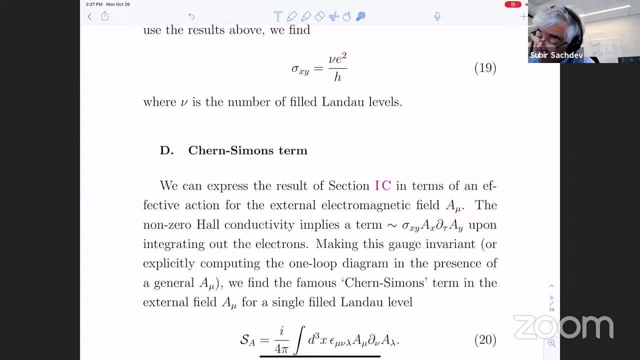 is the. you know what is the whole conductivity is the current. the current which is the uh, the change of the action with respect to, you know, just j sub r. well, it's the current in the x direction, let's say to a sub x, and that's equal to the Sigma X, Y times the electric field. 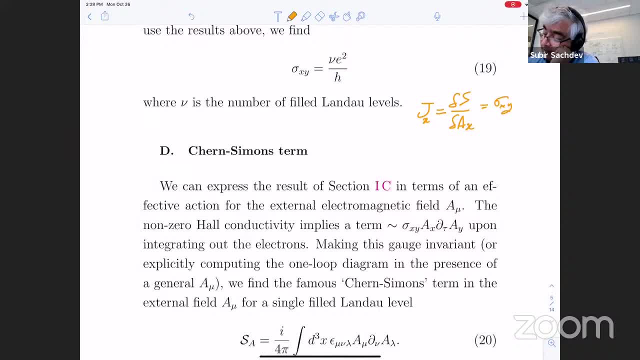 The electric field is D, A, Y, D, T in the Y direction, So it's Omega times A, Y. So the Hall conductivity corresponds to term in the action. So there's a term in the action which is Omega times, Sigma, X, Y, which is just a number times A, X, A, Y. 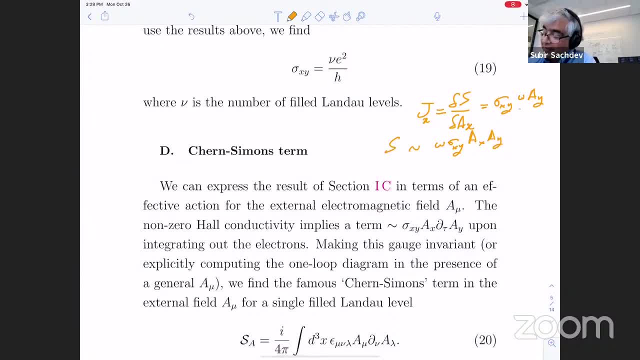 Okay, this is just. you know, the electric field is D, A, D, T. That's what I'm, that's the gauge that I'm using. So now we want to make this gauge invariant, Sorry. what is the electric field? 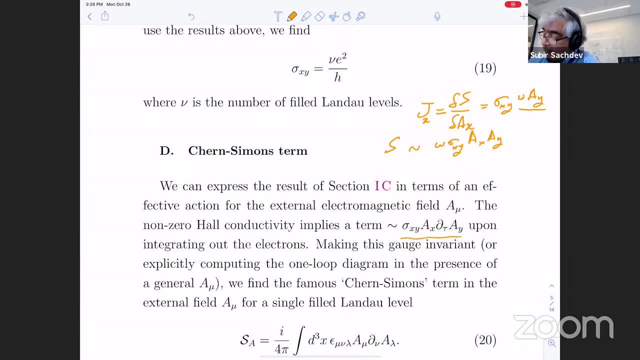 Yeah, that's correct. Okay, yeah, I wrote it right. All right, so this is the term. So now we want to make this fully gauge invariant and we want to compute the response for an arbitrary A mu A nu, And so basically, you have a bilinear in A, mu in A here. 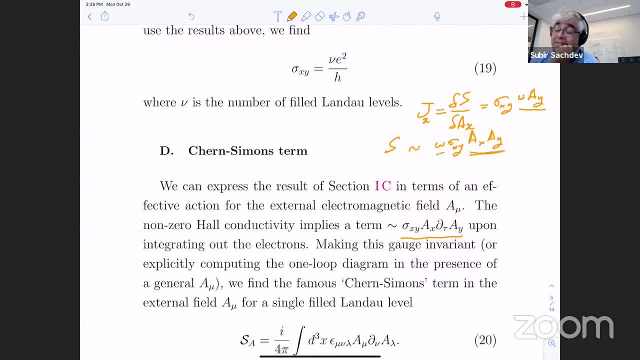 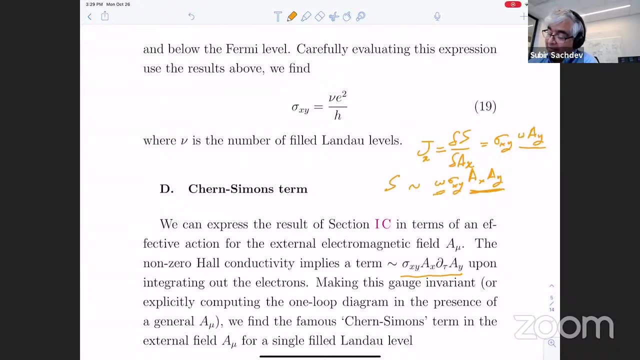 And how am I going to? with one derivative? So is there, is there some expression which is gauge invariant, which is which has one derivative of space, time and two product of A? Of course, we already know an expression which has two derivatives, which is gauge invariant. 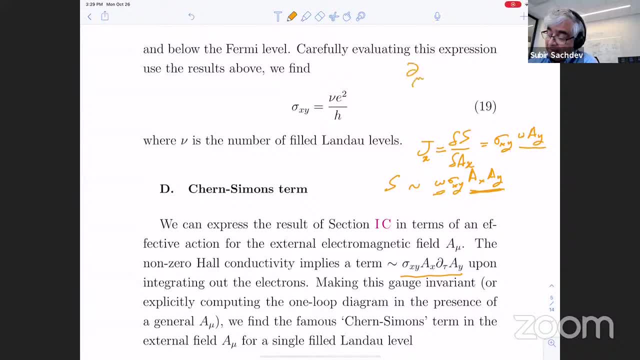 That's this. you know, that's the Maxwell term. The Maxwell term is D mu A nu minus D nu A mu whole squared. So that's the Maxwell term in the action, as you learned in your electro-dynamics course. But that has too many derivatives. 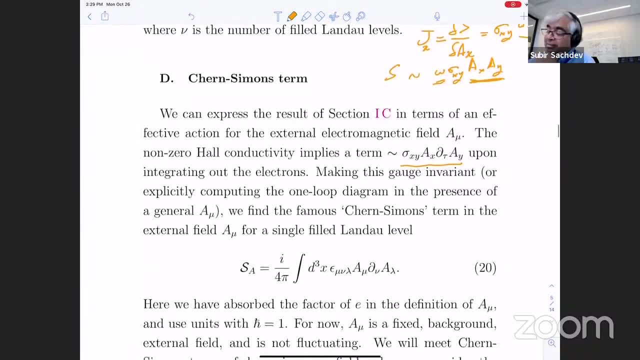 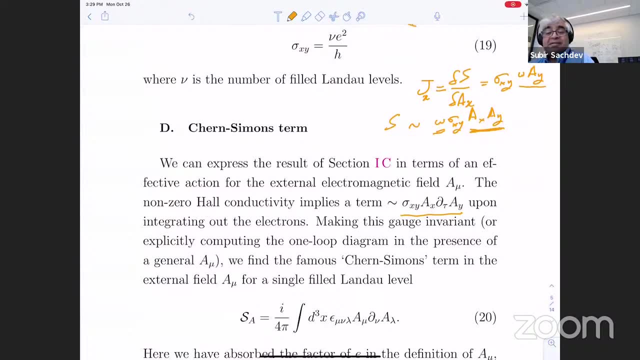 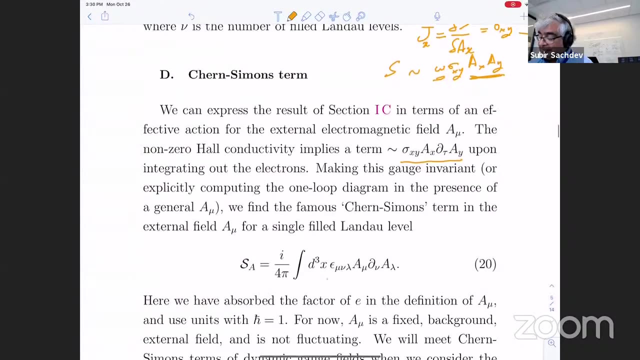 So here the question is: is there any term that has the right structure? Just one derivative, And it turns out in two plus one dimensions, and the two dimensionality is important here. There is such a term, And that's the famous Chern-Simons term. 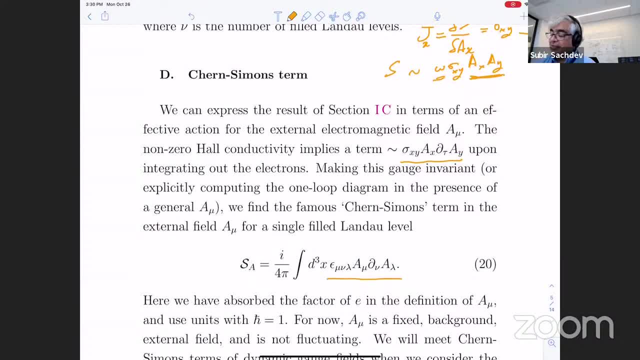 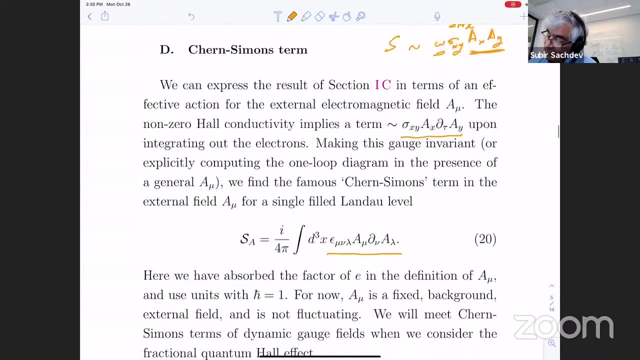 which is written right here. Okay, so here, mu, nu and lambda extend from over three indices: x, y and tau, As and so- and this term turns out to be gauge, invariant, almost, And the almost will play a crucial role. 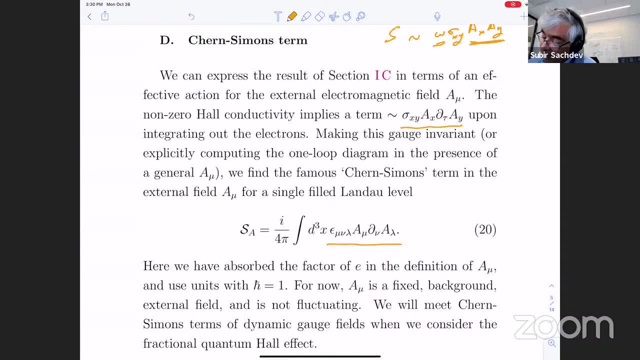 But for now, if you're just looking at things in the bulk, what happens if you make a gauge transformation? A? mu goes to A mu plus D mu lambda. Well, you can see that this combination is already gauged invariant because of the epsilon mu nu lambda there. 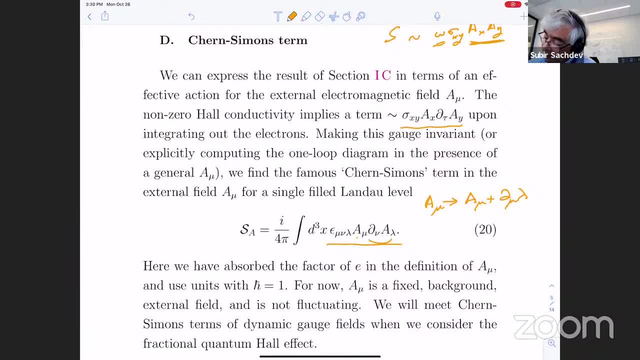 But what about this term in the front? Well, the term in the front will give you D mu lambda as a change times. D nu A lambda. This is two degrees. Okay, Two different lambdas. The indices lambda have nothing to do with that lambda. 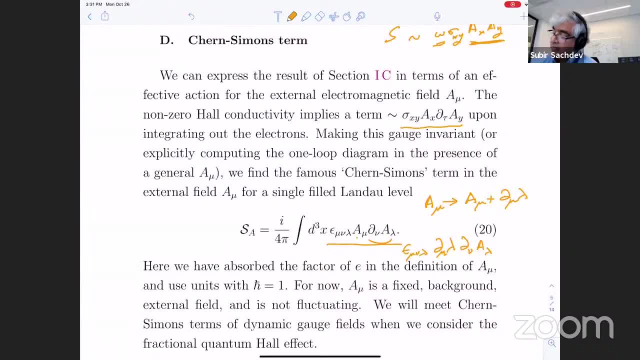 Epsilon mu nu lambda. Now that's not zero, but after integration by parts. if I bring this over to this side, then it's zero. So this is gauge invariant after integration by part, or in other words, up to surface terms. 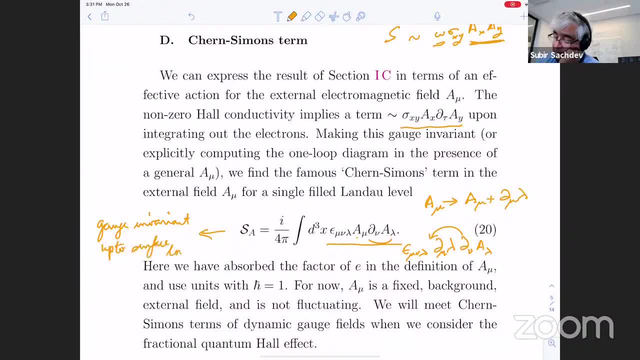 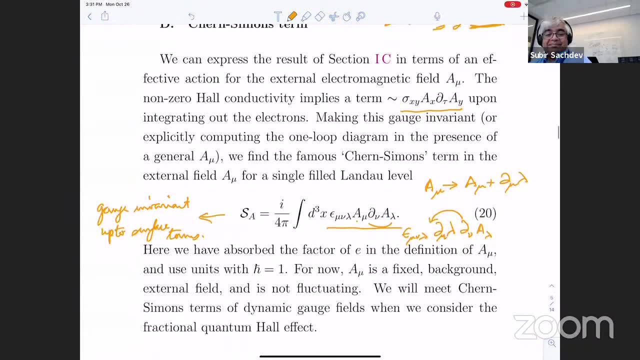 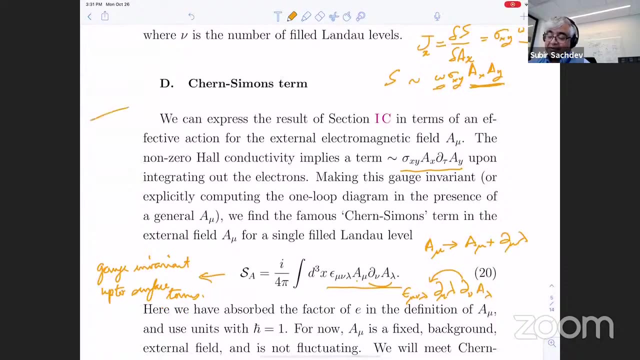 So what we have worked out is that if you have an electron gas which is sitting in the lowest Landau level, so here's your Landau levels, and then this is filled, So that's at a very low temperatures. Now those states are all filled. 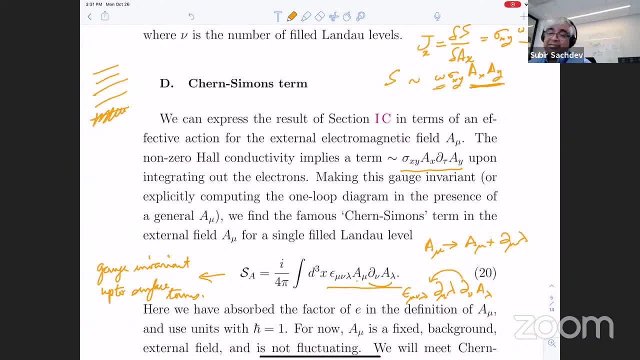 and all the states that are not filled are above some gap. So basically it's just a very low temperature. So you're out in the warm front. It's just a vegetable sitting there. No excitation is some quantum state or matter. 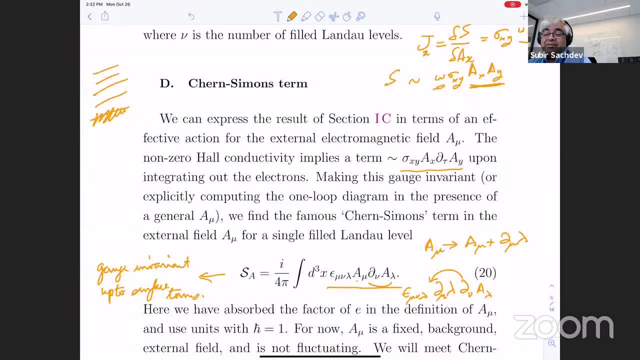 Now. what I want to do, therefore, is figure out how it influences electro electrodynamics. You know, this is the analog of figuring out the dielectric constant. you know, and we, when you have an insulator sitting there. 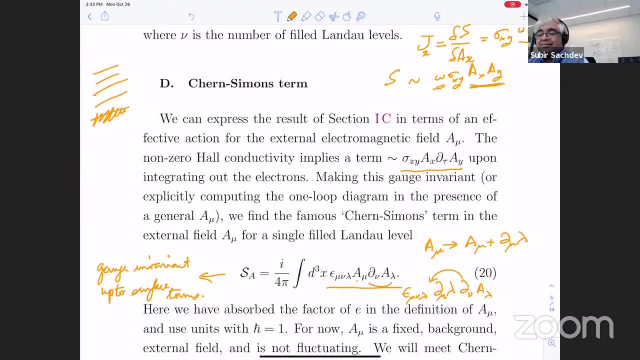 well, it does influence electrodynamics because it there's a dielectric constant and a magnetic permeability that determines how fast light will propagate. So that's what I'm asking to do, that insulator. so the way you can express that is what you imagine. you have some piece of matter. 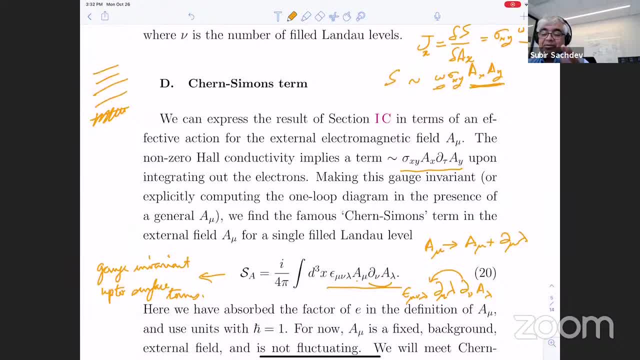 coupled to electromagnetism. it's an insulator because it has a gap. we just do a path integral where you integrate out all the electrons. if you integrate out all the electrons, you end up with a new theory for electrodynamics where the Maxwell action has been corrected. it's got a new term. 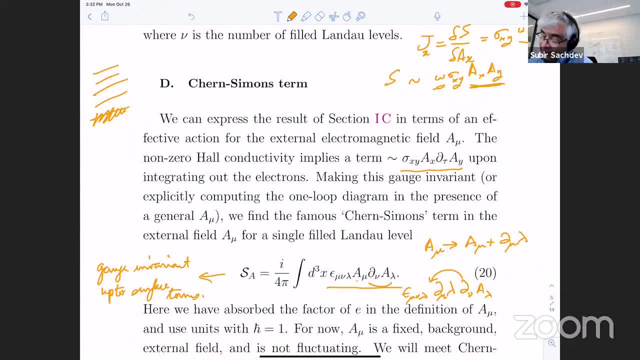 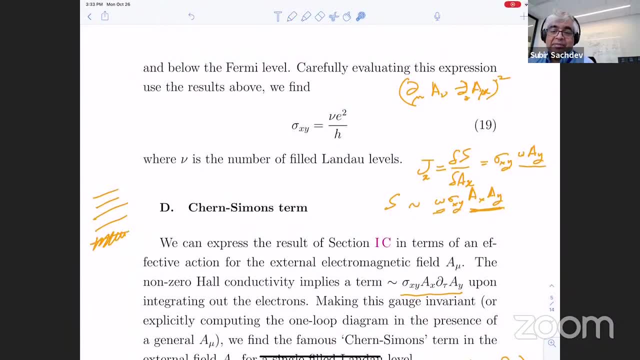 and normally you correct the bare Maxwell action by just changing the coefficient of this, this kind of term, over here, and that's where you get dielectric constants and magnetic permeabilities. but here you get a new term that you didn't have before and it's allowed because of this. 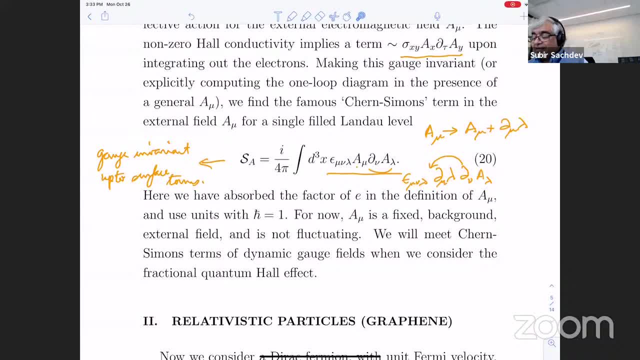 fixed magnetic field that I'm expanding about that break time reversal this thing does and it's this Chen-Simons term. so this is the, the new term that appears in the theory for electrodynamics in the presence of a fully filled land or level this, but not quite gauge invariant term. 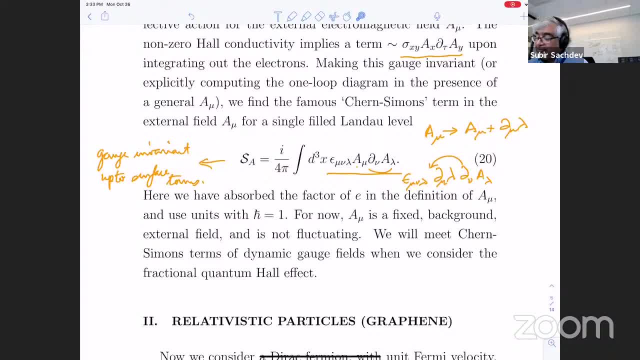 okay, so this Chen-Simons term is going to occupy us really for the next few weeks. it's a. it's an amazing, uh has amazing consequences in all kinds. but over here right now, um, its consequence is simply that there's a whole conductivity is its coefficient, and if you put in all the 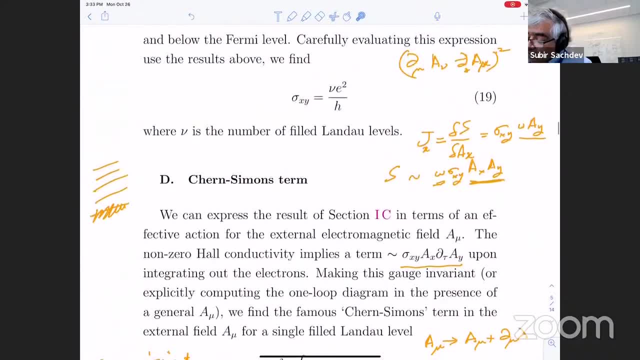 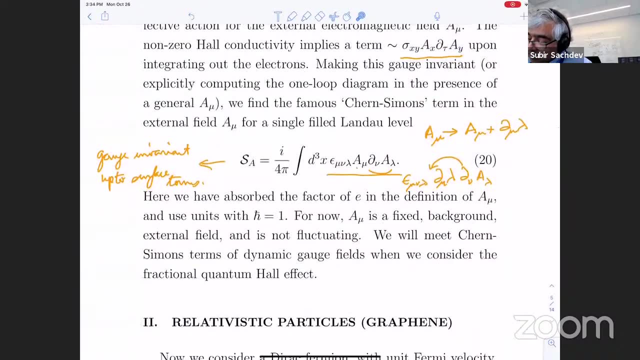 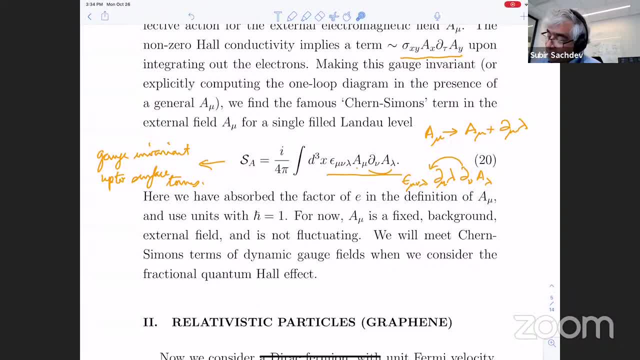 if you just keep track of exactly where everything is going. so in fact you know this term. in units where h bar is one is just dimensionless, because a mu has the dimensions of inverse length, and then so the integral d, three x, uh meets three factors of inverse length. so just a pure number, um, and it comes with, it's a phase factor and as 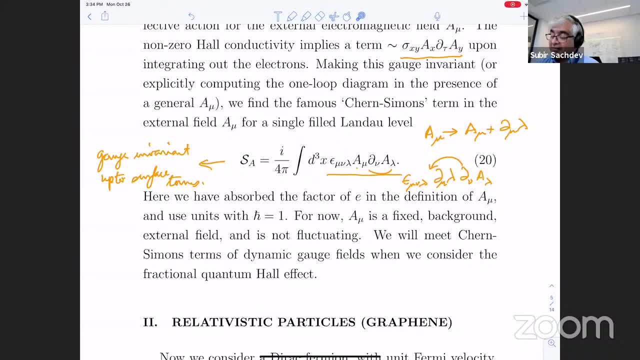 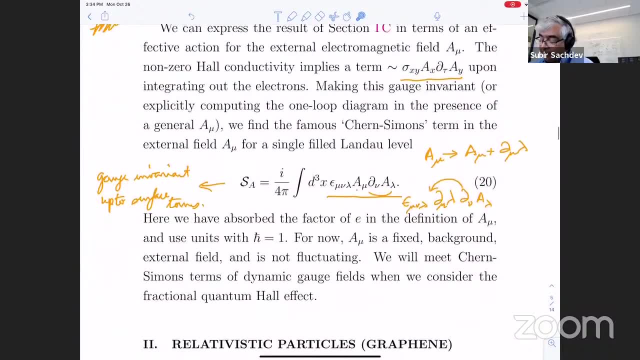 we'll see. um, you know, it's sort of like a berry phase term which will have lots of interesting consequences. one of it so far is just this: sigma x, y, all right, so I'm not going to do much to this, except this is a good time to introduce the. 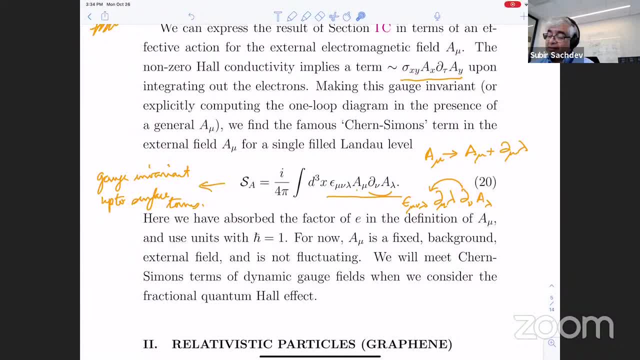 Chen-Simons term. you know, for for us, as far as we are concerned, the external electromagnetic field is a fixed field. you know, for for us, as far as we are concerned, the external electromagnetic field is a fixed field. it's just something that I'm controlling with knobs in the laboratory. it's not a. 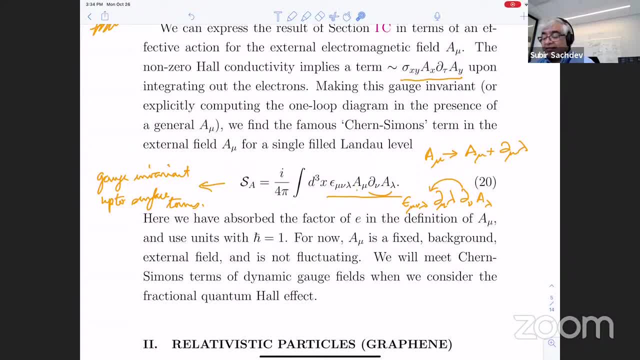 quantum degree of freedom. yet it's a background field, um, because quantum fluctuations of electromagnetism itself are extremely weak for at the condensed matter energy scale. but pretty soon we'll talk about other gauge fields. there'll be emergent gauge fields which will also acquire this Chen-Simons term. and for those emergent gauge fields, 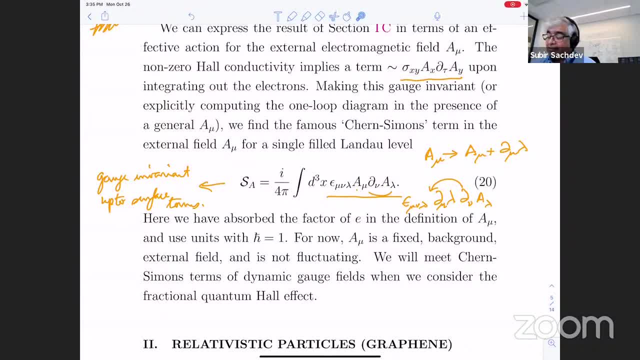 I will have to treat them as quantum theory. they will have to be fluctuating. they're not background, because they have. you know, there is no fine structure constant that makes their fluctuations weak. okay, any question? okay, just as another aside, let me quickly mention that you can. 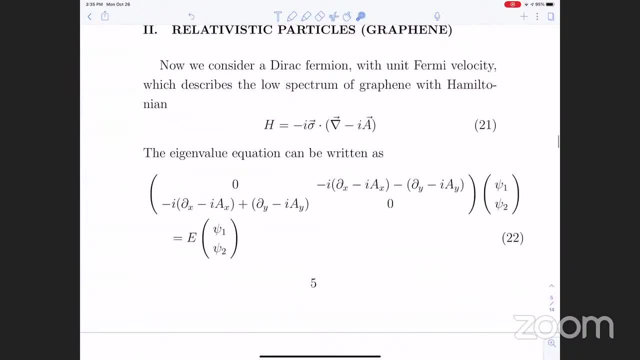 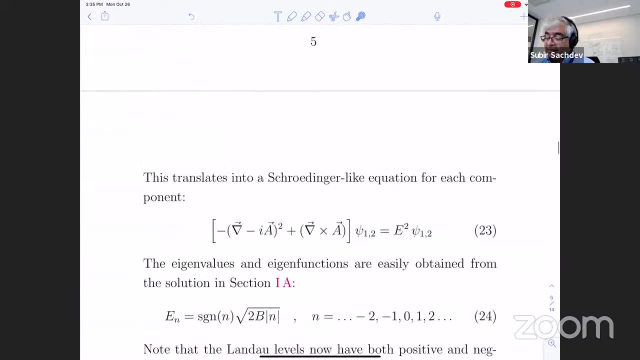 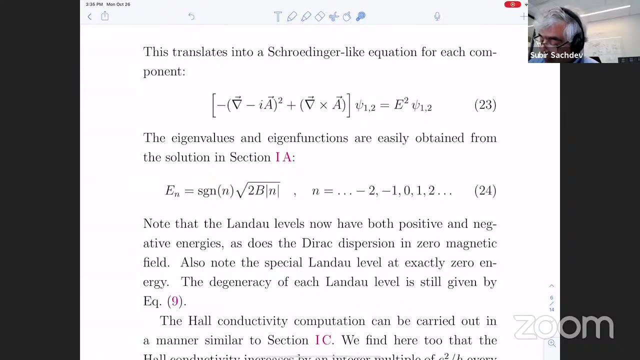 redo the same thing for graphene, where you have relativistic particles. I won't go through the details. you have to solve a two by two matrix equation. you can certainly look it up- and then you find that the energy levels have this, this result here. so first of all, just 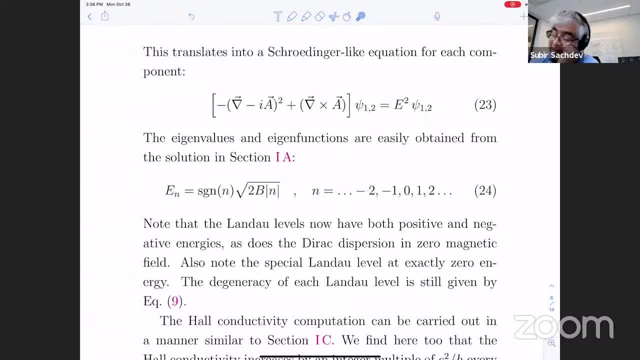 like graphene, has a direct dispersion that I'm sure you've seen before. so in the, in the absence of a magnetic field, you have this uh, conical direct dispersion where the Fermi level, let's say, is here. so these states are all occupied and those states are empty. 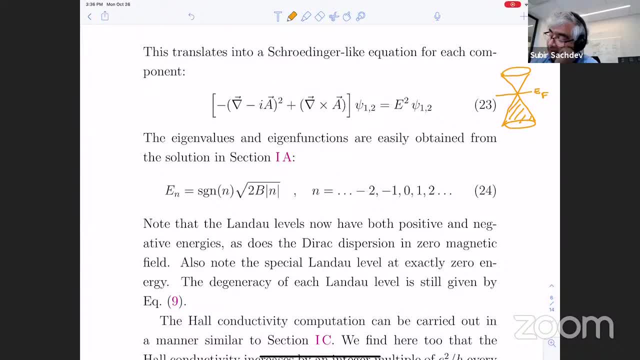 um, and then when you apply a magnetic field, this dispersion breaks up into again Landau levels. but now the Landau levels are not uniformly spaced. uh, I think I'm drawing it the wrong way. and there's it goes, the square root of no, it's fine. okay, the spacing is square root of n. 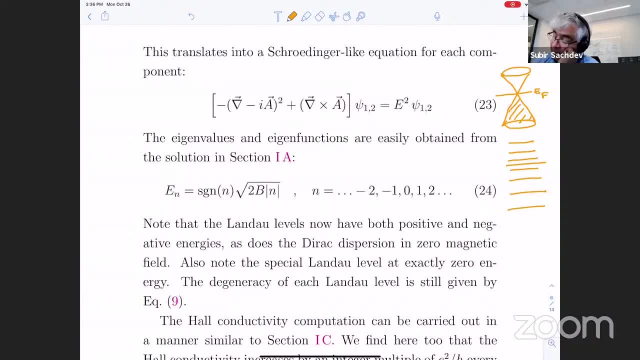 the energy is uh. square root of n. uh, So the spacing. I think it becomes smaller as you go farther away, not the way I've drawn it. So there's the zeroth level and the first level is a square root of 2b. 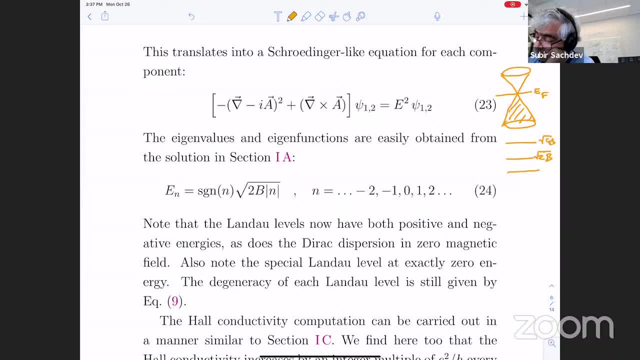 Second level is a square root of 4b and so on. You can get closer. Sorry about this. Okay, there, I think myself can tell. Yeah, so this is the zeroth one here. Okay, All right, so they're not equally spaced and they go from minus infinity to infinity. 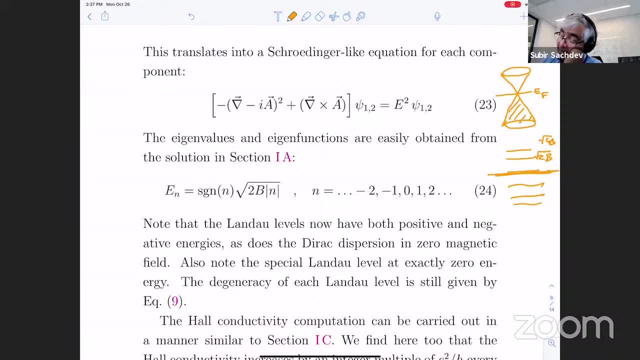 But of course the lower ones, They're going to be filled, just like the negative Dirac C at zero magnetic field over here. These states will be filled and those up above will be empty And anyway. but there's another subtlety here in the computation of the whole conductivity. 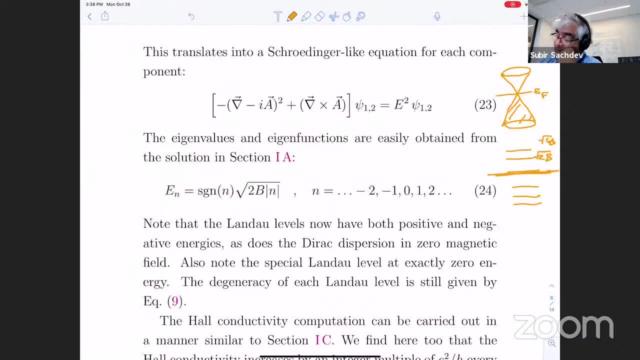 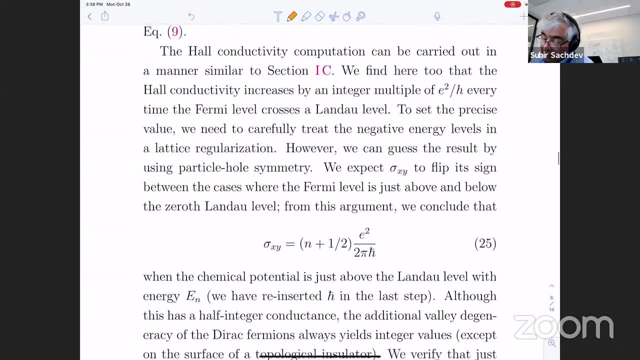 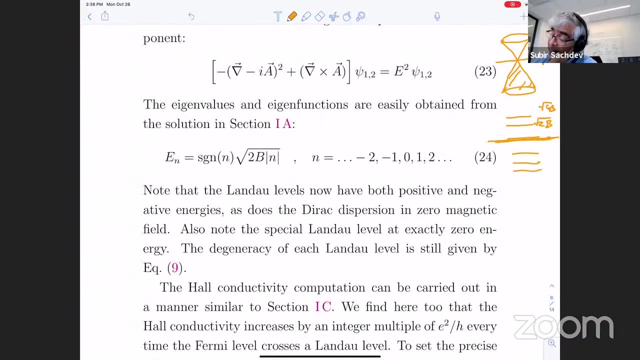 What is sigma xy of these levels? Okay, so again you can go through the calculation. It's a bit tedious And what you do, what you do find you know. first of all, you say you start doing the computation when your energy level is sitting here, right? 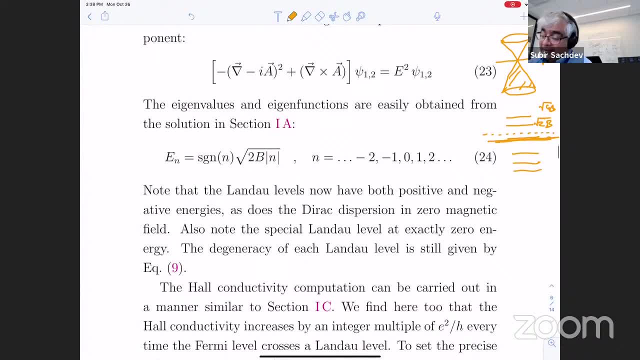 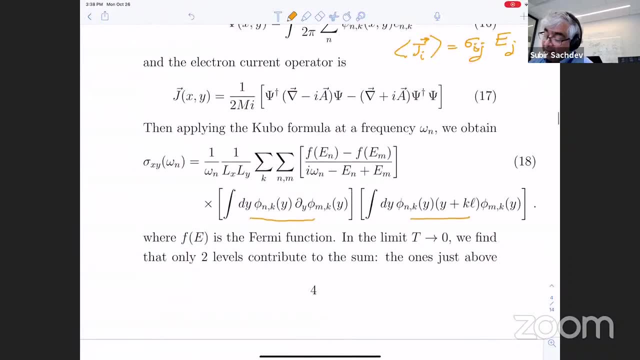 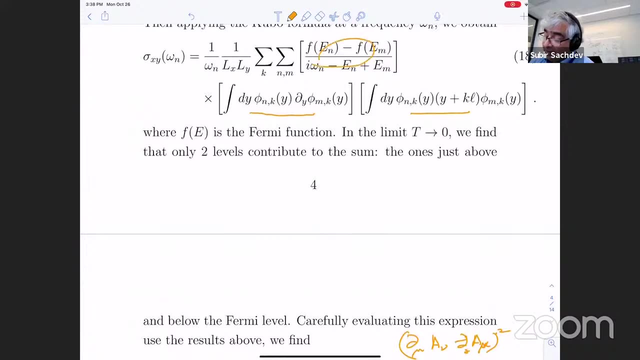 Fermi level is sitting here. Then, as for the free particle with a k-squared dispersion, you'll find, as I say here, that only two levels contribute to this. This is horrible, You know, you can get off the surface, but you can't get to the top of the surface. You can't get to the bottom of the surface. So if you assume that you have two levels, you'll find that one is filled. You're going to have two levels that are filled. So if you assume that you have two levels that are filled, then you're going to have two levels that are filled. 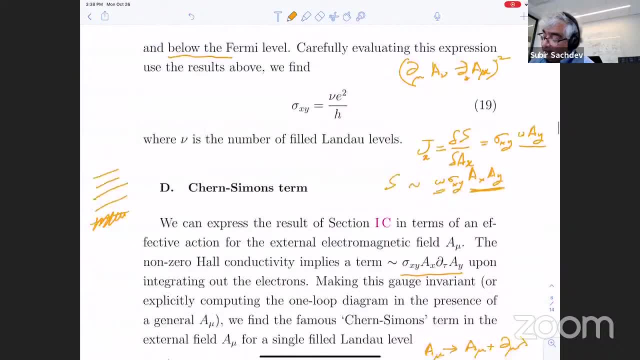 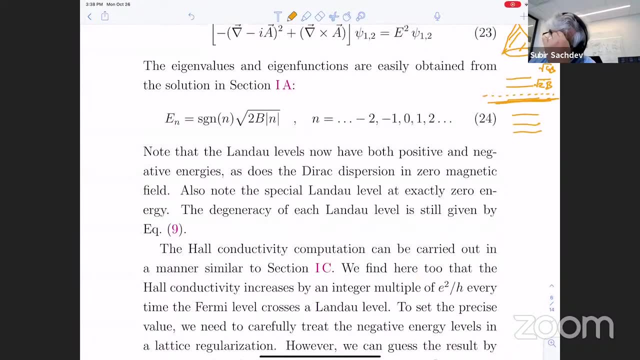 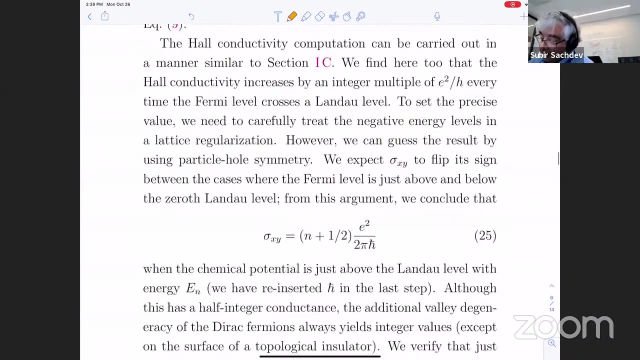 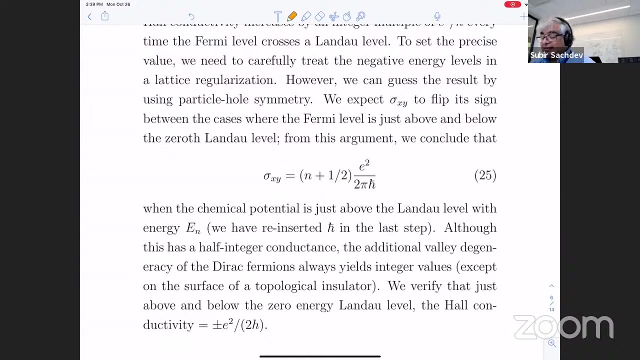 And that one is just above and just below the Fermi level. Okay, So if you assume that all the ones below the Fermi level are filled and your Fermi is here, you only need to take two of these into account And you do the computation. you'll find that actually now the answer, amazingly, is not an integer at time g squared. 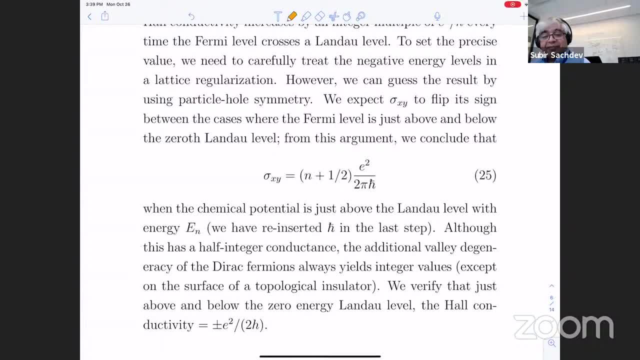 over H. It turns out to be half integers times each of E squared over H. per valley, per direct point. Now it turns out graphene has two direct points, so you have to multiply this answer by two so you don't actually see a half integer sigma XY. But if you were able to somehow 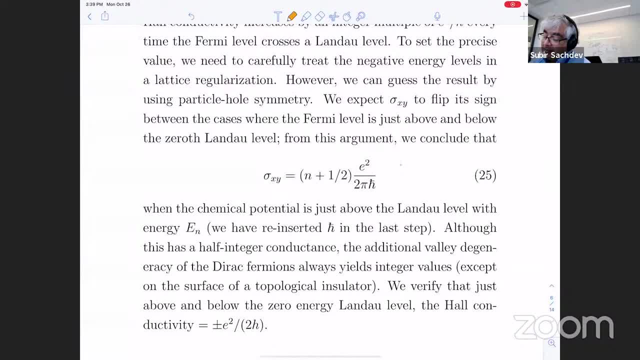 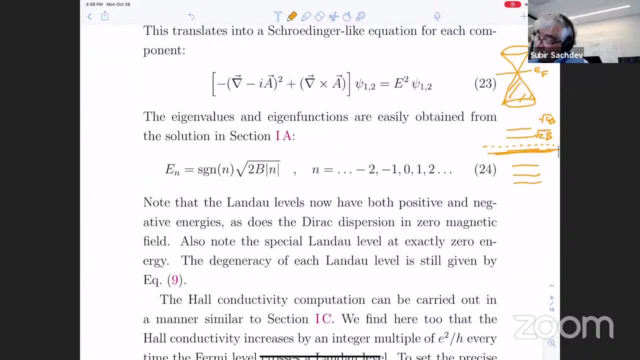 compute sigma XY for a single direct cone, then you would get this half integer conductivity. And one way to understand this is the following: So, just like in ordinary non-relativistic electrons, every time your Fermi level crosses the Landau level, the Hall conductivity jumps by one. 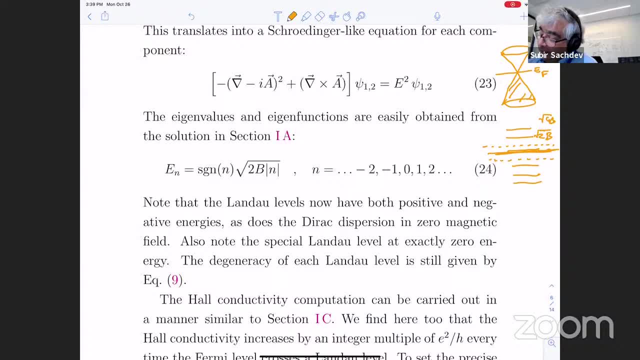 in multiples of E squared over H. On the other hand, if you were here and here the Hall, conductivity is a flip sign. because of particle-hole symmetry, You could work with particles in respect to hole. These two should have basically the same properties. 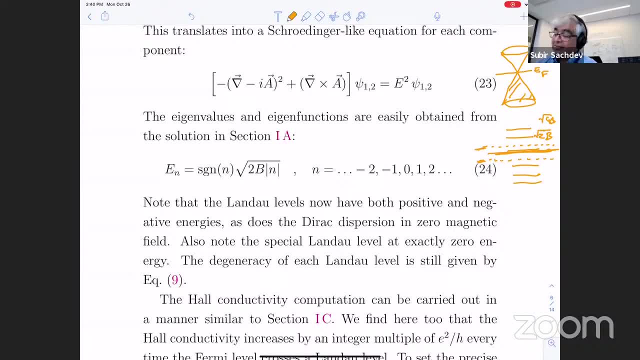 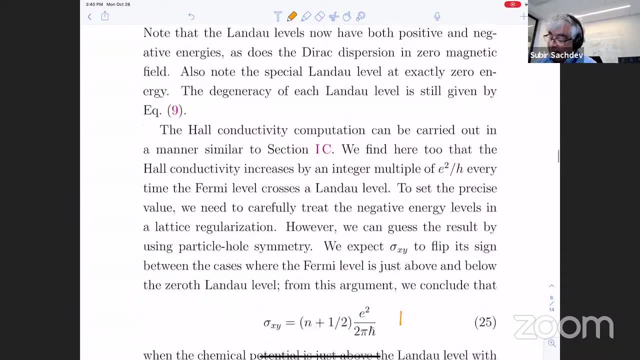 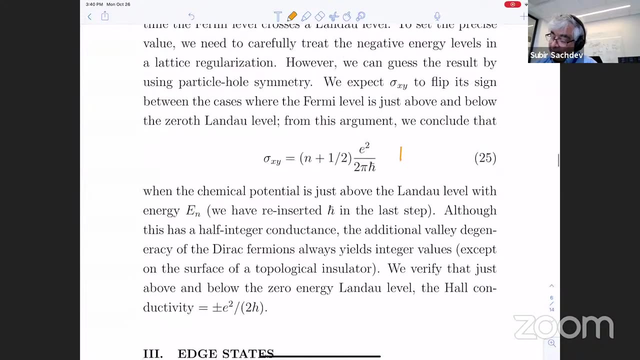 And so if you shift by one as you cross the zero's Landau level, then the only possibility is you go from minus half to half, And that's what accounts for this extra one half. one way to understand it: To really see half integer quantized Hall effect, you need just one direct. 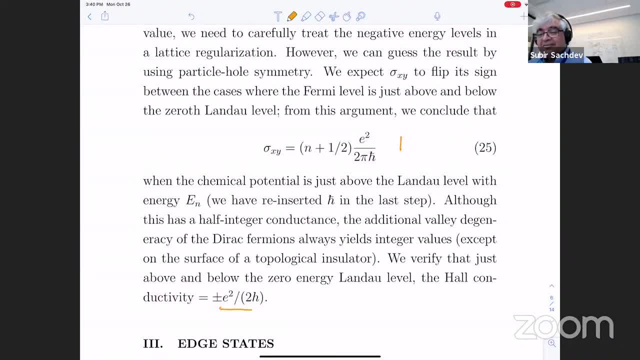 cone, And that can only happen in SPT phases on the surface of a topological insulator, As I hope to show you eventually. Okay, More questions Or any questions. Sorry, No one said anything. All right, So now let's move on to something non-trivial. Well, this is also quite non-trivial. 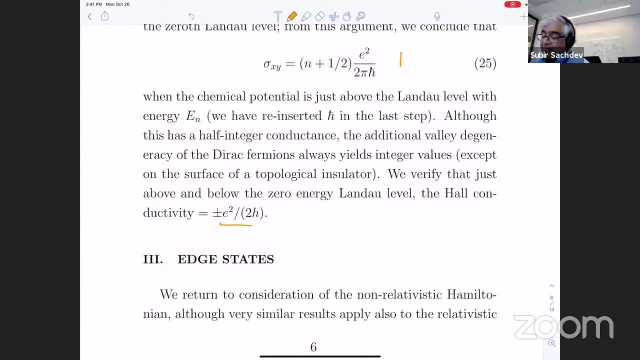 but it's all one series of amazing special properties after the other And you might have, you know, can't help but wonder- it's because you're considering such simple models- How could these, some of these properties you found be generically measurable? 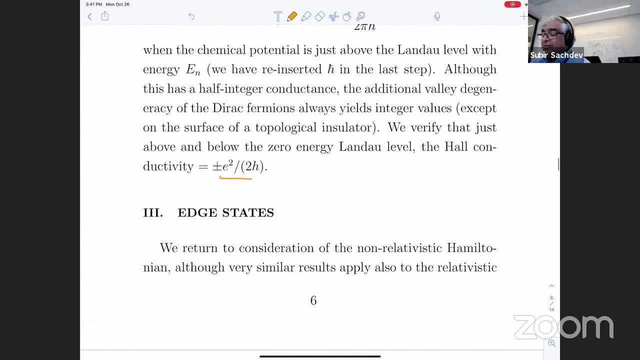 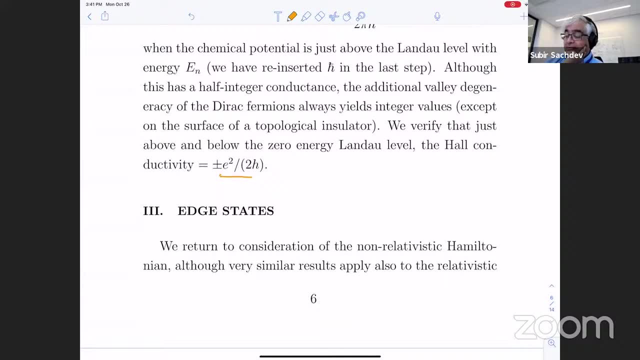 Okay. So to understand what's going on, it's absolutely crucial. it turns out to not take an infinite sample in space. So far I've been talking about just infinite samples and trying to compute just the way you normally do in condensed matter physics. any response? 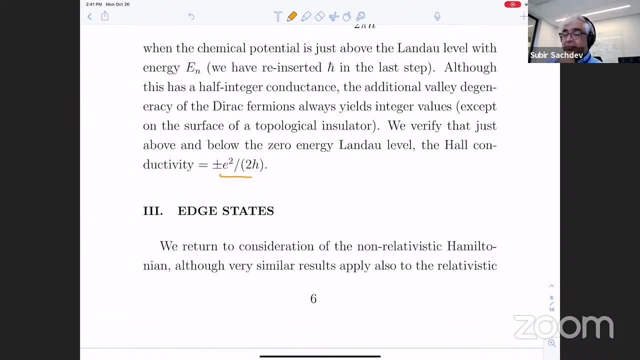 function by just doing some computing, So you can do some Green's function and integrating over momenta and it gives you the answer. It turns out that the states that give you this quantized Hall conductance are, you know, are mostly at the edge of the sample. Any sample has an edge in the real world And 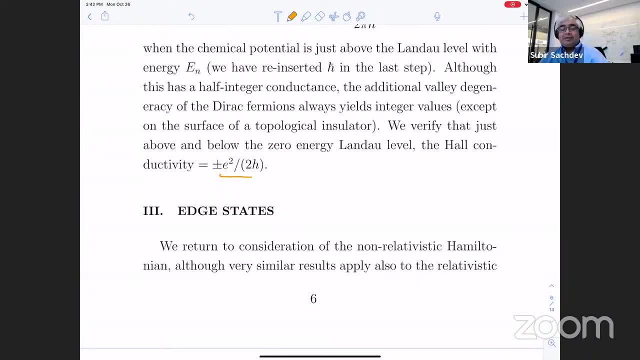 so we really want to think about the physics of the quantum Hall effect in the presence of an edge. So far we're not going to include any interactions now, but we want to see what happens on the edge of a, of a corner, of a quantum Hall sample, And what happens is something extremely 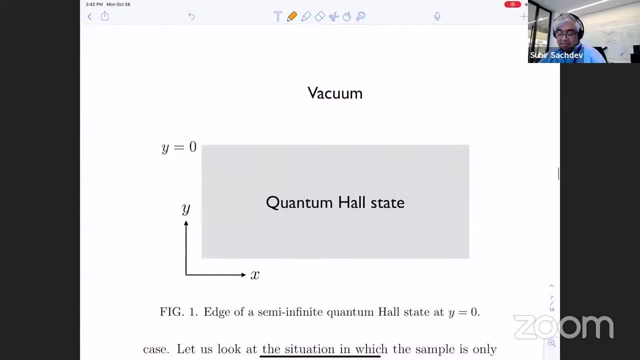 interesting. So we consider the following geometry: So along the y direction we're going to introduce some potential V of y And the potential will be such that it's very weak over here And becomes very strong. So all the electrons are in the negative y, They're just trapped in the y less than. 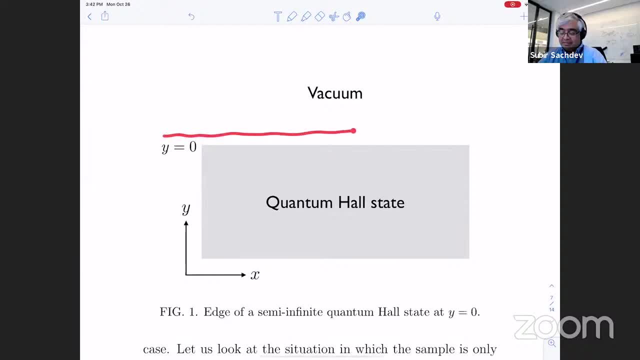 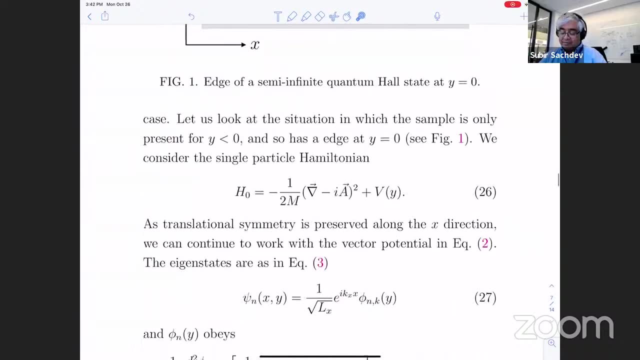 zero region. So we have an edge. Here's our edge: separating our quantum Hall state with a vacuum. Okay, So basically, all we have to do is add this function: V of y And V of y. you know this. 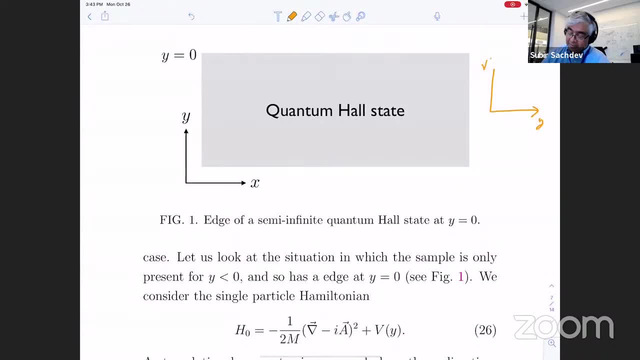 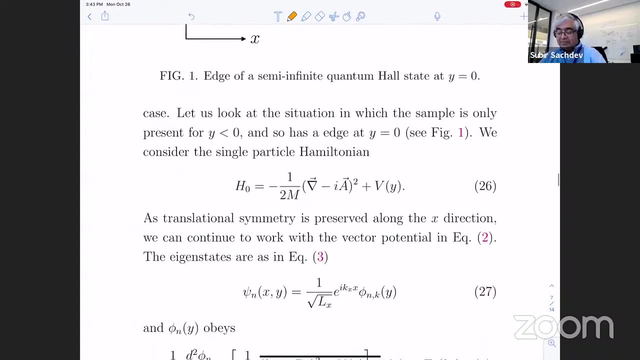 is y, This is v. Then for y negative, it's y less than zero, It's almost zero, And then it zooms up as y becomes positive. So all the electrons are in the negative y direction. All we have to do is just add this potential V of y. 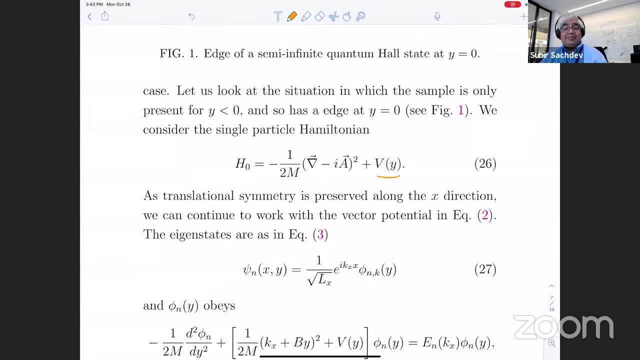 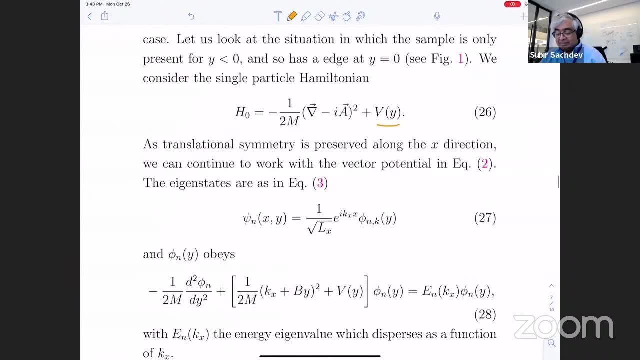 Now, fortunately, that turns out to be not so hard to do, At least in the Landau gauge. So this is why I chose Landau gauge before, Because in this gauge it's still true that there's complete translational symmetry in. 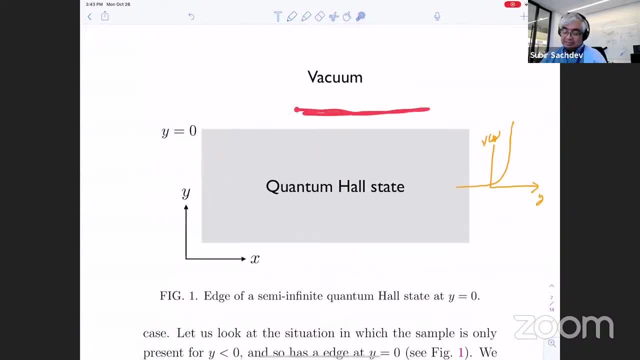 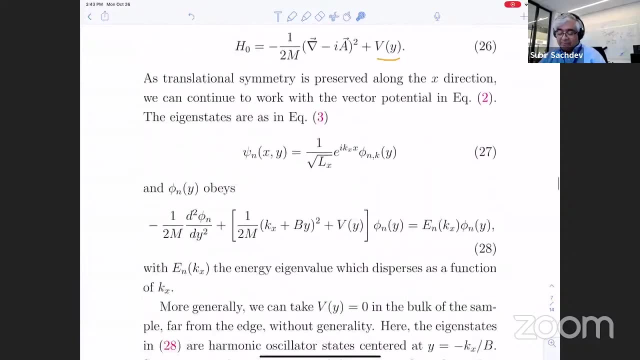 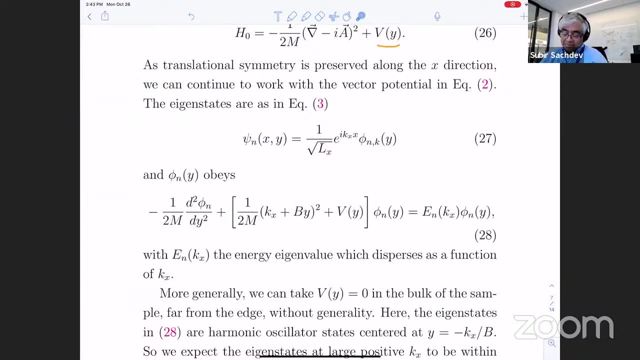 the x direction. So along this direction things are still translationally invariant, even though they're not in this direction, And so I can still write my wave function as a plane wave along the x direction. So everything goes through as before. 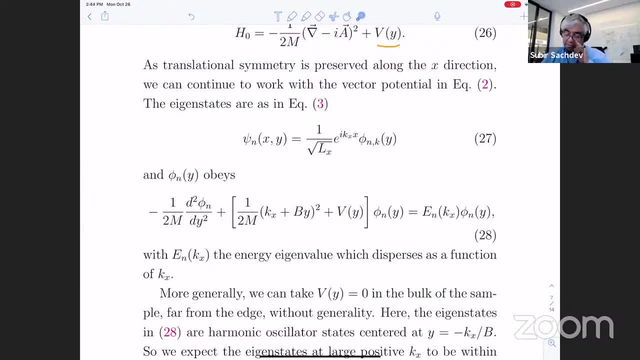 The only change is there's some other potential V of y here. It's not a purely harmonic potential. Okay, All right, So what's going to happen now? So you have a new potential to deal with, But what makes this easier to see what's going on is that the potential V of y is on a very 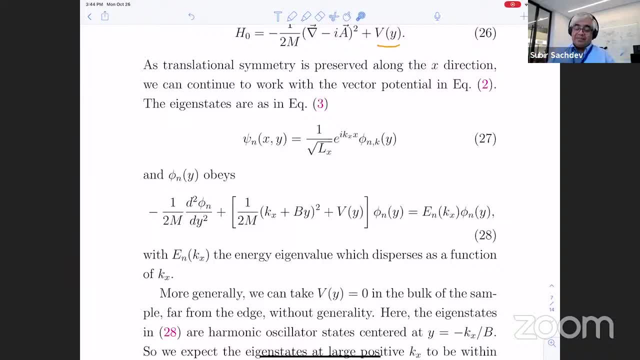 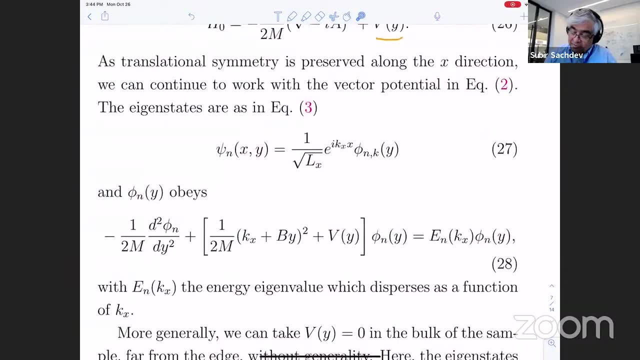 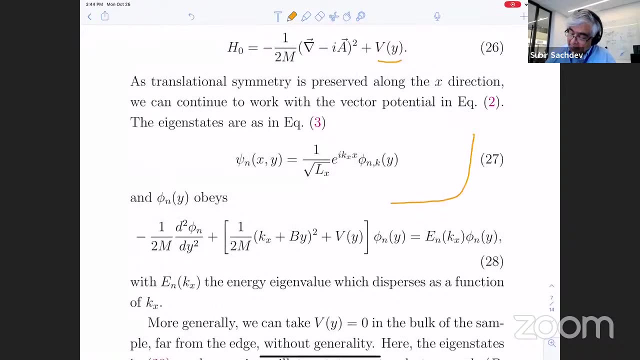 long macroscopic scale It varies, Whereas this is something microscopic on the scale of a magnetic length. Okay, So here's your potential, Here's our potential. V of y, And suppose I took an original wave function which is a Gaussian. 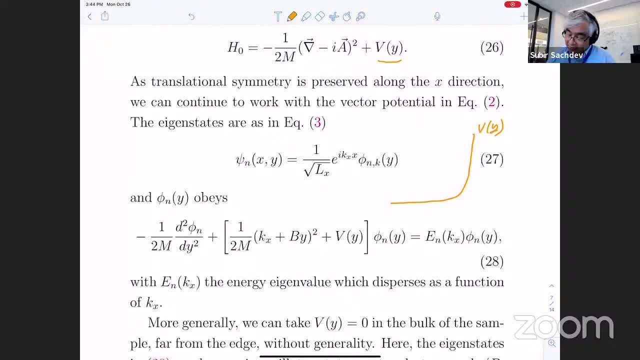 Let's stick ourselves to the lowest Landau level, And it was a Gaussian, which is somewhere here. So if you were here at the location of this point, this is y equals minus k, L squared. So you pick a k that tells you where the y is. 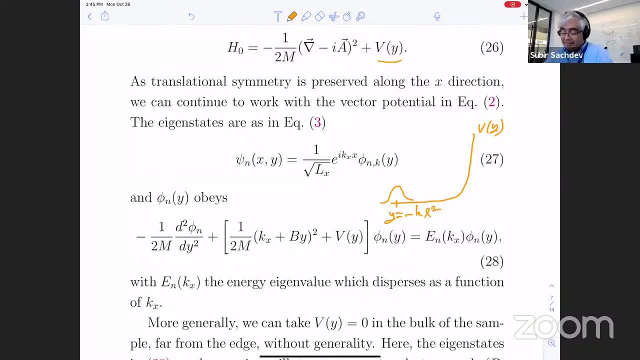 If the y is way inside the sample, no big deal. Its energy is not going to change Because the potential is just flat there, Just an overall shift, but that all states experience that shift. But as you change the value of k, as this state comes here, then its energy is going. 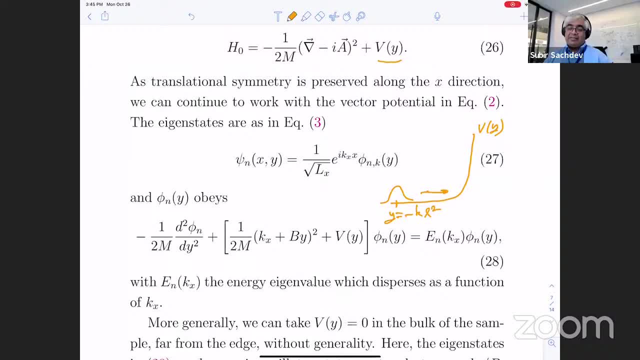 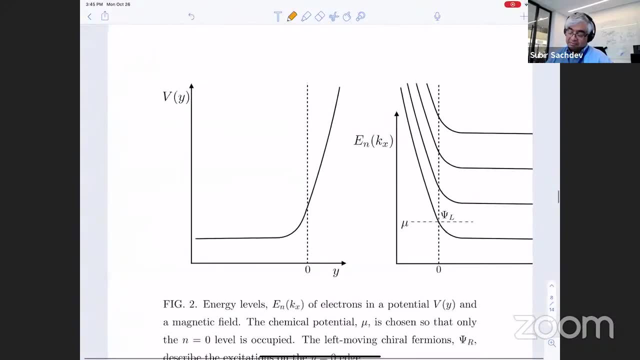 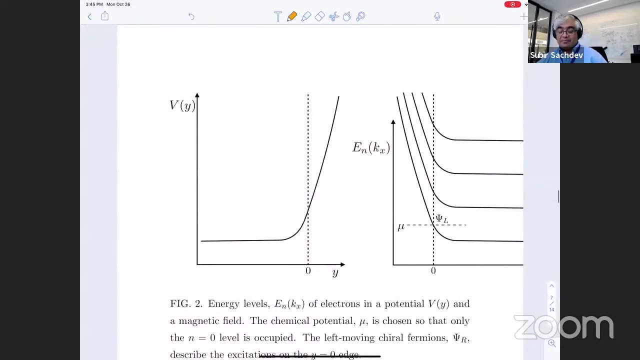 to go way up. So we're going to find that the energy which previously was independent of k will now become dependent on k. So here's the picture. Okay, So here's V of y. Yeah, the picture, Yeah. 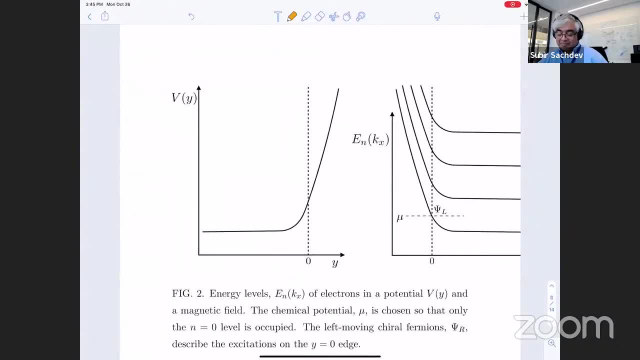 Okay, And here's the energy as a function of kx, So the particles are running in this direction And as they're running in this direction, they have a dispersion. Okay, So this is the Landau level deep in the sample. 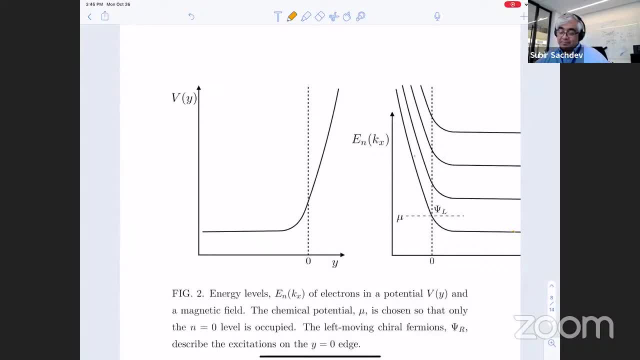 And as it hits the edge it starts to move up. So it goes over here in the bulk of the sample And then the energy starts to move up, And you can see that that will happen for all the other Landau levels too. 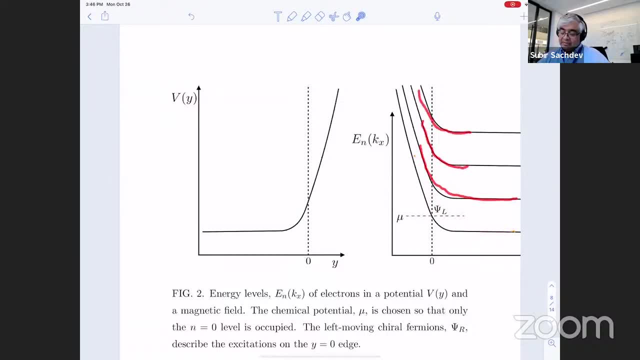 They'll all start to move up as you hit the edge And so as a function, but they're still, you know, plane waves along the x direction, And as you're moving along the x direction, the energy is different. Okay. 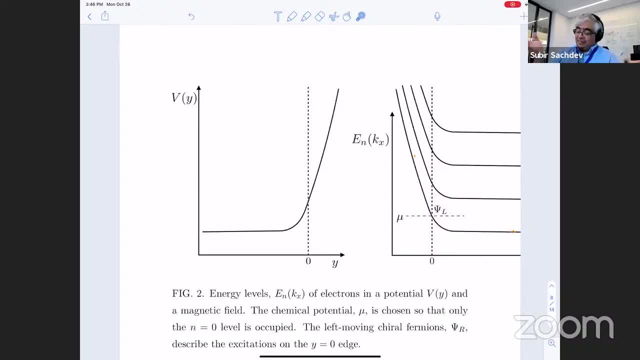 So what are we going to do now? Well, we've got some energy levels that are. they're not totally flat, They depend on kx, But these are free electrons for us right now And we're going to fill them up up to some chemical potential. 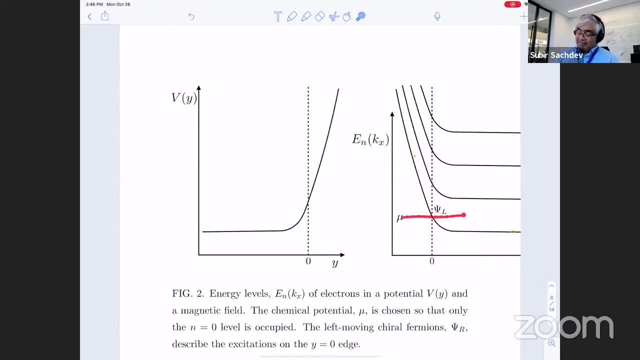 So I consider the case where the chemical potential was between the first and the second Landau levels Right here. So previously I just said these states were all full and these states were all empty, But now I see that near the edge something more interesting is going on. 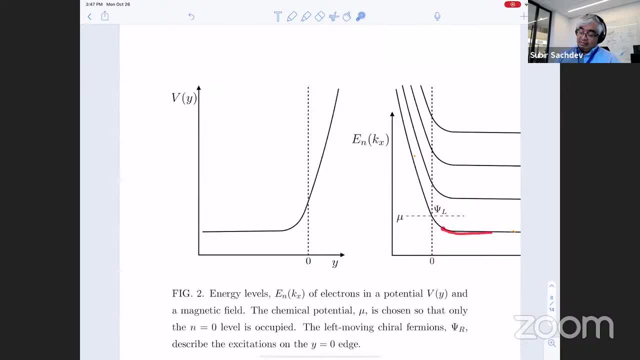 As I change the value of kx, the chemical potential goes, I mean, the energy goes right through mu. Okay, So this direction here, remember, is just kx, This is just kx, And what I have then is a Fermi point. 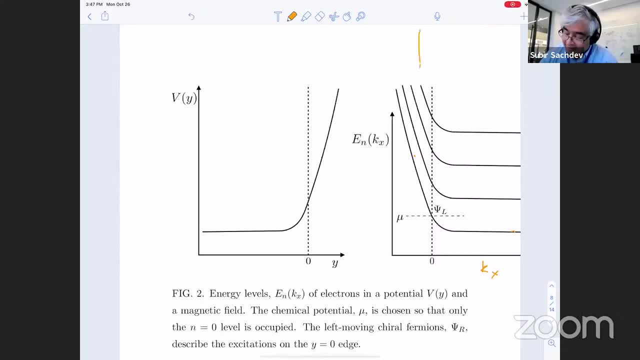 Just like in a. you know, normally if I had a crystal, I draw the Brillouin zone, This is kx, And then I say, well, here's some dispersion And here's my Fermi level. And these states are occupied. 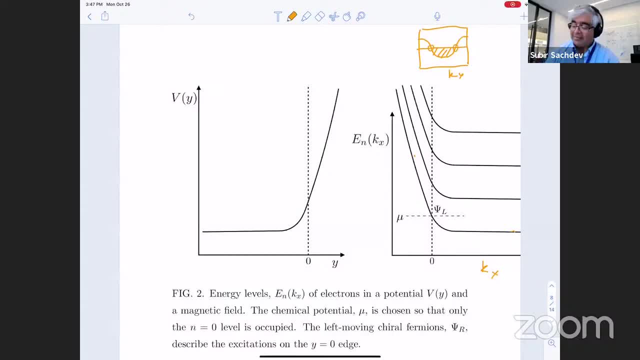 And then I said: this is where the Fermi surface or the Fermi point is, And then I linearized about that point. So here now these states are all occupied And I have a Fermi point here, much like this Fermi point here. 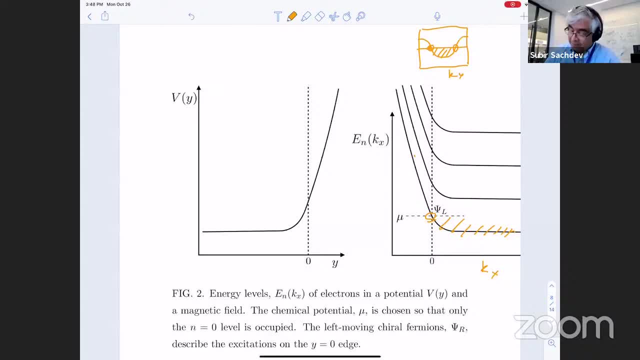 Okay, But This is the remarkable thing: Where is the other point as a function of kx? Well, it's nowhere to be seen, Because the other edge of the sample is presumably a few miles away. at y equals, you know, minus 10 million, or something along this direction. 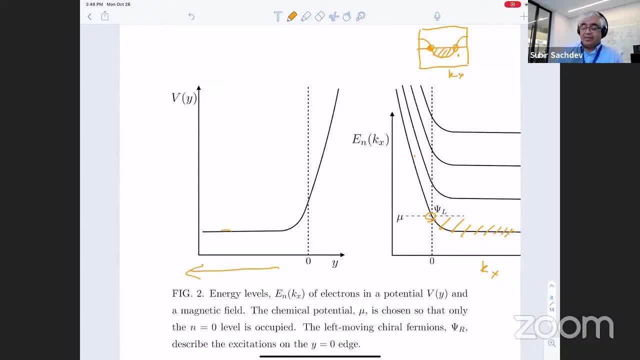 You know, that's where. And kx- that's a very different value of kx that I don't care about because it's so far away, It's microscopically distant from me. So therefore I have a remarkable situation: that on the edge of a sample I have a Fermi point or particles that move only along. 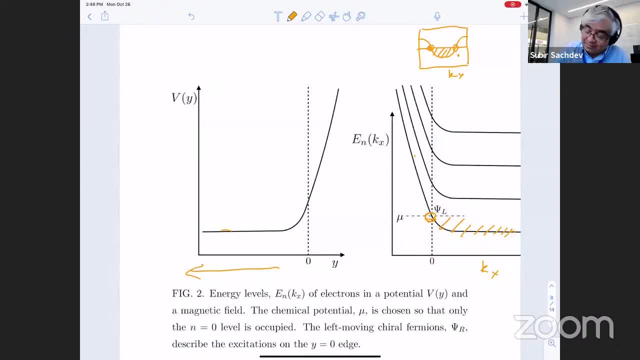 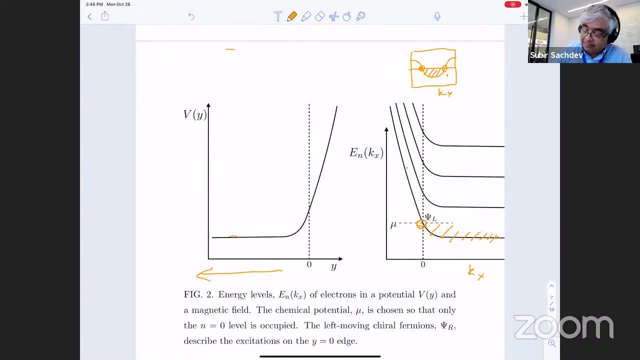 This is the left edge in the left direction. So here's my sample, If I try to draw a sample. Yeah. So This is x, This is Yeah. This is y, where the potential is. This is x. 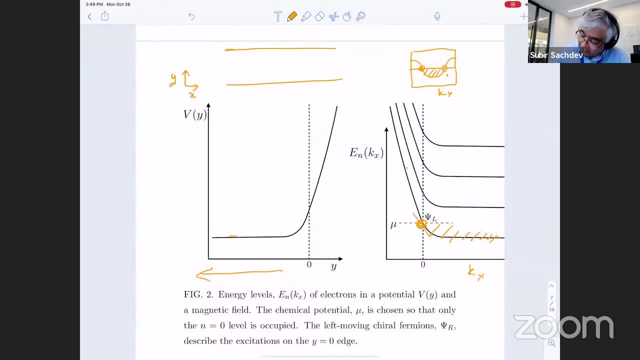 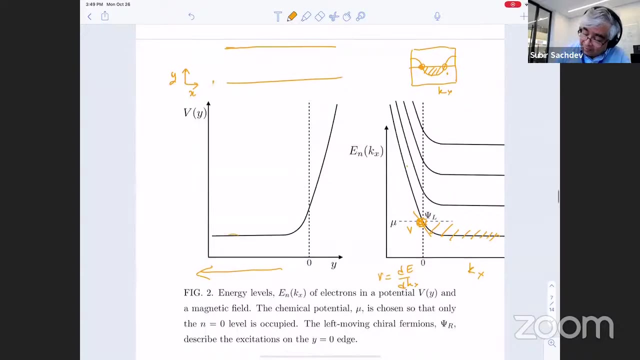 Then at this point I have some slope. That slope will determine some velocity. dE dk is always a velocity, So v is dE dk. So on this edge of the sample, at y equals 0. I have a particle that's. you know, energy increases as kx decreases. 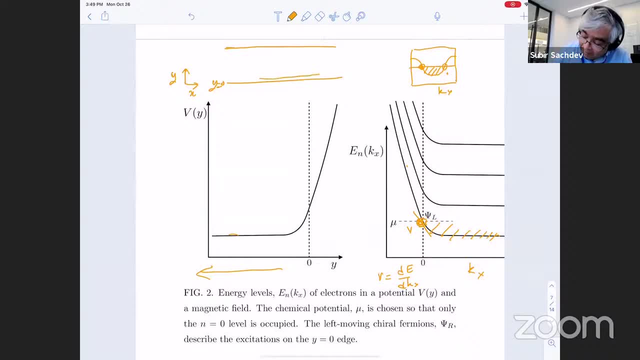 That moves to the left. So I have a particle moving in this direction, Okay, And its wave function is some sort of Gaussian, you know, of all of the magnetic length, or a few, or maybe a little bit bigger right near the edge. 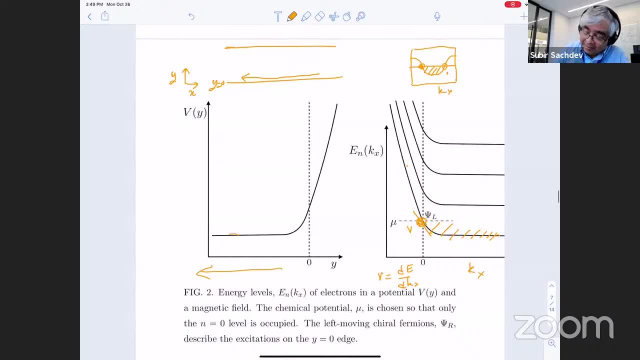 So as long as I don't care about the other edge of the sample, which is x, I don't care about the other edge of the sample, which is l? y away, Then on the other edge I'll get a right moving edge. 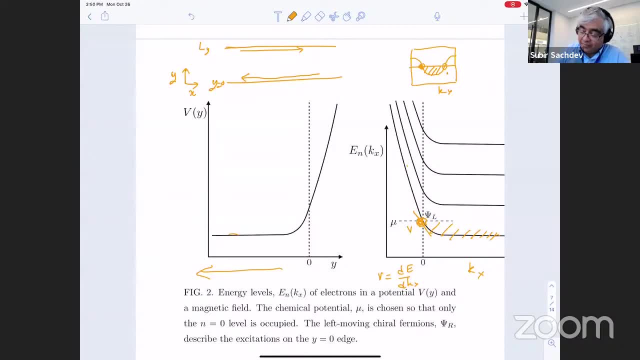 And on this edge I have left moving And in fact, if this was a closed sample, they're of course going in a circle And these excitations are essentially zero energy. They're right at the Fermi level. 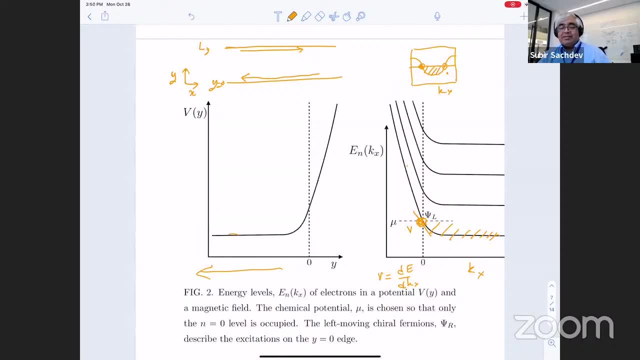 So what we find is they're gapless excitations And the edge of any quantum Hall sample. it doesn't have a gap. There are gapless excitations, But the gapless excitations are not two-dimensional, They're one-dimensional. 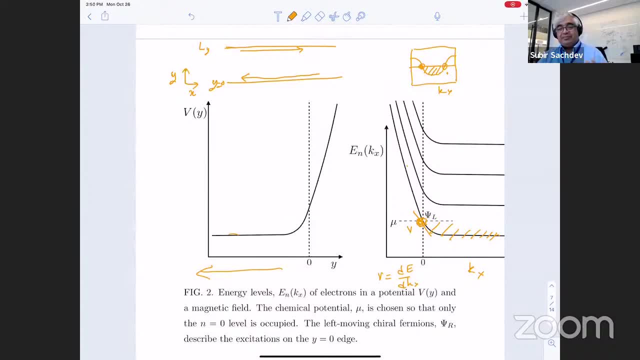 And, furthermore, they're chiral. On one edge, they only move to the left. On the other edge, they only move to the right. Okay, And so what you're seeing, as we'll discuss in some detail, something that can only happen on the edge of a sample. 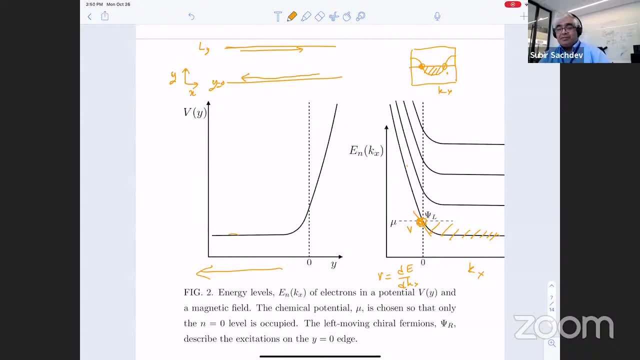 It can happen in the bulk Where you just have only left movers and not right movers. But at the edge of a sample in the principle magnetic field for a two-dimensional electron gas, there are states that are gapless And they move only in the left direction with some velocity v. 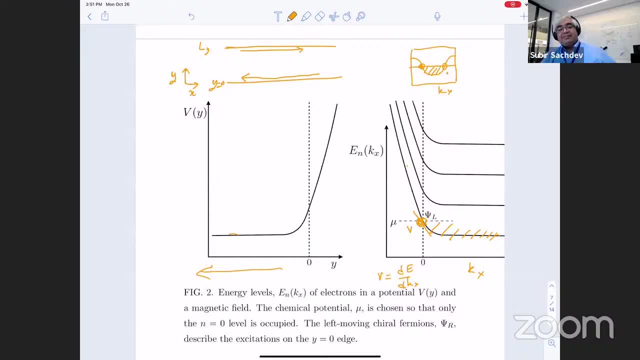 And on one edge and only on the right direction at the other edge. Now, of course, you could imagine that. you know there's some backscattering process, There's some impurity or something here, And because of the impurity, 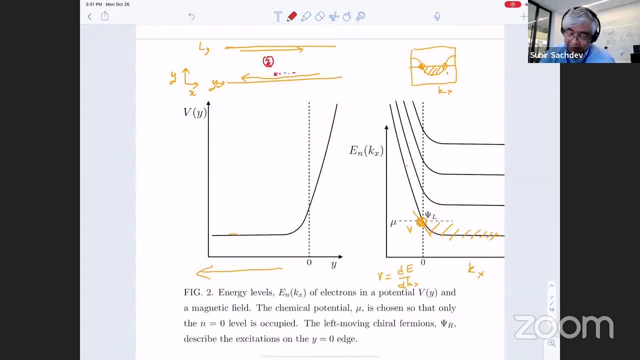 some scattering region here, an electron can come in on this direction and get scattered back And, as we'll see, it's only these processes that destroy the quantization of the Hall conductance. But in the absence of such processes, having things that 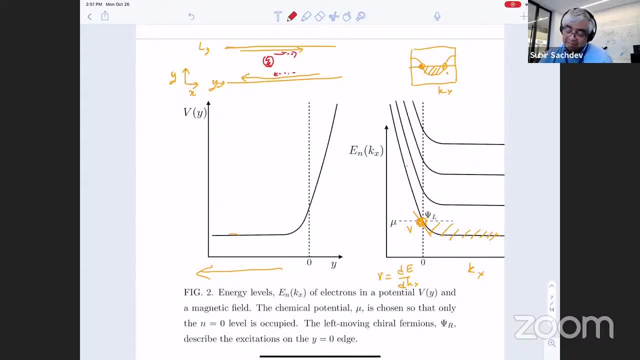 move along the edge means that if you put in some impurity over here or impurity over there, the particle as it's moving along will just can't turn around, because it's only left-moving states will just go around it. 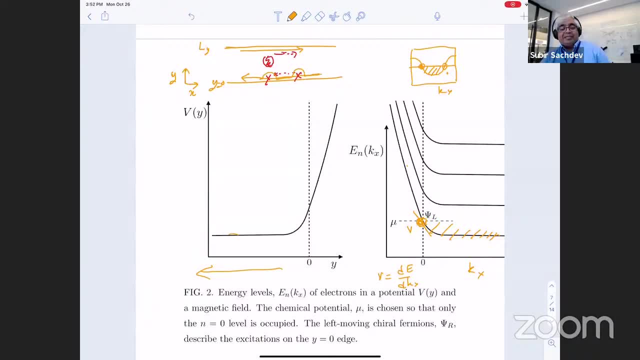 So there might be some deformation to the trajectory because of impurities, but it'll never turn around And this is ultimately the reason. the absence of backscattering on any one edge is the reason for the quantization of the Hall conductance. 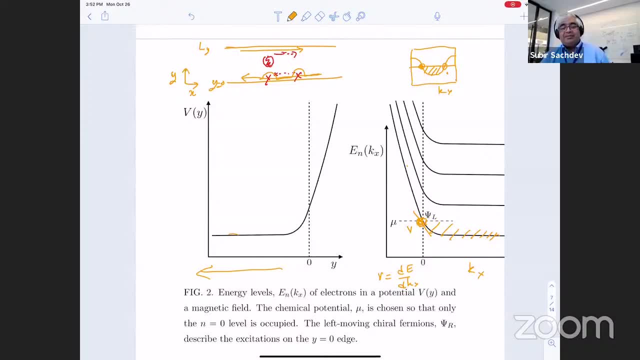 Even when you put in interactions, when you put in impurities and so on, it's totally robust because nothing ever turns around. Everything keeps going the way it was on the edge. The only way it can turn around is by going to the other edge. 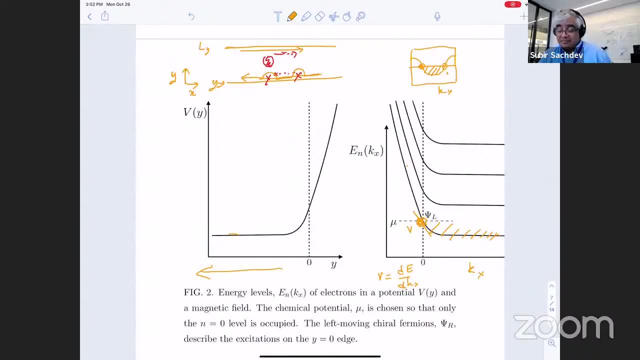 which could then be really far away on the scale of the magnetic length. Okay, I mean, there's a classical analog of this that's also worth showing you: The so-called skipping orbits. classically, So classically, if I have a magnetic field, 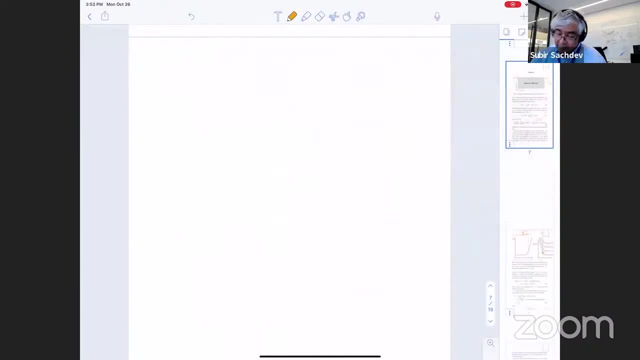 and a sample, then you know. here's my sample. now let me make it an actual sample. Classically we learned that the electrons all just go in circles in the presence of a magnetic field. So these electrons are really not going anywhere. 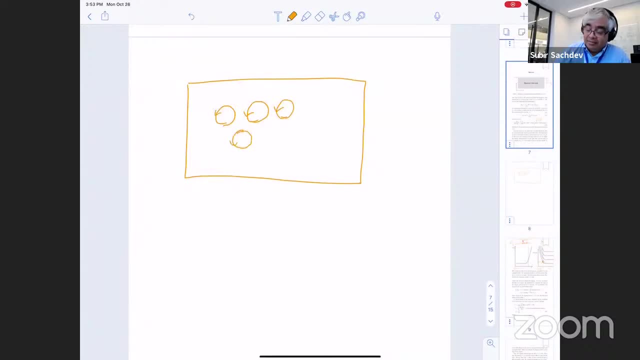 They're the analog of the Landau levels in the bulk of the sample. But as they're going, what would they do at the end? Well, at the edge of the sample there'll be an electron that's going to go this way. 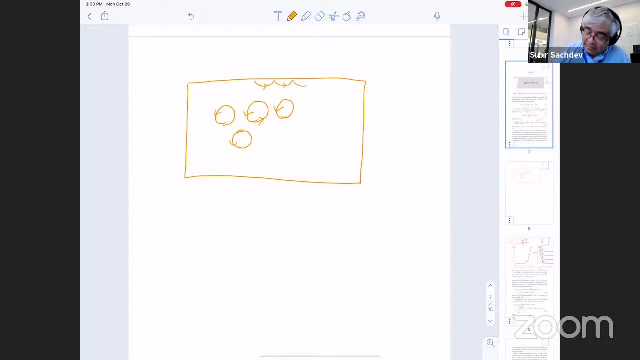 that'll be bounced back, So it's going to keep going this way. So there's only at the edge, with the help of a potential due to the boundary, can charges actually move. Everywhere else they just go in circles. I hope I drew that the right way. 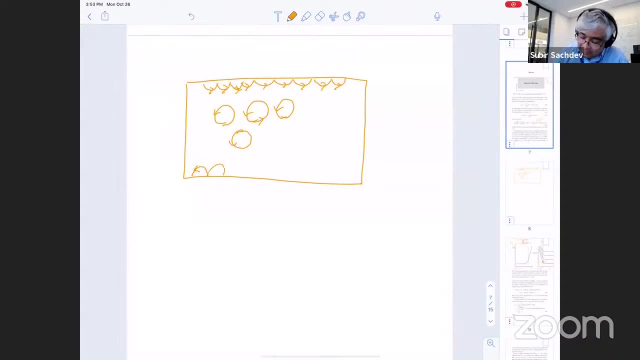 Yes, Okay, Here they'll be this way. So everything's just going in circles, but on the edges there'll be various skipping orbits that even classically you would conclude that all the action and the charge transfer the thing that's giving you the conductivity. 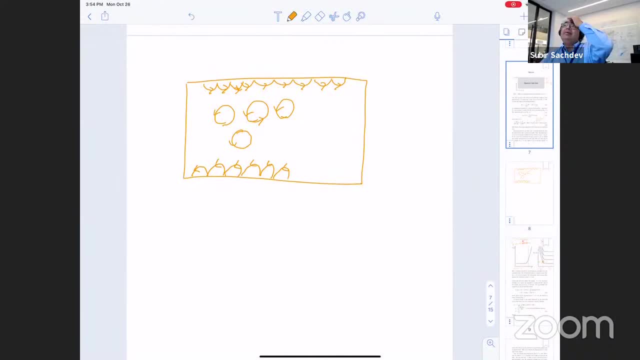 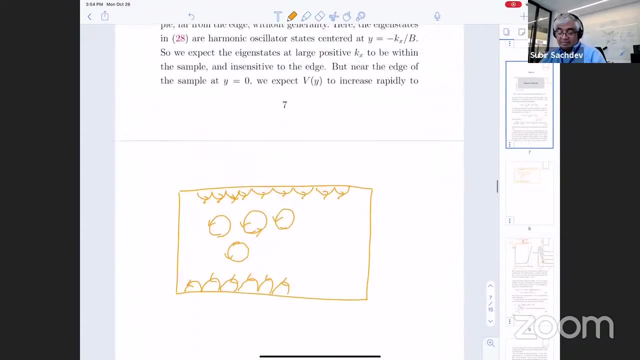 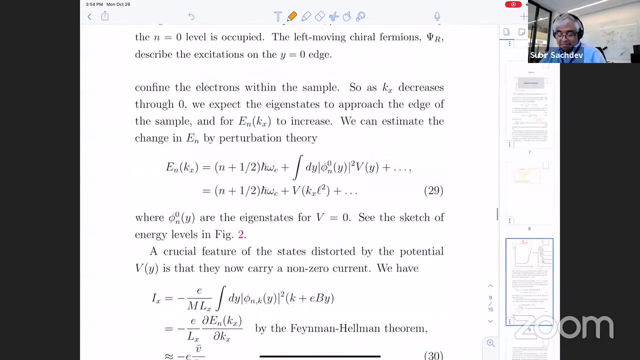 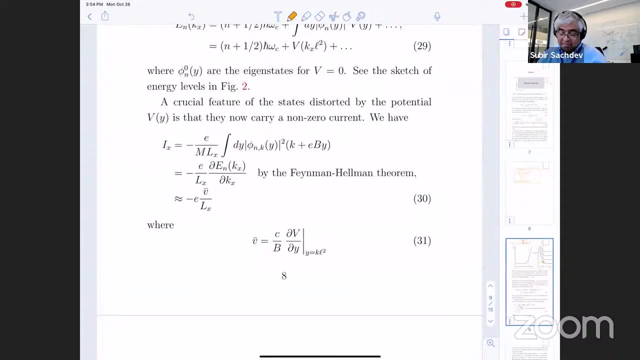 are the electrons right at the edge. Okay, So where are we? What time is it? Five minutes left. Yeah, I think I've done that. Okay, So now, now you okay, okay, Yeah, all right. So, yeah, let's discuss this. 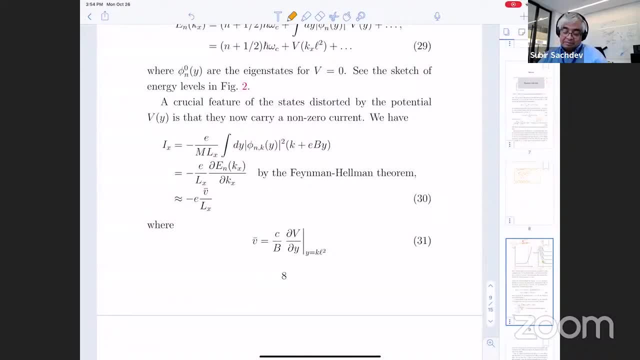 We can now go back to our previous computation of the current, which I told you each each orbital in the Landau gauge had zero current. In this case, it's the same expression as before for the current carried by any one of these orbitals. 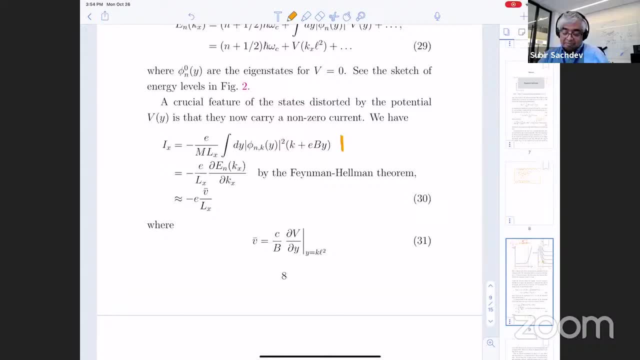 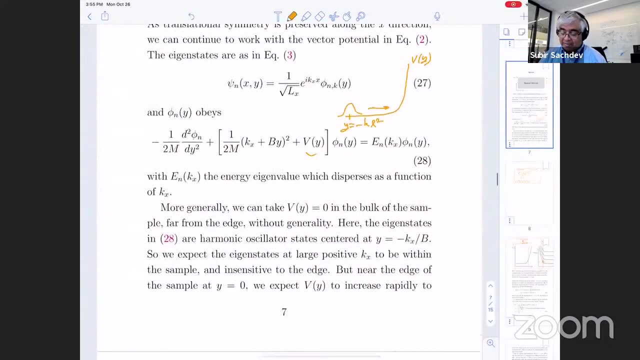 But, but it's. but this is not zero anymore, because I don't, because the equation for phi has this extra v of y in it. So there's no symmetry in v of y that allows me to tell me that that matrix, that integral, is zero. 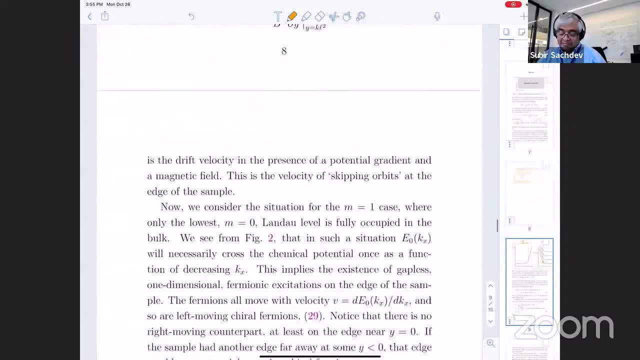 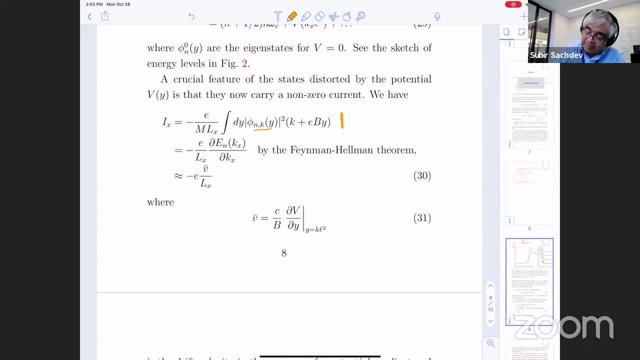 However, nevertheless, I can use the Feynman-Hellman theorem to show that this is the derivative of the eigenenergy with respect to kx. So the Feynman-Hellman theorem which you can try to prove is that, if you have, 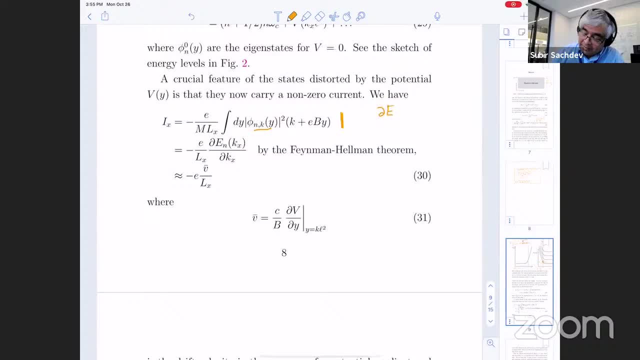 some parameter- lambda- on which your Hamiltonian depends, then the rate of change of the energy with respect to lambda is equal to the expectation value in the state that you're interested in of dh, d lambda over m. So if you wanted the derivative of the eigenvalue of any state, 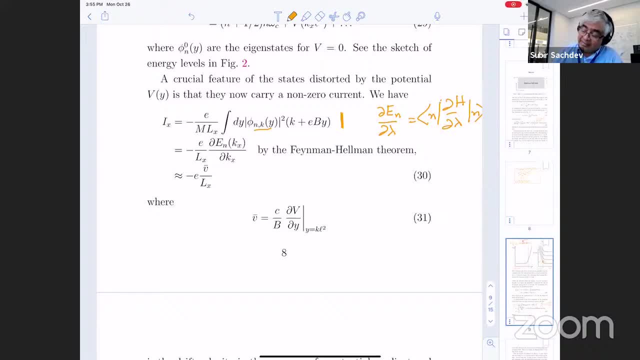 with respect to any parameter, it's the same as taking the derivative of the Hamiltonian with respect to that parameter and taking the expectation value in the eigenstate that you're interested in. So if you use that result, which is takes a few lines to prove, 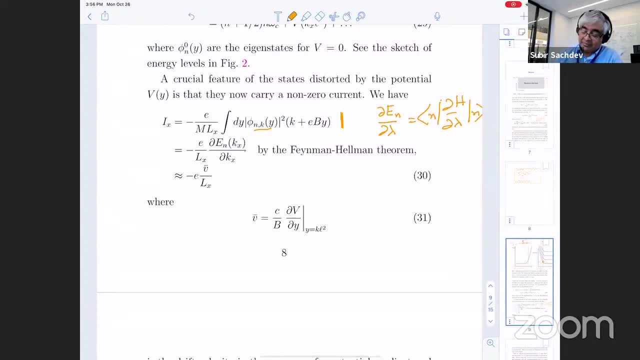 not difficult. you conclude that this is true, And this is another way of understanding why this was zero before, because en was independent of kx. But now the energy does depend on kx, right here, And so that derivative gives me the velocity. 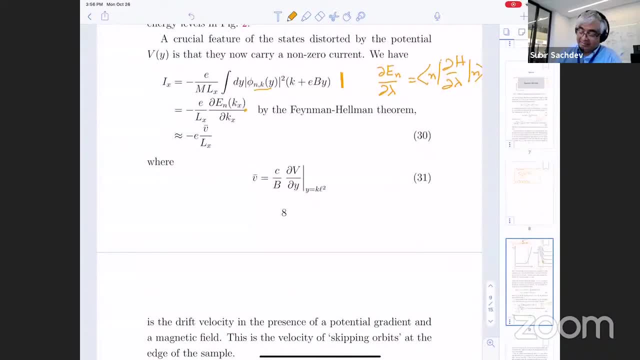 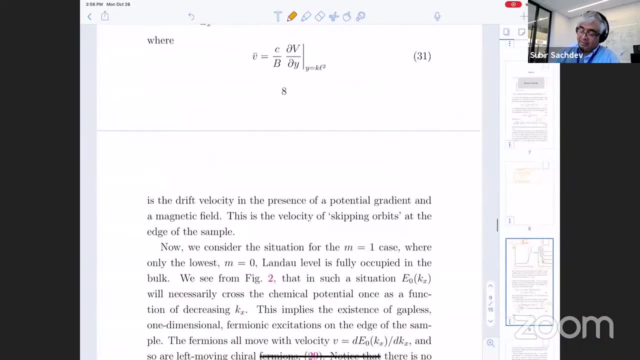 So in fact, that's what it is. All right, All the units are all worked out in the node, So there's a drift velocity in the presence of a potential gradient And this is the skipping orbits at the edge of the samples, like I just said. 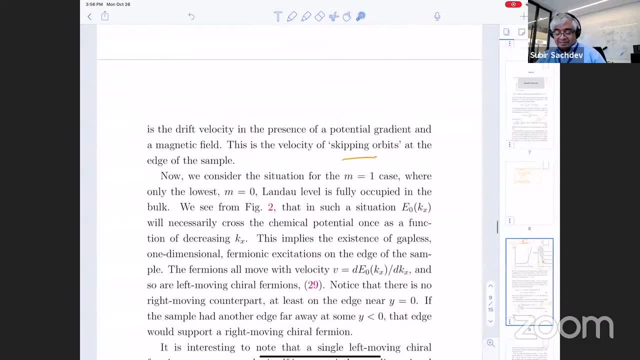 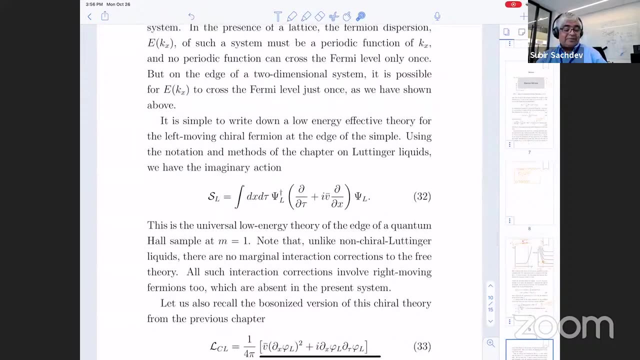 Okay, So they carry current at the edge, And you can see that from all the pictures I've drawn or by explicit calculation. Okay, So what is the low energy theory then of the edge? But now you see why I spent so much time. 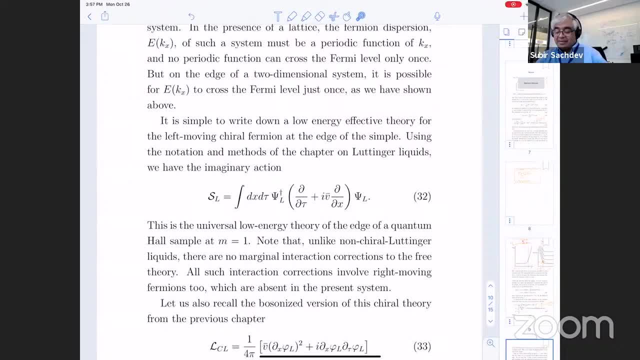 on 1D physics. Even in this 2D sample, 1D physics wears its head on the edge. So the theory for the edge you have like a one. you have a one dimension electron gas on the edge which has only left movers. 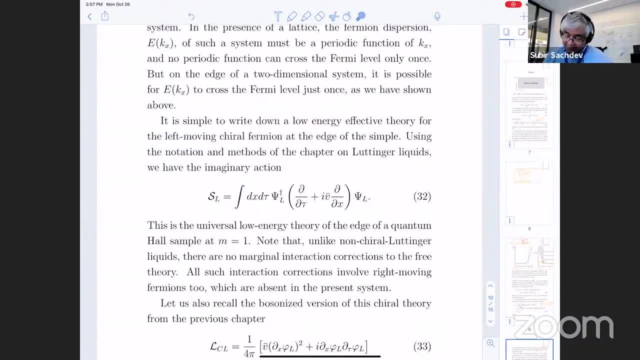 Okay, And so this is what's called a chiral Lattinger liquid. I mean, in fact, this is just chiral free fermions. We haven't yet met a non-trivial Lattinger liquid which is purely chiral. 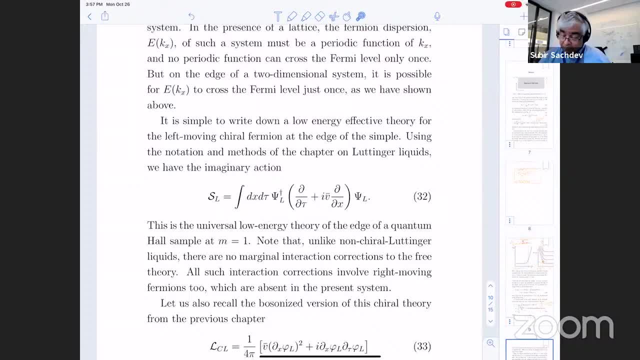 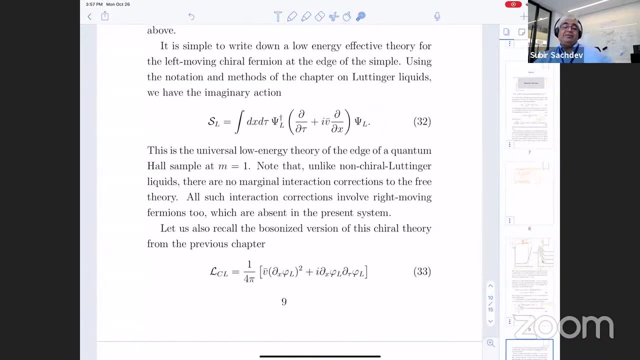 That turns out to be quite subtle to make. If you put in now interactions between this, you can bosonize the sample, this theory, as we just did in the previous chapter, And you get this Lagrangian which we saw also. 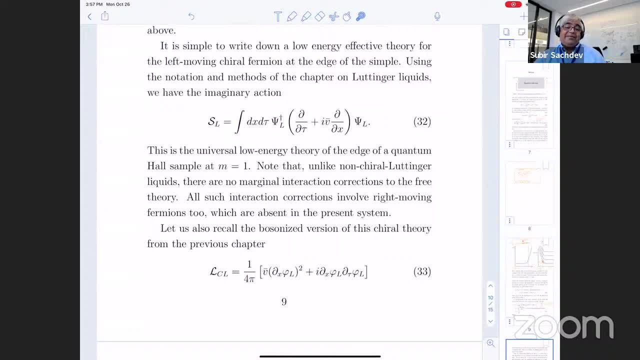 in the previous chapter. Now it only involves phi left moving, phi everywhere There's right moving- has disappeared. Now, as you go back to our previous chapter, you'd also see that all the interesting interaction effects that we consider the things that change k. 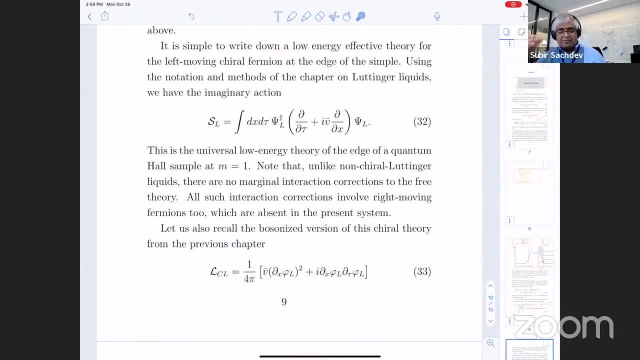 from one to some other value, the Sengordon terms. everything all had to do with both left and right movers. So all the stuff that we considered in the last chapter has disappeared Now, if you go back to our previous chapter, 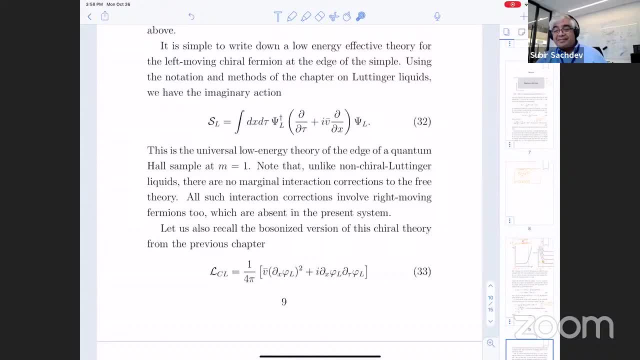 you can see that in the last chapter disappears. Basically, if you have chiral fermions like this, interactions make essentially no difference to their low energy properties. This is pretty much the final theory, apart from you know some corrections you might have to put. 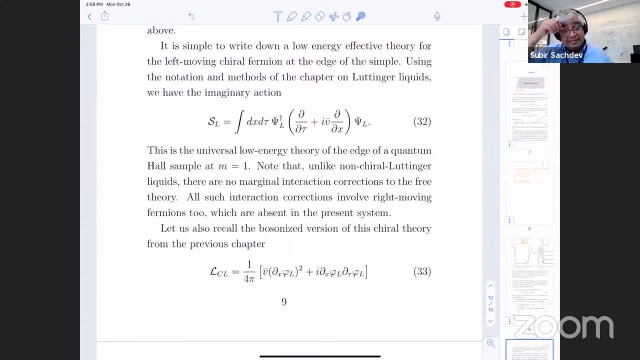 into the velocity of, to the, to the value of v bar. So the defining property really of any sample sowing integer quantum Hall effect is that it's called a chiral Luttinger liquid, The simplest free of free left-moving fermions. 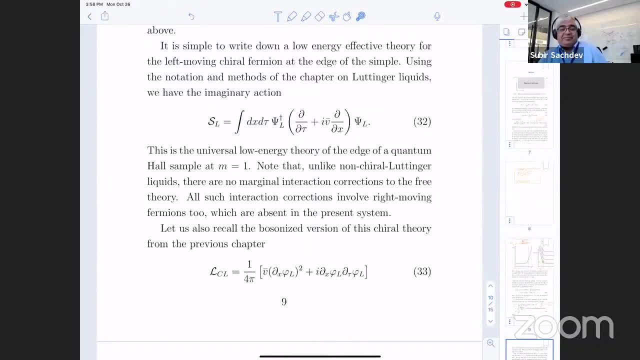 Calling it a Luttinger liquid is a bit too much, because this is just free fermions right now, But we'll eventually see a theory when we go to the fractional case where it's not free fermions. And so that's the defining property. 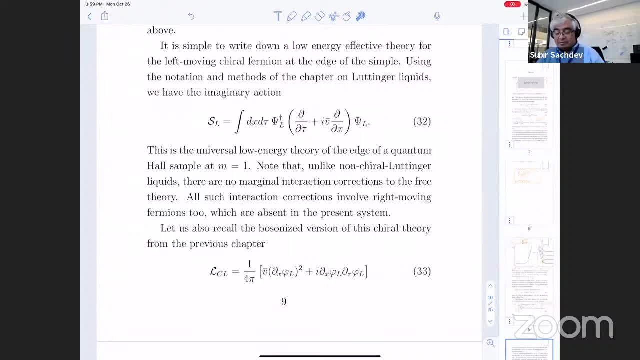 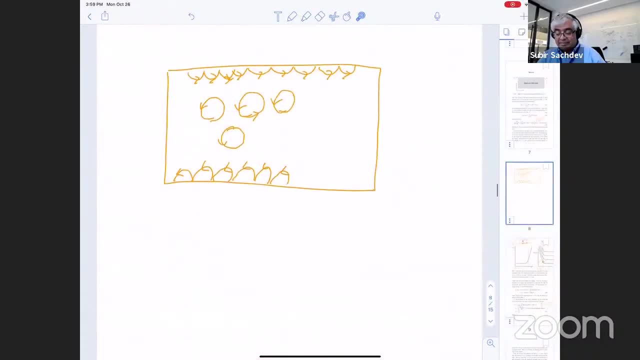 of any integer quantum Hall system And there's nothing you know at some level, nothing remarkable or surprising, It's just. this simple picture gives you an idea of what's going on. But then the edge orbits here of course, has to be treated. 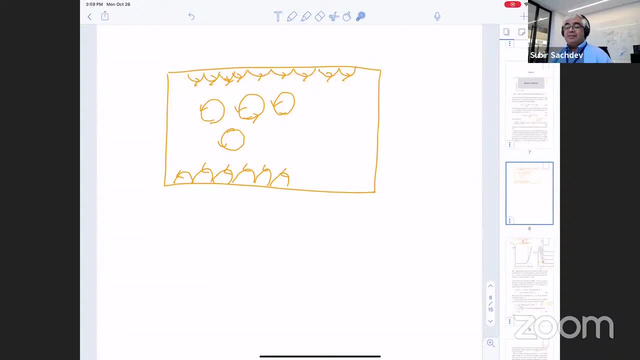 fully quantum mechanically, which we will. And you know, all kinds of beautiful experiments have measured very subtle quantum mechanical properties of this 1D, 1D electron gas on the edge of the sample, which only moves in one direction on each edge. 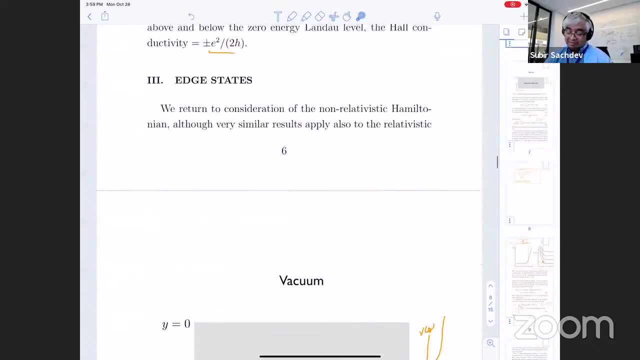 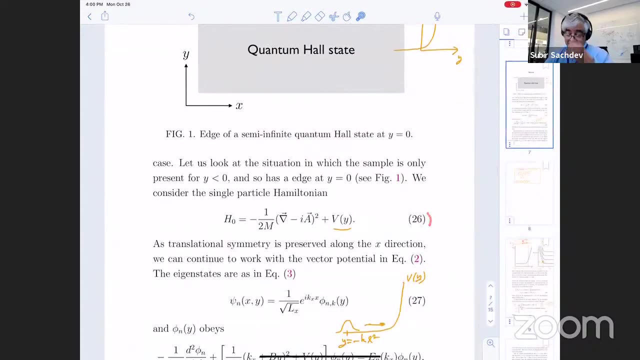 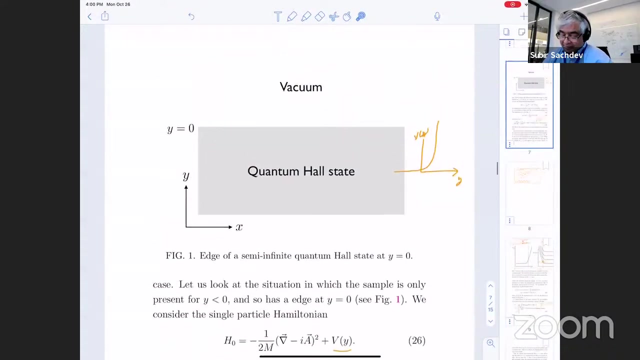 Maybe I should also note that this problem here and this description of the edge states here was worked out first worked out in a famous paper by Bert Halperin when I was an undergraduate. I think This was long before anybody had ever talked about. 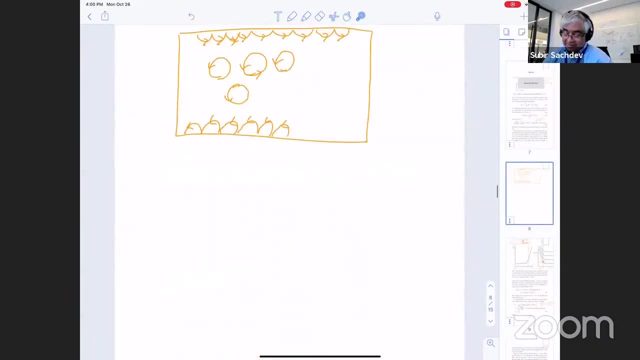 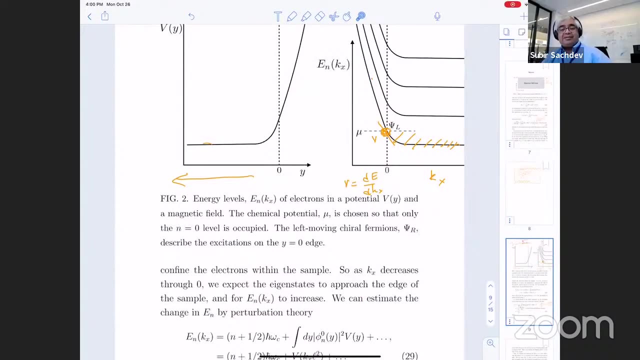 edge states and bulk edge correspondence and in terms of any such thing- And this, you know, is the key to many developments- that we're going to continue talking about the next few lectures. All right, I think I'm going to stop there and we'll continue. 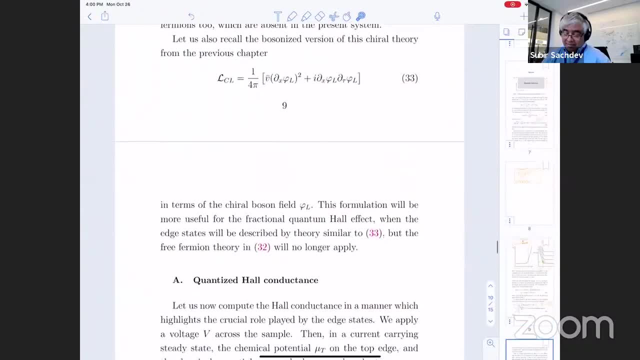 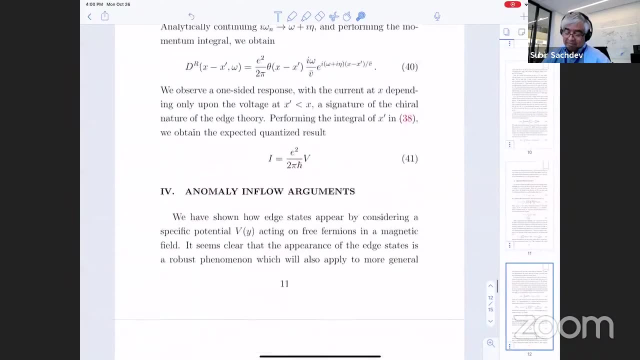 our discussion of the integer quantum Hall effect tomorrow. I have been updating the syllabus on the website depending on how far we're going, So, as you'll see, we'll compute, you know, the conductance a different way, not without using. 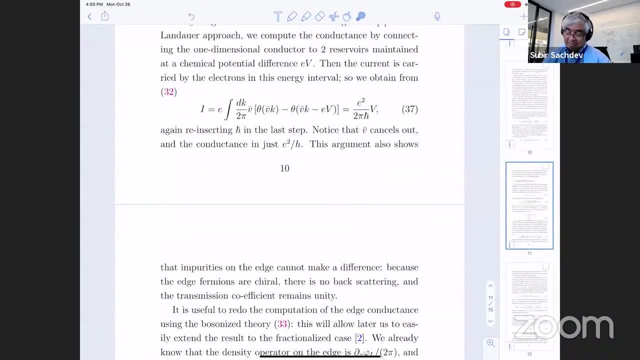 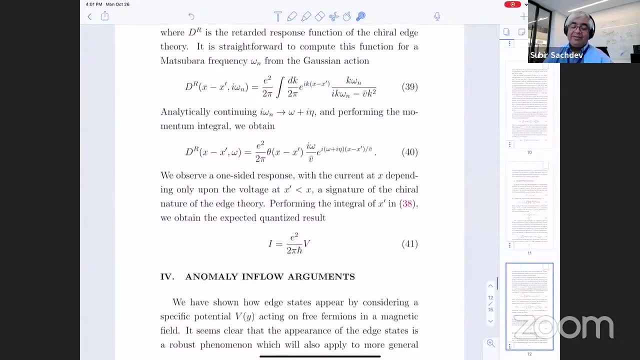 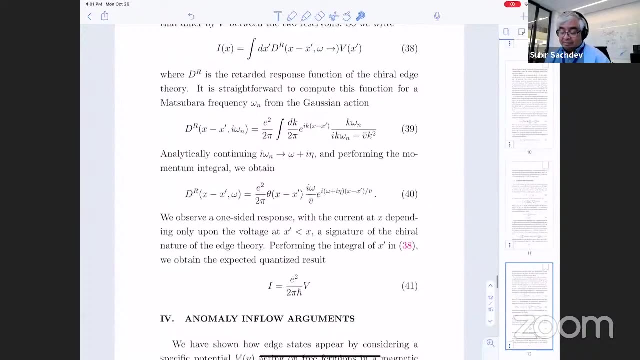 the Cooper formula, but using more, you know, just explicit evaluation, using the Landau picture, And that will also make it clear why it's quantized and also show us how you know and the reason for doing it this more revealing way. 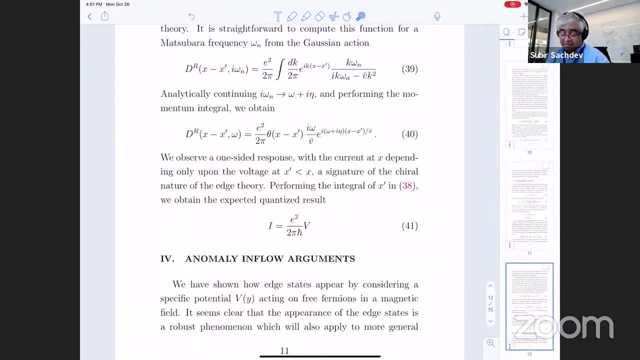 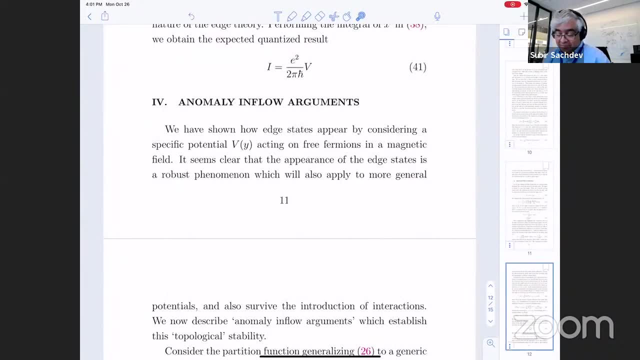 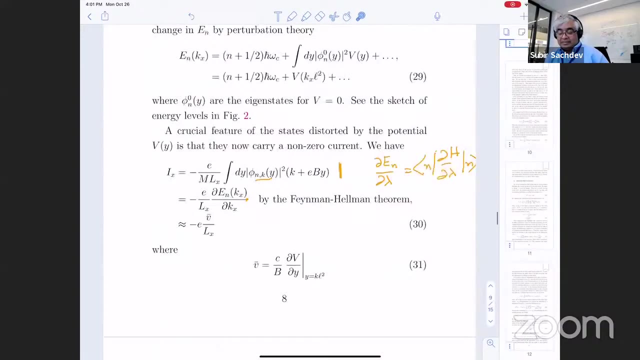 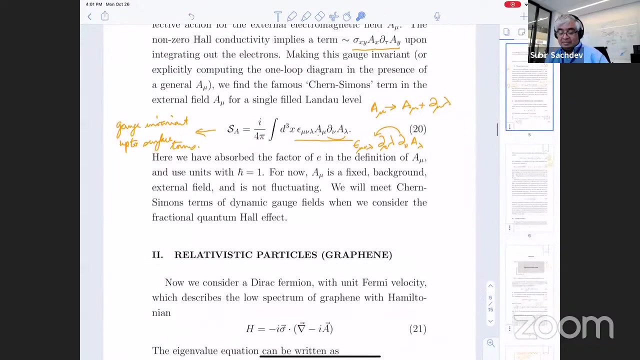 is that these ways are the ones that generalize to the interacting fractional cases. And finally, I'll make a connection between the fact that the Chern-Simons term I wrote down here, in the presence of this external electromagnetic field wasn't fully gauge invariant because of the 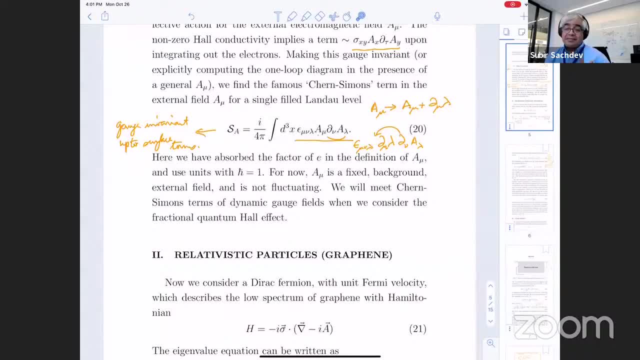 extra surface term and the existence of the edge state. So those are very closely tied to each other by what's called an anomaly inflow argument, And it's really that argument that tells us most cleanly that the edge states have to be there. They're just required. 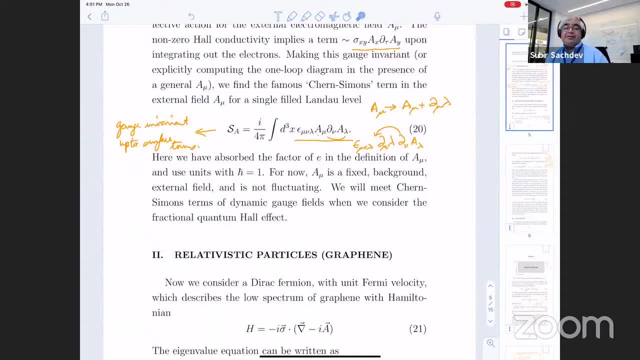 to be there. You can't remove them any time. you have a Hall conductance like this, you know, in a gap sample in the bulk. All right, I have a question. Yeah, please go on. So the it makes sense why with this? 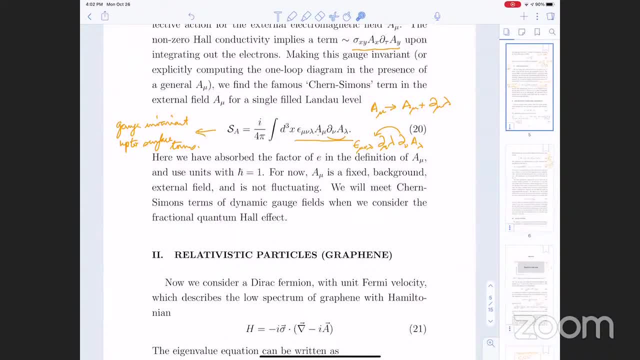 like plane wave. in the X direction basis we have these states moving along the top and bottom edge. But if we had side edges, wouldn't those plane waves be bouncing off the side edges rather than going along them? Like you would have to use Y plane waves. 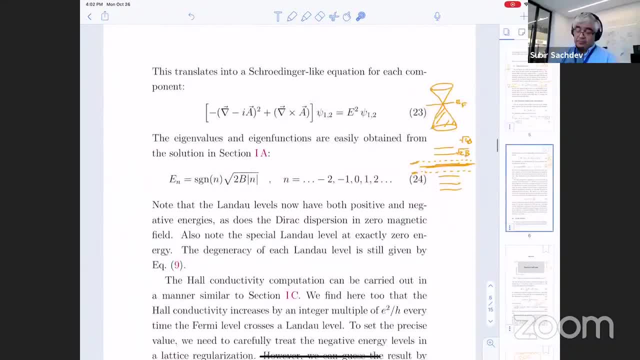 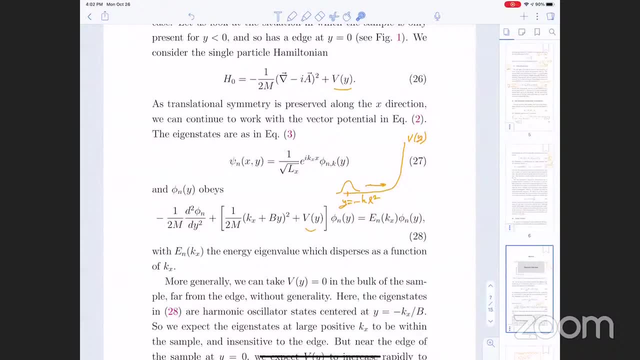 along the up and down edges would or like. is that what's the general idea to include, I guess, like edges on the top and bottom and on the sides. Well, of course that becomes a very difficult problem. So the one freedom that I've been 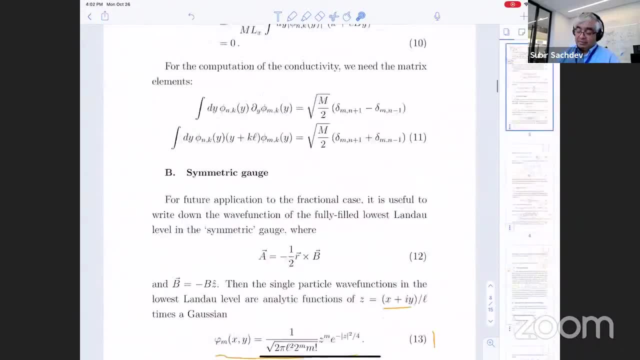 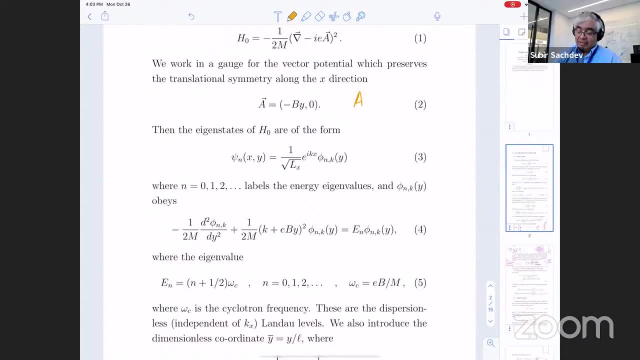 exploiting is. is is the gate choice, you know. so I said I'm going to choose. you know, AX equals BY, where I could equally well have chosen a valid choice. They gave they both the same magnetic field in both cases. 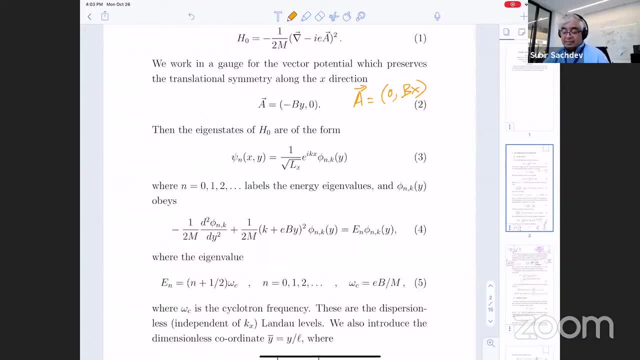 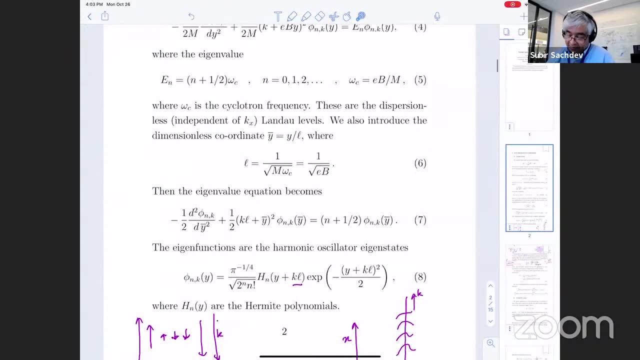 So what does that mean? Well, that means that if you work in this gauge, if you work in the first gauge, you'll find some eigen functions which are here, these eigen functions, here, and they turn out to be, you know. 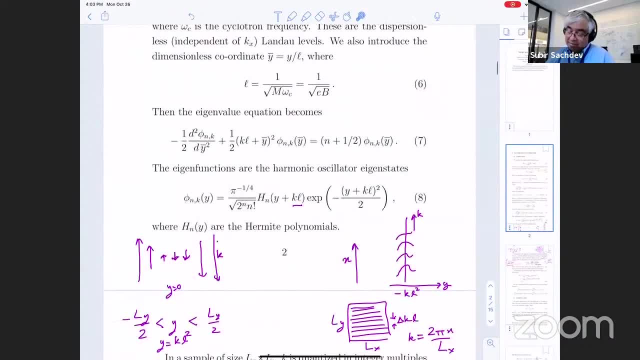 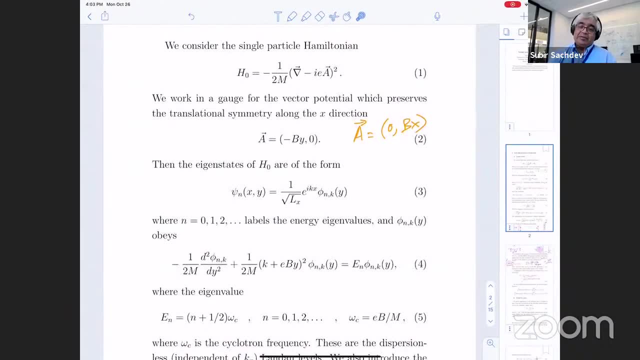 quite degenerate. But you can find some set of eigen functions and eigen energies. Well, if you work in a different gauge, you're guaranteed by the gauge invariance of the Schrodinger equation: you get the same eigen functions, eigen values. 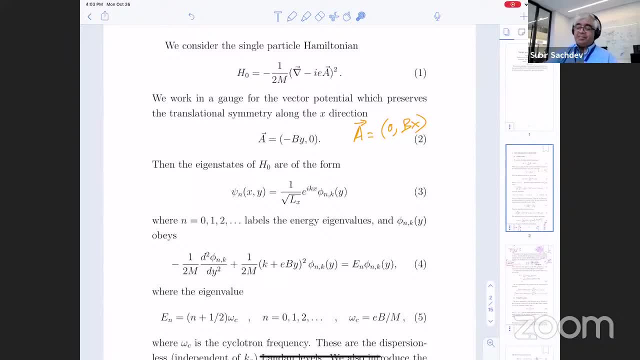 And the eigen functions should be gauge transforms of each other. If you have a non-degenerate level, that's straightforward: You just do a gauge transformation. If you have a fully degenerate level, as we had here, without a boundary, then all you're guaranteed. 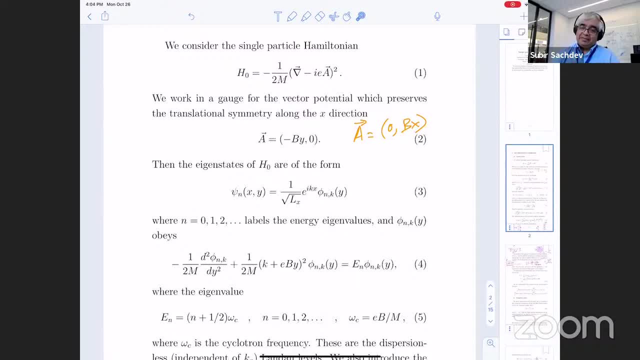 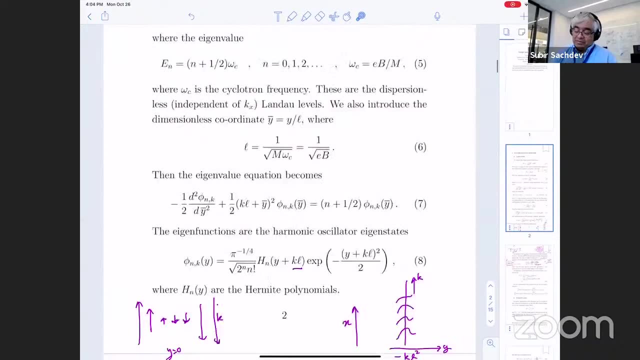 is that wave functions in one gauge are linear combinations of wave functions in the other gauge after the gauge in the other gauge. All right, So. so it's just a choice. Okay, So what you would do here, you know. if I don't worry. 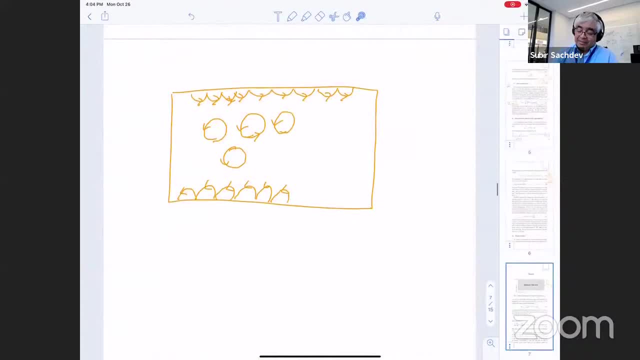 about the edge, the corners. the corners are, of course, the most difficult. So if I'm working over here, I will choose the gauge I've chosen where the vector potential doesn't depend on x, because physics doesn't depend on x to begin with. 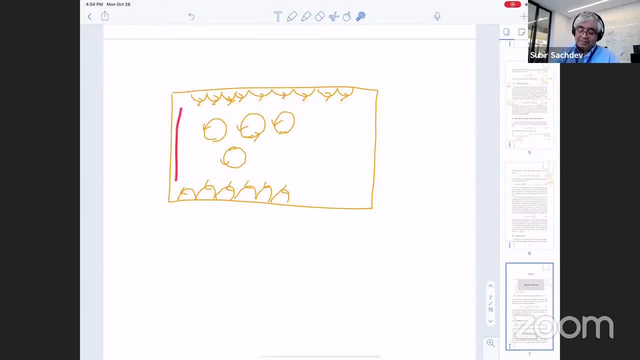 in this direction. So it may make the vector potential depend on y, But if I'm working over here the vector potential, that doesn't depend on y, because everything seems to depend on x, and that'll just make my life simpler Now, Okay. 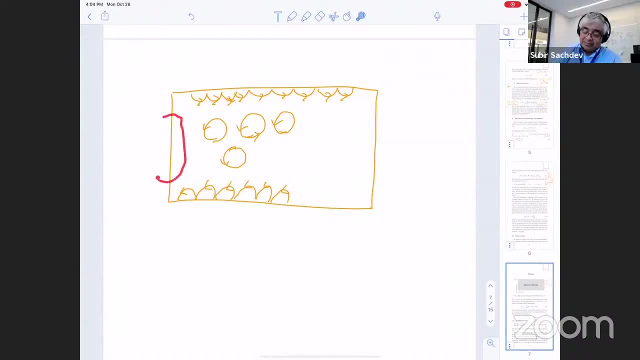 Okay, I mean so you can kind of, at least in patches, by choosing different gauges, solve the problem here and solve the problem here, And now you have to connect them together by, because that's complicated, You'd have to do that on a computer. 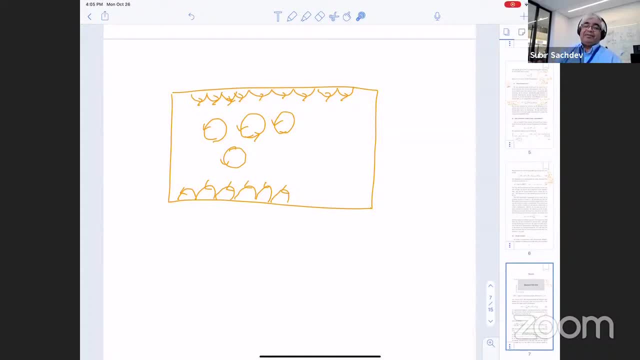 or something So. so in each region of the samples different gauges and there's no obvious gauge that works fully on, you know, sample with full edges On a torus, you know, there there are other gauge choices that people 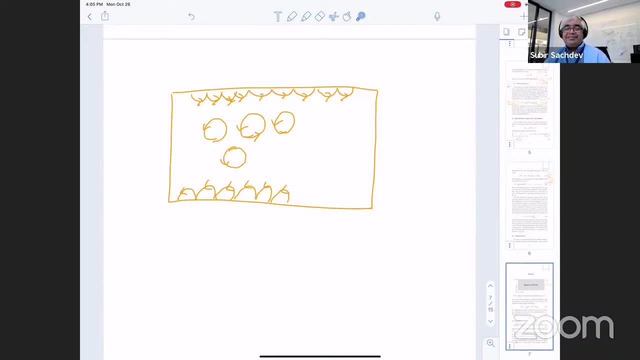 have developed, Yeah, but it becomes a messy problem in general, But at least in every region you can, you know you're free to choose the gauge that's convenient for you. That's all really we're doing here, I see. 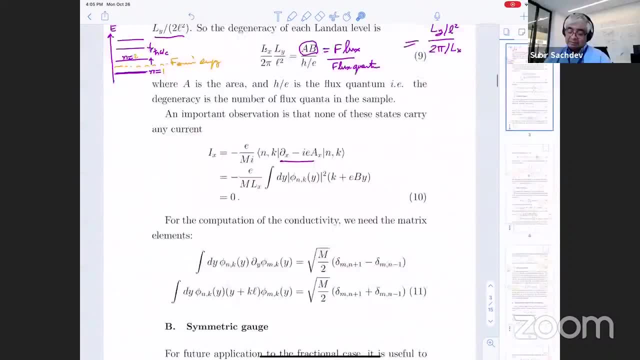 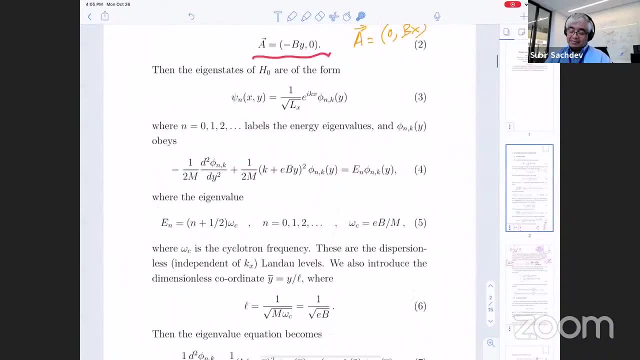 That's why it was very important when I- you know, when I made this choice in the equation one or equation two. it's very important. It's precisely for that reason that the boundary was in the right and ran in the X direction. 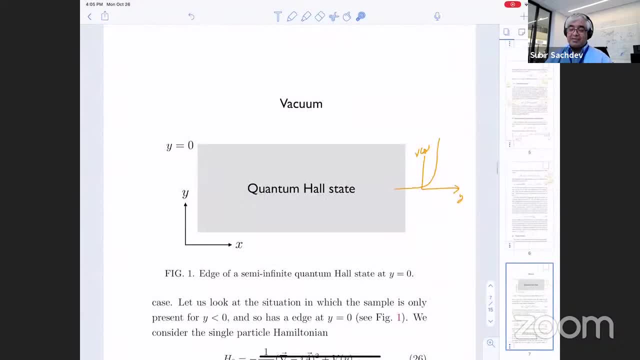 So if I took- you know that I took this picture- if I wrote it in this picture by 90 degrees, I would have chosen the other gauge. I, I guess my follow-up question was going to be: what do we know? 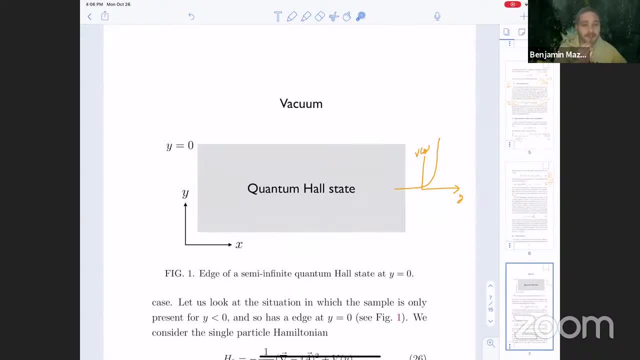 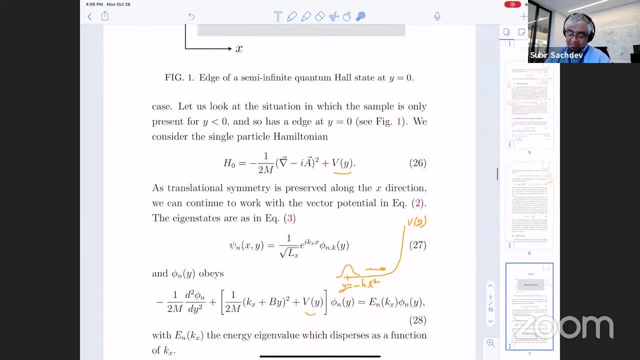 what happens in the corners, or is that just like some some mess, that Well, I think the semi-classical picture is not too bad, You know? I mean it just tells you that there'll be some orbital here, I mean. 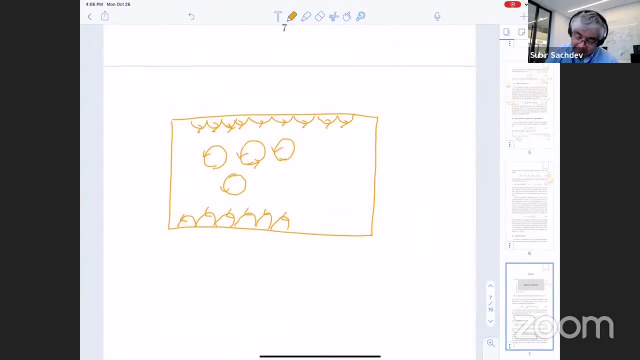 you can imagine, you can just try to draw it some, some orbital like that. You know, it's just, it's going this way, right, Yeah, so it'll go that way, Okay, well, it won't be exactly circular. 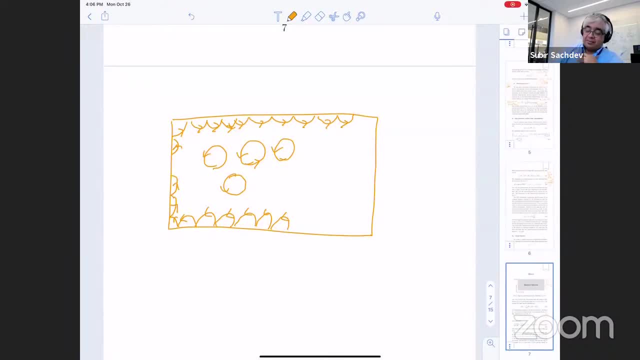 but there'll be some wave function here which is moving that. So. so the one thing I should say, that what the things that I'm drawing here is a physical object, It's the current, The phase of the wave function, you know. 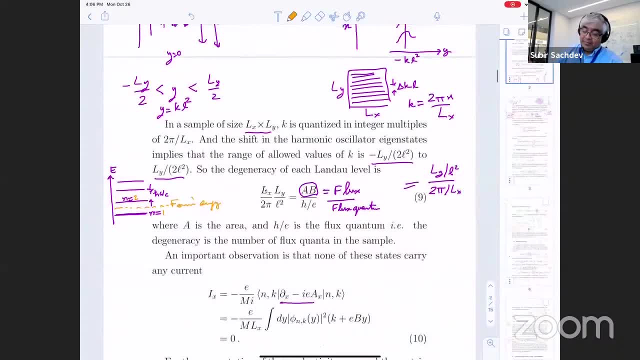 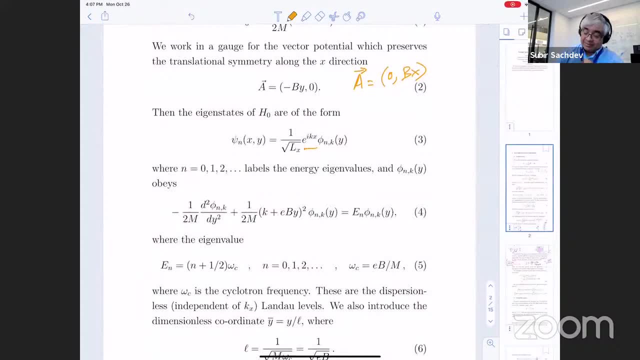 and that's one important thing to keep in mind. You know, if I, if I, if I, if you just look at this wave function, you would say it's moving the X direction. It's got a momentum. H bar K.